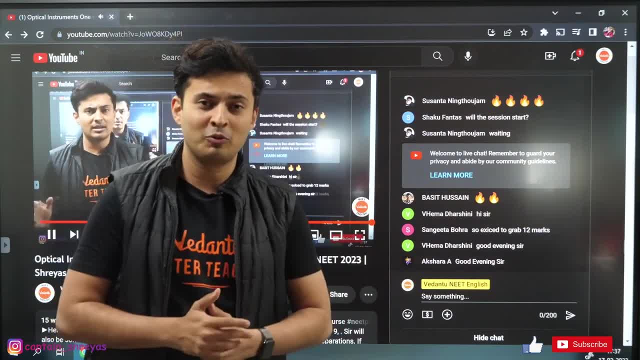 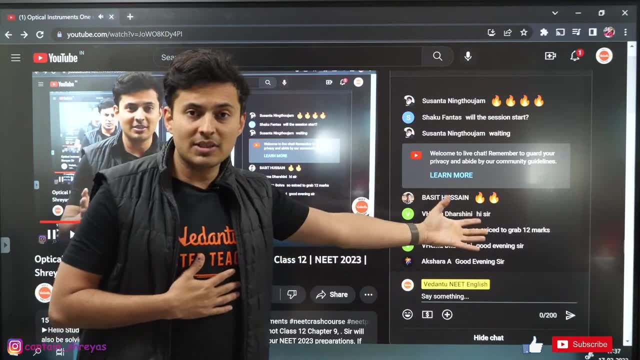 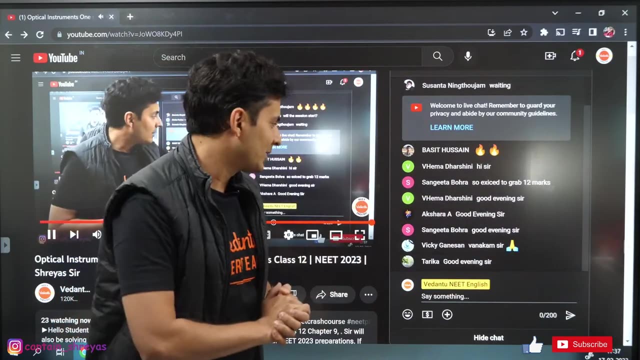 watch that one-shot marathon, which is more important- More than three hours, almost close to four hours. so watch that, okay, in case you have missed it, and if you have watched it before, then welcome to this session and make the best use of this. this will complete your ray optics chapter for boards, as well as NEET perspective Vanakam, good evening. 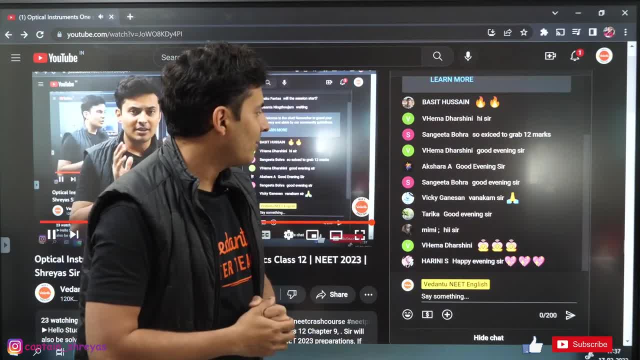 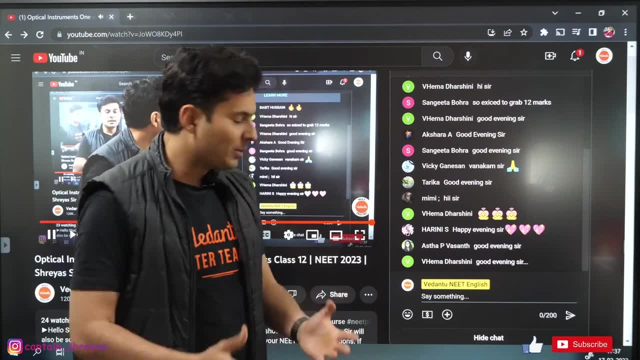 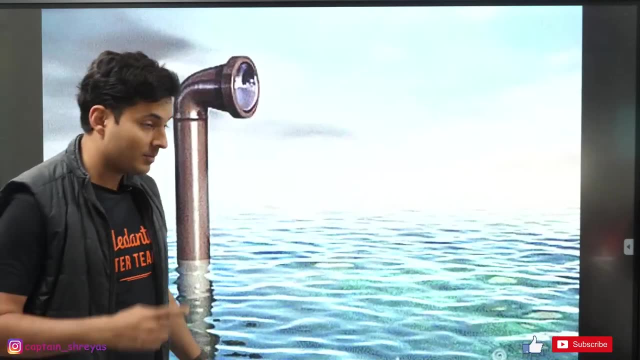 nice to see all of you, and so many of you are excited to grab the 12 marks, glad to know that. hello astha, hello harney. hema, mimi, tarika, vicky, sangeeta akshara, welcome, welcome, welcome. so let's first of all smashing the like button. okay, in case you haven't done that yet, please do that, it helps. 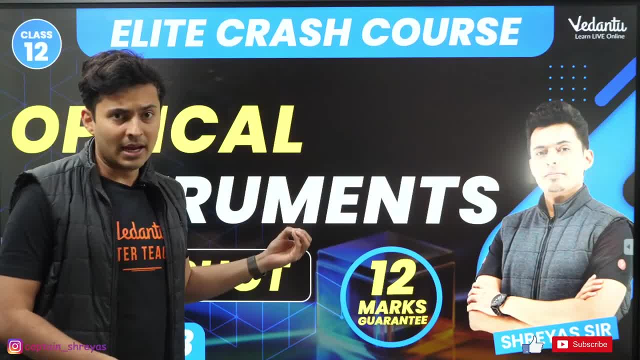 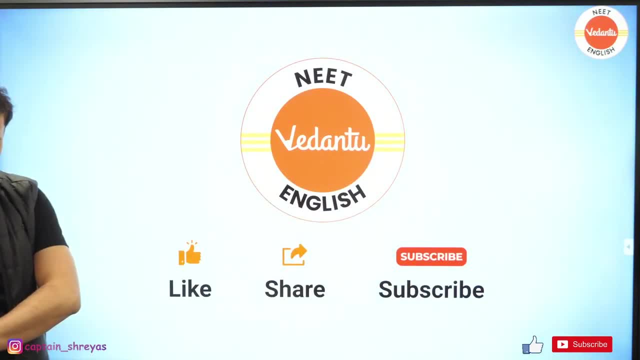 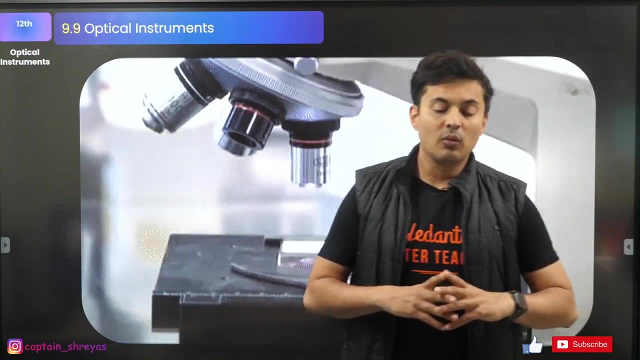 a lot in growing the channel and also hit the subscribe button. and those of you who do not know me, my name is trias. i am the physics master teacher, so let's begin the class, okay now? the first thing when we talk about optical instruments you should realize is that what? 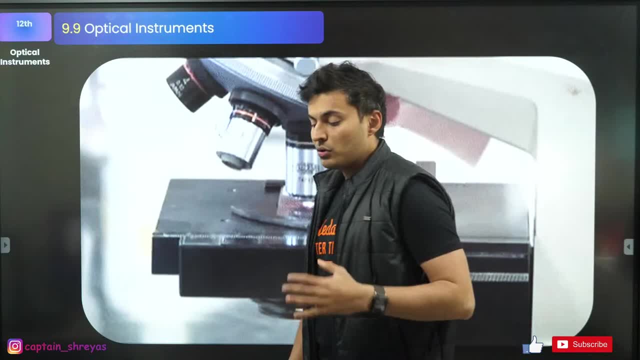 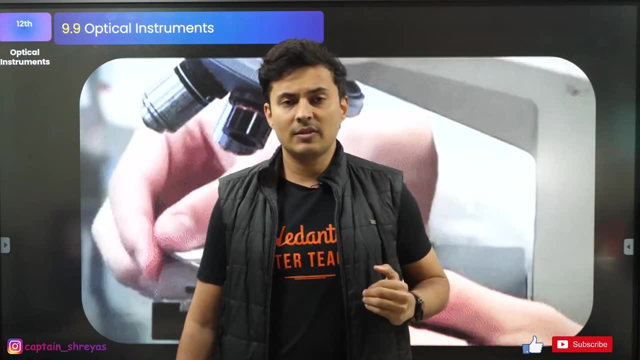 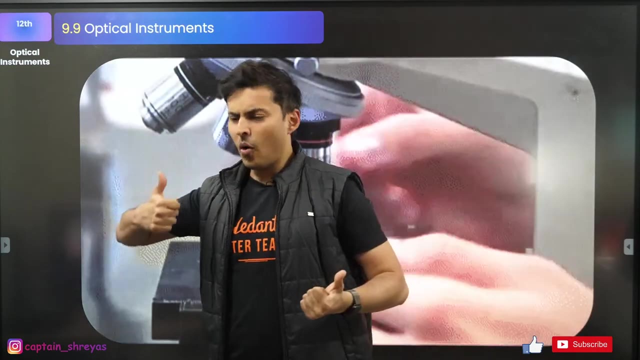 is the basic purpose of these instruments, and when do you use what see? when you see some object, okay, located at certain distance, then it might be seen clearly. it might not be seen clearly. if it is seen clearly, okay, everything good. if it is not seen clearly, you. 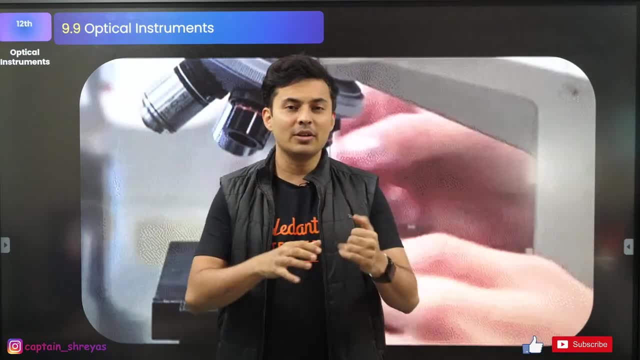 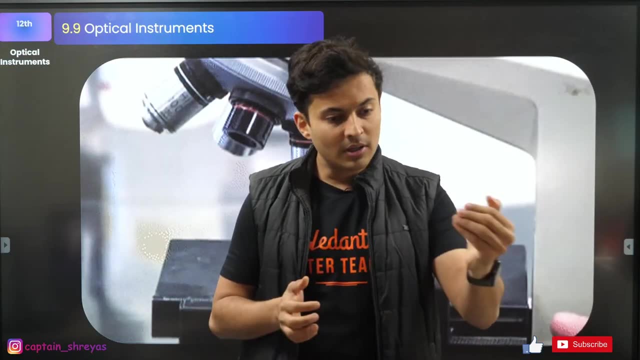 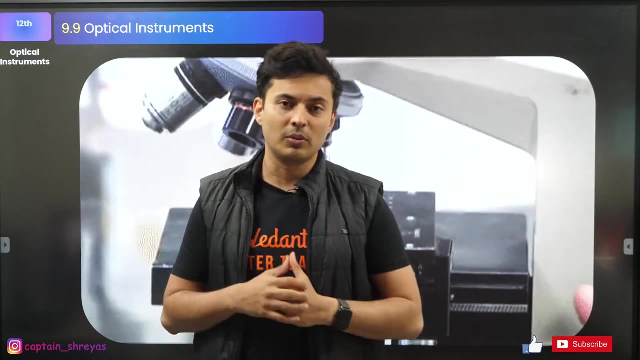 need the help or you need the aid of some instrument now. if the object is very far, then you will use a device called telescope, but if the object is very close, which needs to be seen, you will use simple or compound microscope. so if you want to analyze bacteria, everything, then you. 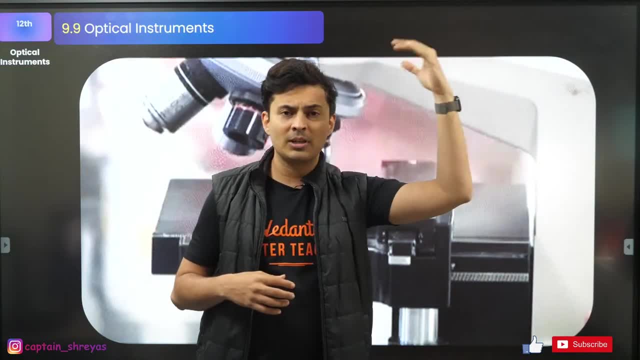 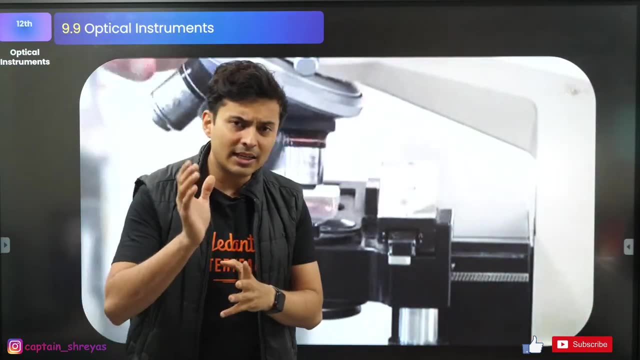 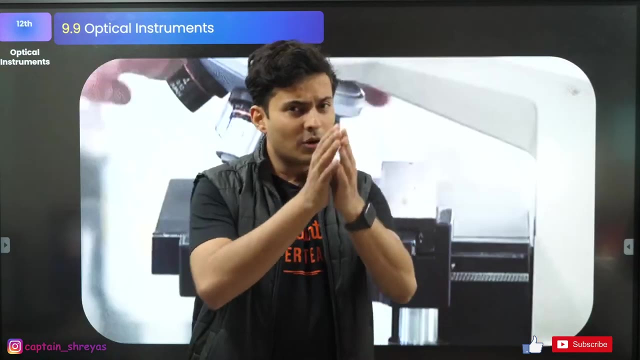 will use microscope. if you want to see the stars or the moon or the planets, you will use the telescope. now that you understand what is it used for, what exactly does each of these device do? okay, so understand that. see, when you see an object, let's say I am looking at Pandu. let's just imagine: 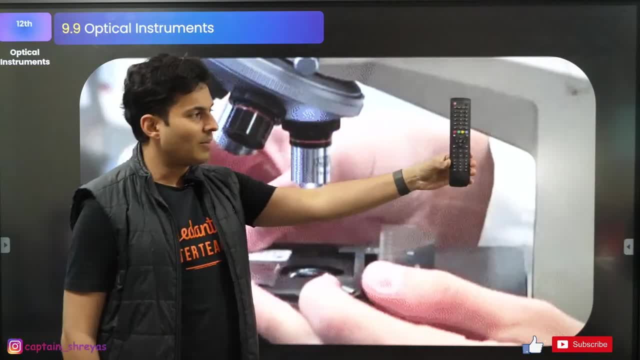 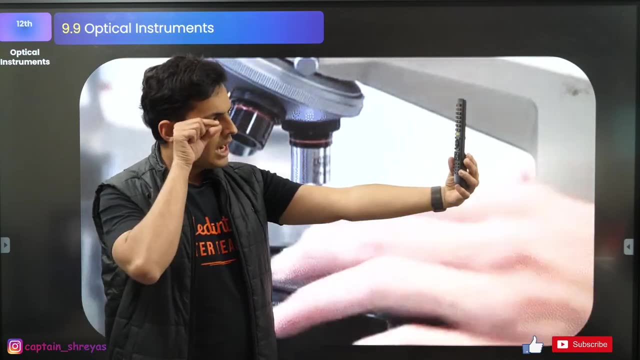 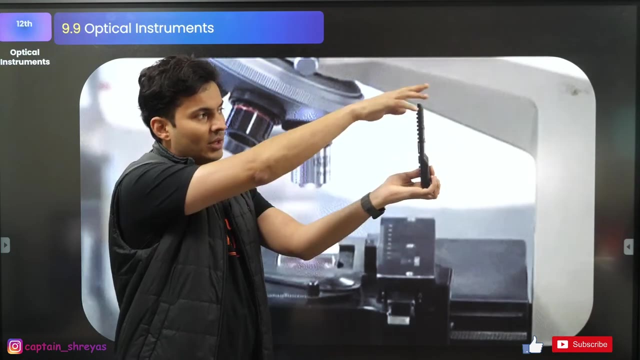 let's just imagine this remote sensor. okay, this is for the remote sensor. let's just imagine this remote of mine is Pandu standing somewhere. This remote of mine is Pandu standing somewhere. When I see Pandu, I will see that Pandu's height or the entire length of Pandu subtends certain angle. 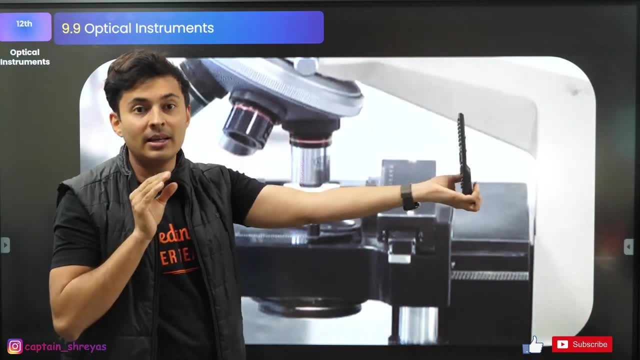 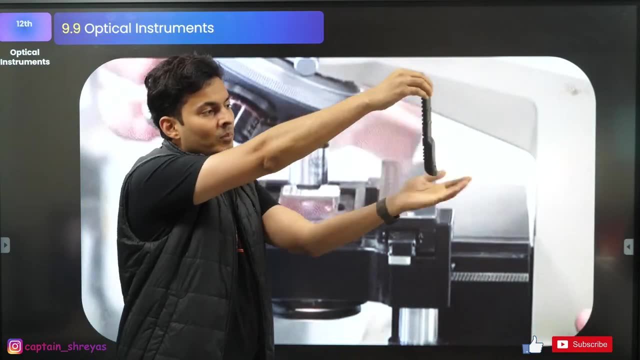 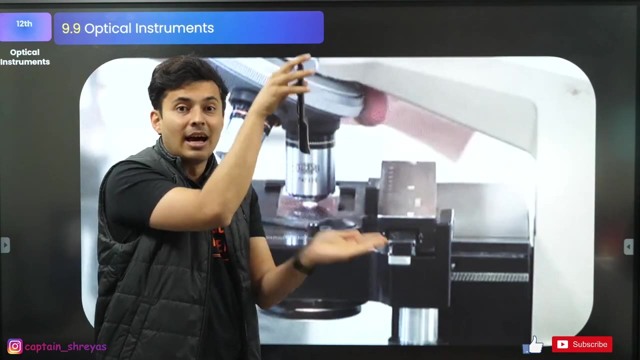 on my eye. Everybody agrees- Subtends certain angle. on my eye That means if you take one line from the bottom or the feet to my eye and the top to my eye, there is some angle between these two lines. That is the angle subtended. If Pandu comes close, the angle becomes larger. The angle: 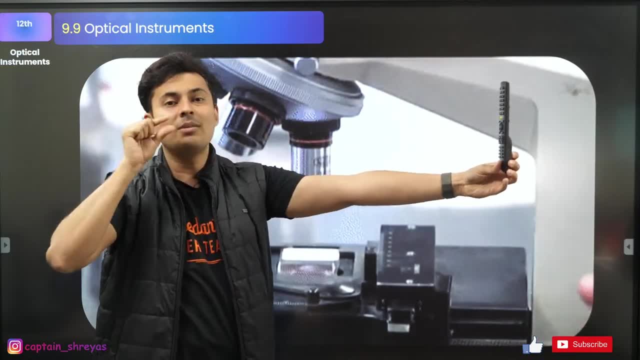 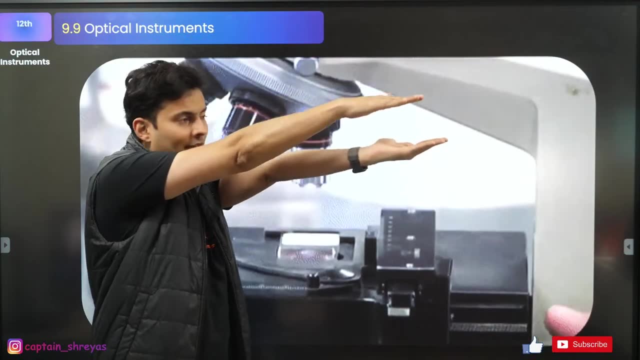 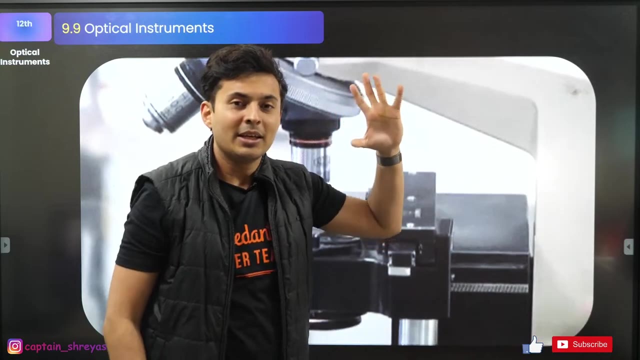 becomes larger. If Pandu goes far away, the angle becomes smaller. Now think and tell me. when you go far away, the angle subtended reduces. So that is the reason why you will not see clearly. So think and tell me. if an object subtends bigger angle, won't it be better for us? Yes, 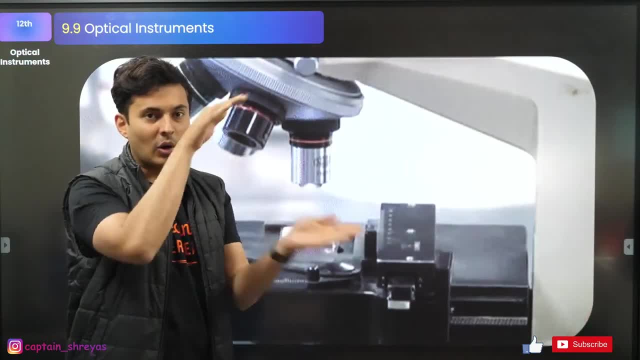 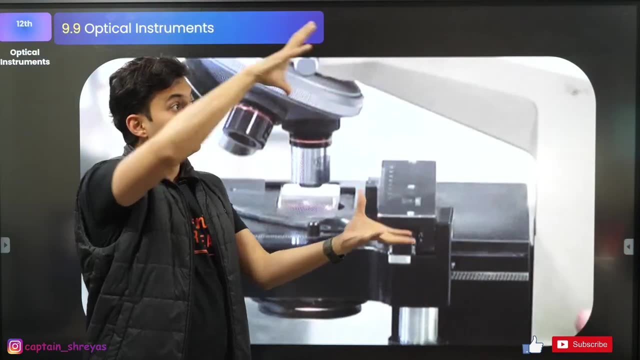 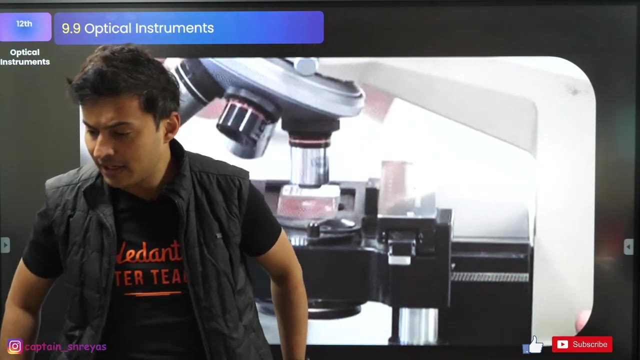 or no. If an object subtends a larger angle onto our eye, then, irrespective of whether how small or how large it is, if the angle subtended is large, you will see things very clearly. Yes, Hema, Sushant, Meena, Asa, Honey, Mimi. yes, Akshara, Shakush, Sushanta, Jewel. yes or no? Perfect. 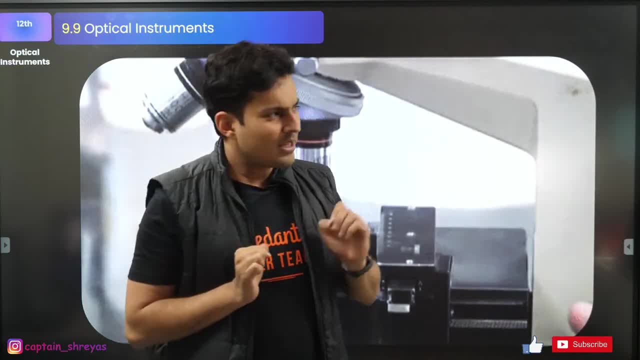 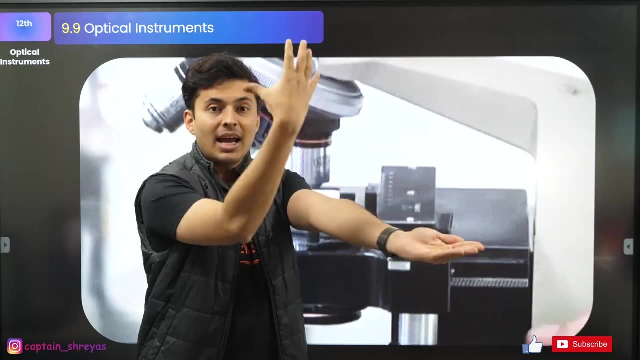 Now, that is the same principle of an optical instrument. When you look at some object which is not so clear because the angle subtended is small, with the help of the instrument, the angle subtended becomes large. With the help of the instrument, the angle subtended becomes large. 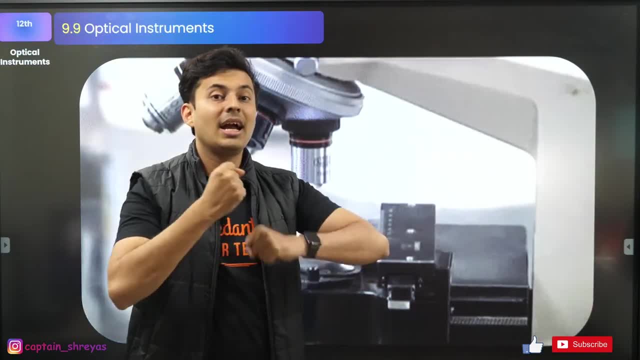 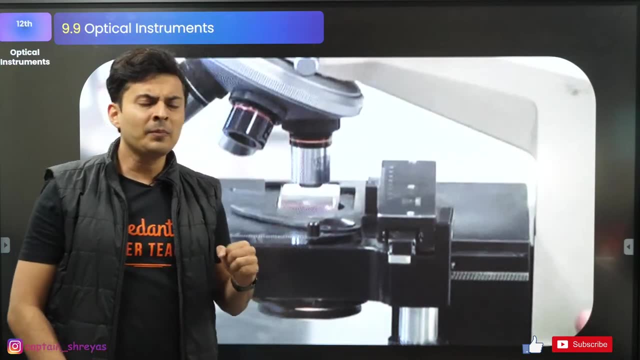 That magnifies the image as compared to the object and that's how you see things clearly, and that is taking the help of the optical instruments. But before going ahead, there is one simple property of the human eye which I am pretty sure you should be aware of, but still I 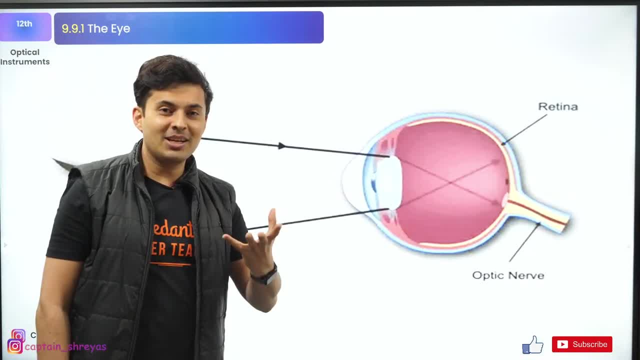 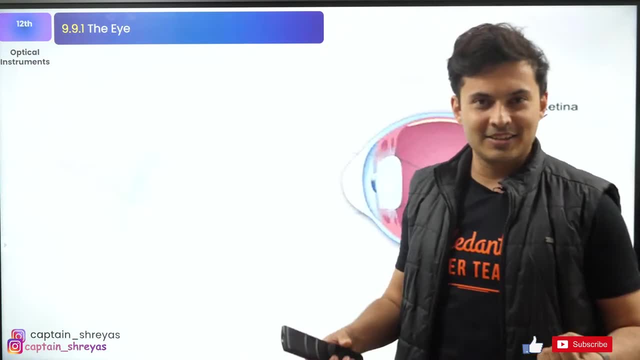 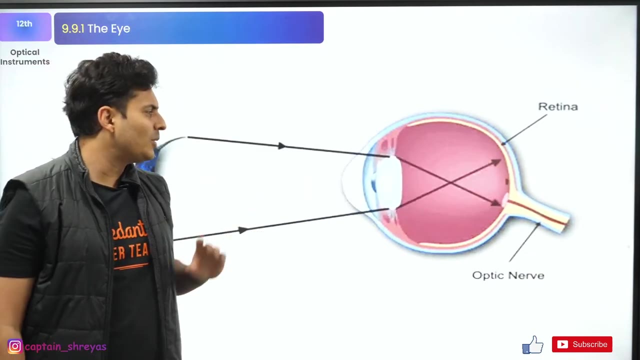 will just quickly go through it. Human eye is a very special, magnificent lens. It's a very very- you know, I would say- adjusting lens, Very special powers. it has A normal lens has a fixed focal length, but eye is not like that. 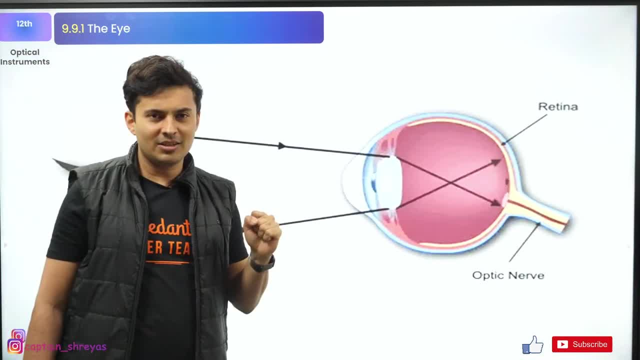 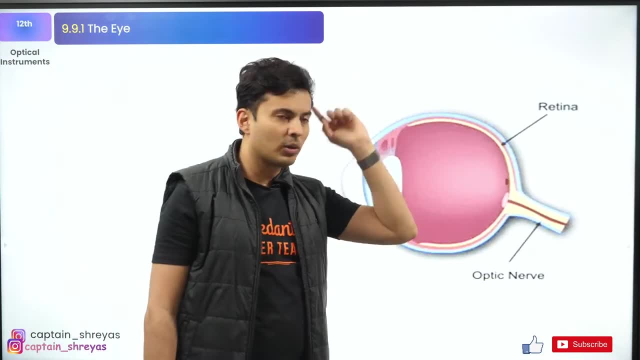 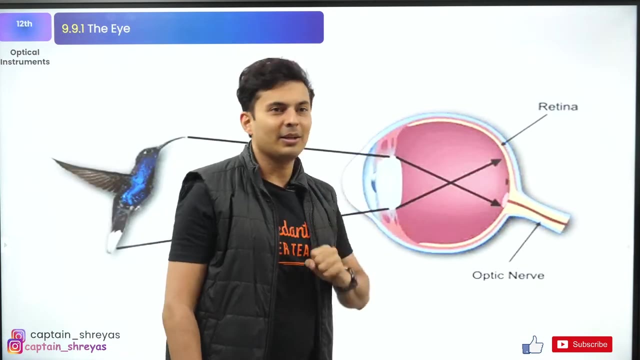 If you see something which is far away, eye will adjust itself and make the image on the retina. The retina sends those signals via the optic nerve to the brain. The brain does the processing and that's how you see the, you know object Because of the image formed on the retina. If there is no image formed on the retina, 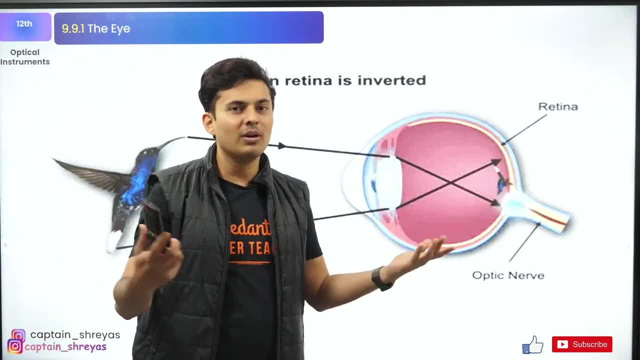 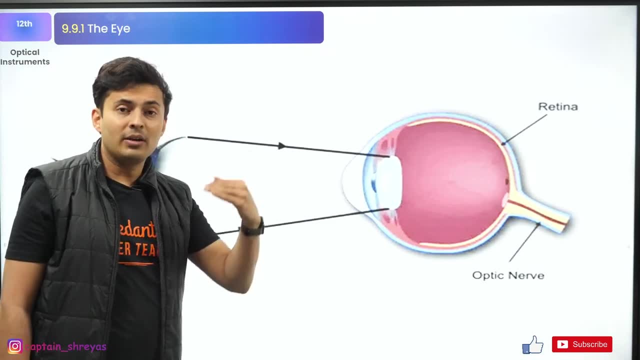 then there will be nothing seen by your eye and your brain will not be able to process anything. So your eye acts like a lens which can accommodate, which can adjust itself depending on where the object is. If the object is closed, it will adjust the focal length so that the image is 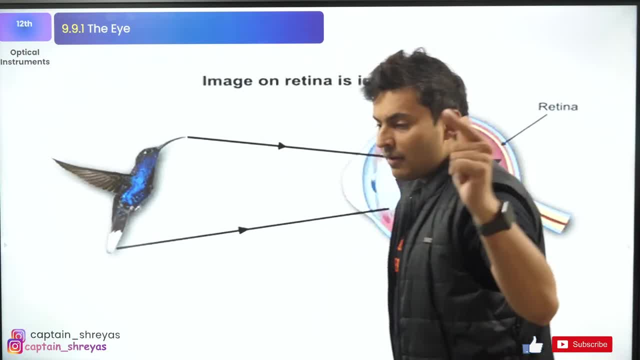 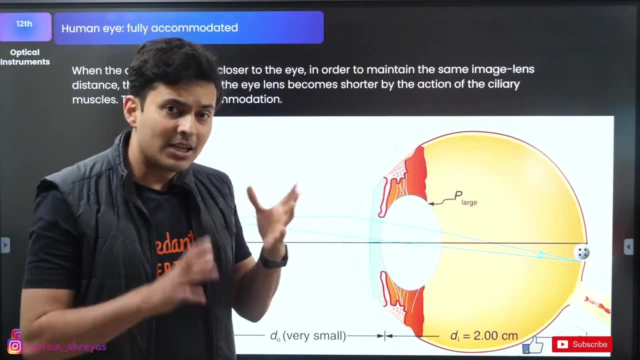 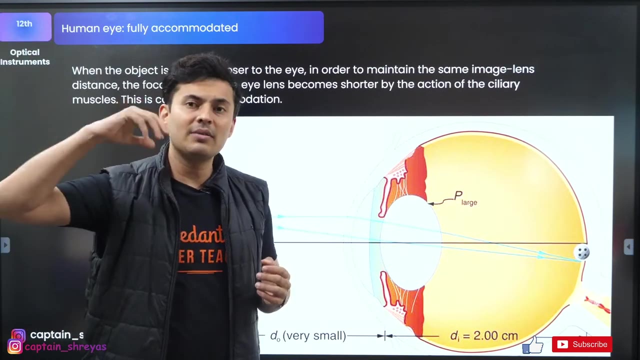 still formed on the retina. Everybody with me on this, Everybody with me on this. Good evening, Raj Ashwita. Now, the problem is that eyes can adjust itself, but not so much. you cannot be like, hey, listen, i will bring the object very close, you adjust, i'll take the object very far, you adjust, not every time the 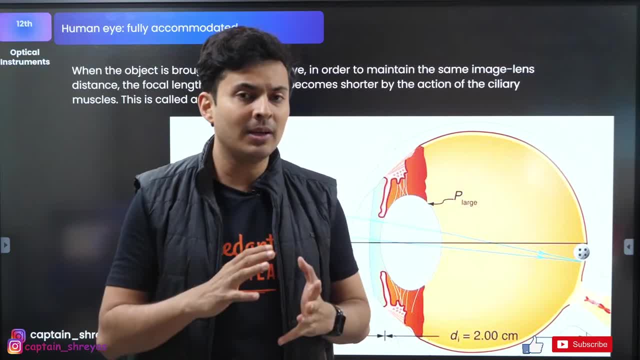 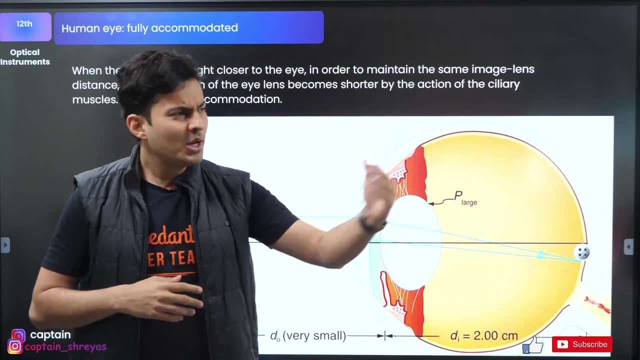 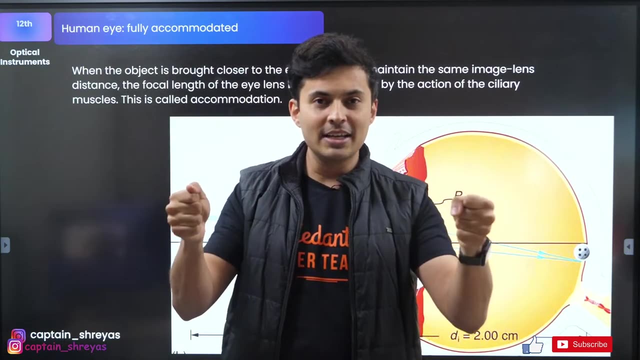 eye can adjust, so because of which there can be some defective eye or there could be a limitation to the eyes. accommodating power. so what is this accommodating power? when you bring an object close, don't you feel the strain on your eyes? try this out if you try reading a book which is very close. 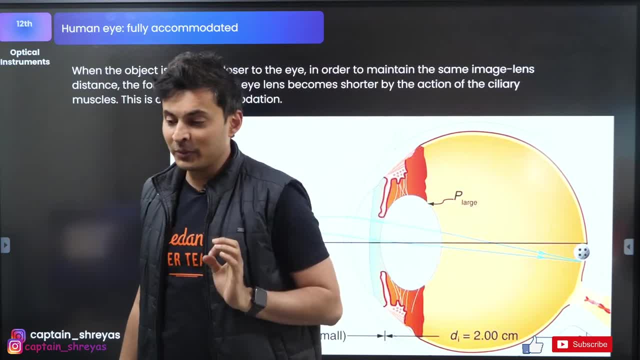 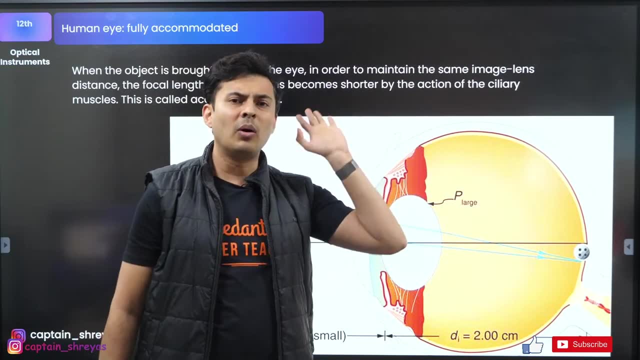 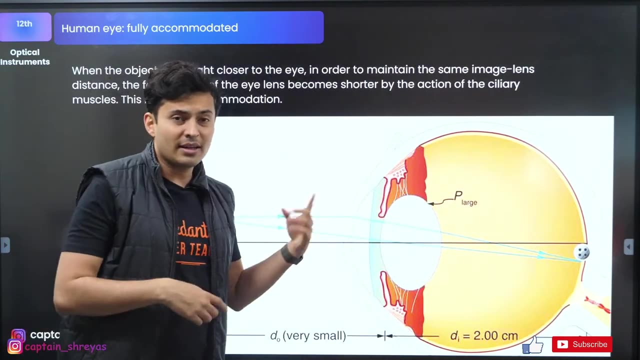 to your eyes for a long time. you feel strained. yes or no, but the same book. if it is far, if it is a far away screen or far away thing, or just staring at a mountain or a lake or the sky, it's fine. your eyes are relaxed. so that tells you the muscles which are responsible for changing the 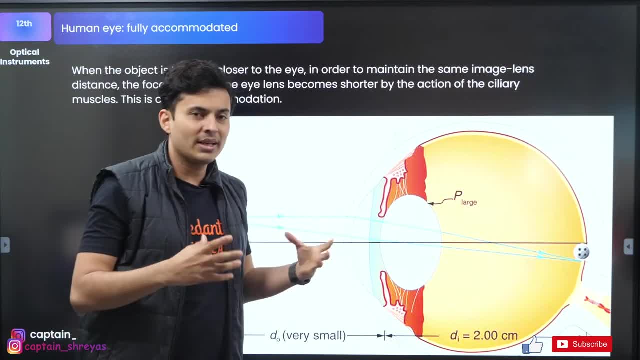 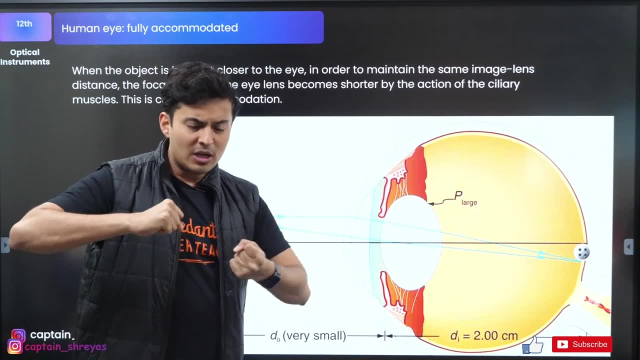 focal length. they are called as the ciliary muscles. okay, they are called the ciliary muscles. they are called as the ciliary muscles. you would have learned that in bio. so those muscles get strained. they have a lot of tension. they strain themselves when you bring the object close and 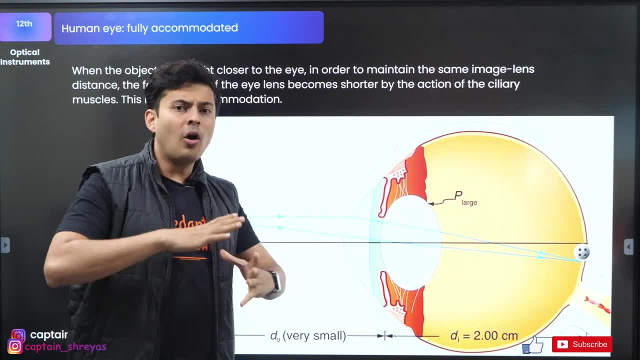 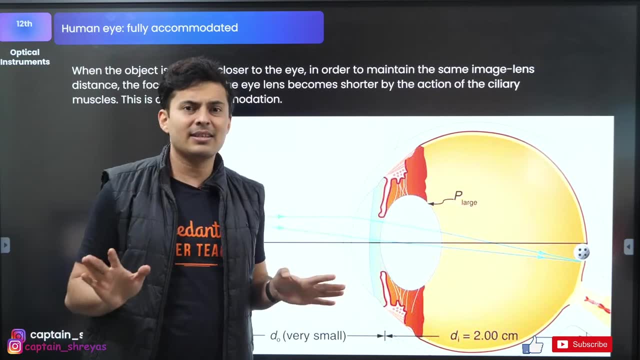 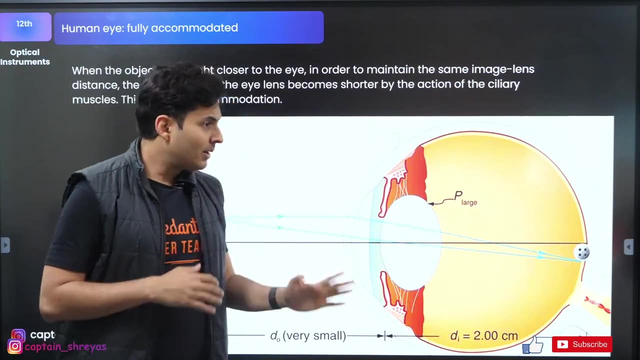 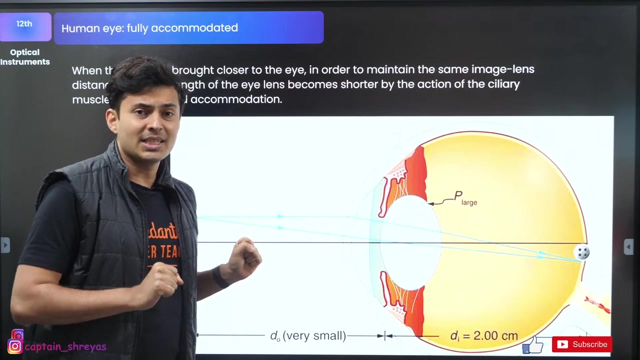 the eye has to adjust itself. when the object goes far away, the ciliary muscles relax and you will see the eye is less strained or relaxed condition and it can easily focus a distant object. now the limitation is that if you bring the object very close, if you bring the object very close less than 25 centimeters, 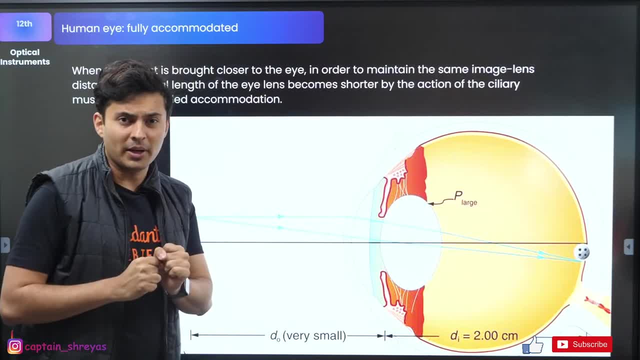 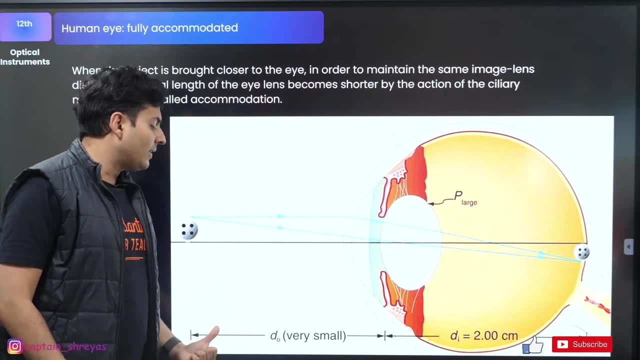 then the ciliary muscles can't strain the eye so much and the eye just gives up. it's like, okay, listen, i cannot strain more than this. so below 25 centimeters, you will see that the ciliary muscles won't be able to strain the eye. 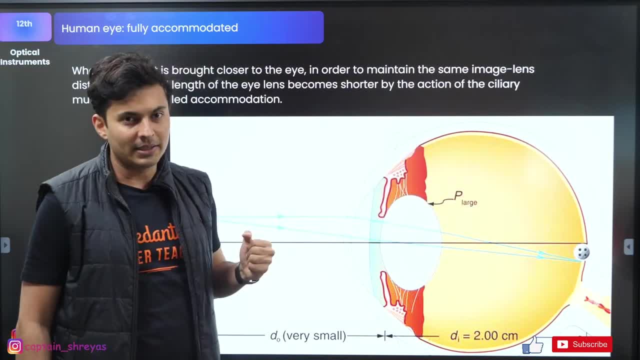 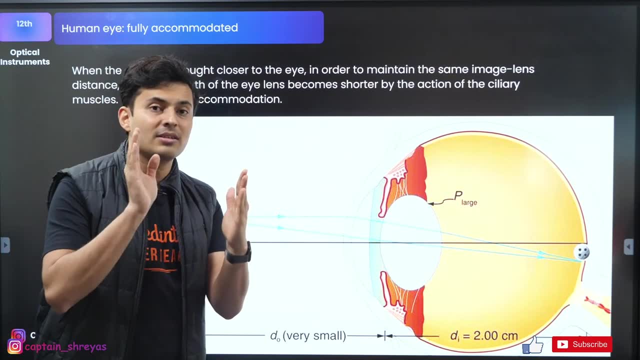 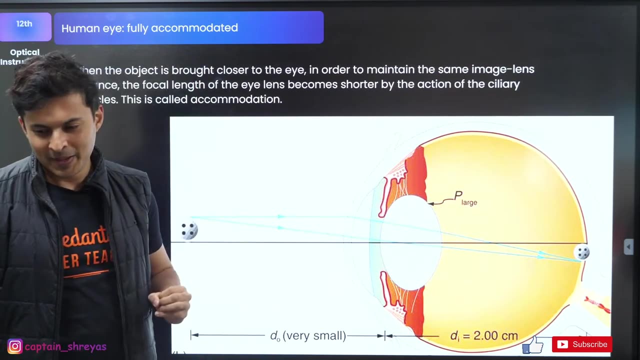 and you will not see the image clearly formed on the retina, so the image appears blurred. so hence, 25 centimeters is the least distance of distinct. that means clear vision. for a standard average human eye, okay, for a standard average human eye. kinematics: Meena Ram, I have already done it, please. 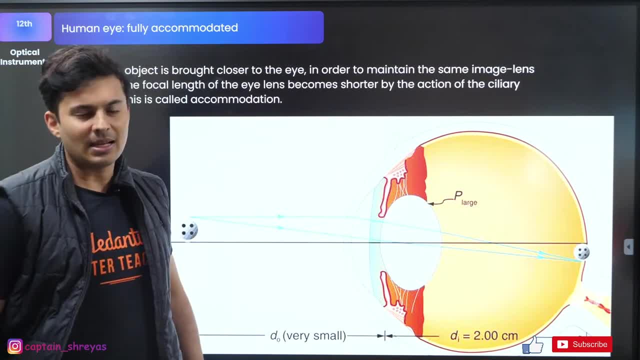 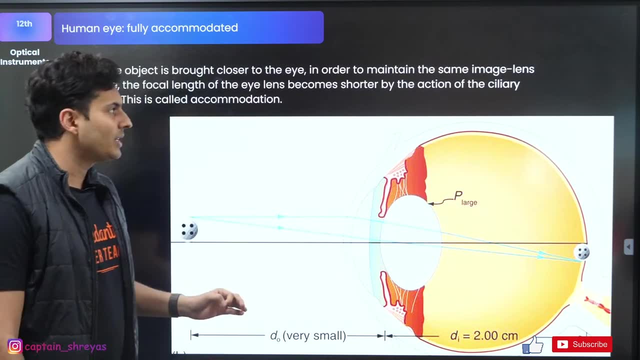 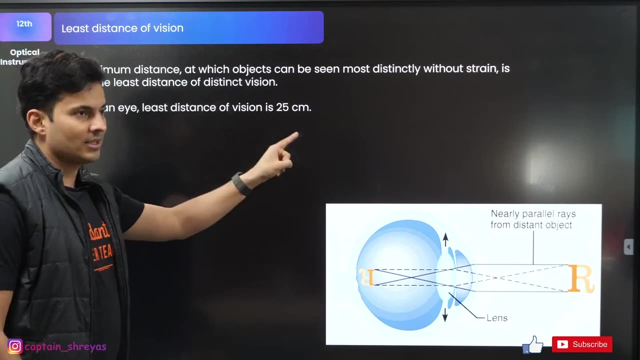 check the past videos. it's already done. if it is not there in the playlist, I'll add it in the playlist, but it's just done few days back, okay. so the least distance of distinct vision for an eye happens to be basically 25 centimeters, least distance below which you cannot see things. 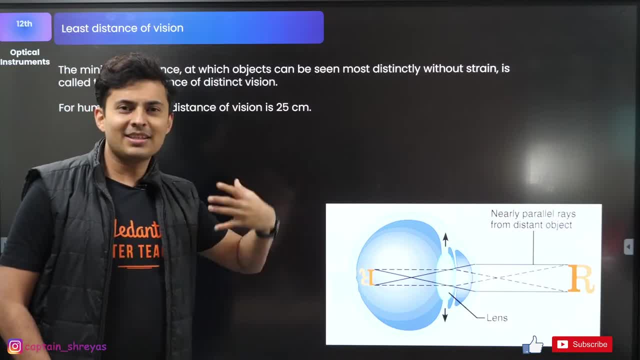 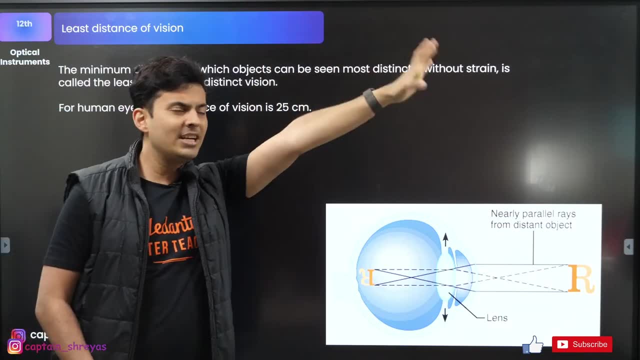 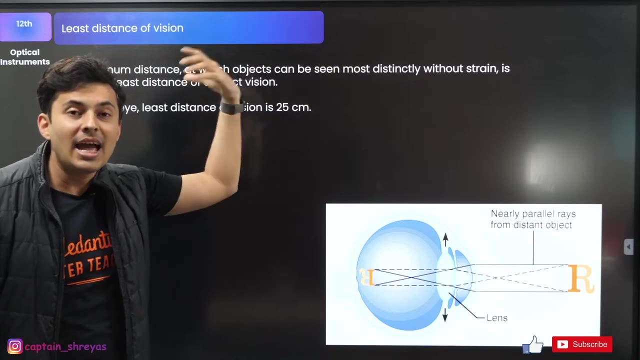 clearly, if you take things far away, then the eye becomes relaxed, it is happy and you can keep taking the object far and far and far, in fact, even till infinity. like you can see a distant star, the eye is very pleased, happy, relaxed. so that brings us to relaxed condition and the relaxed condition 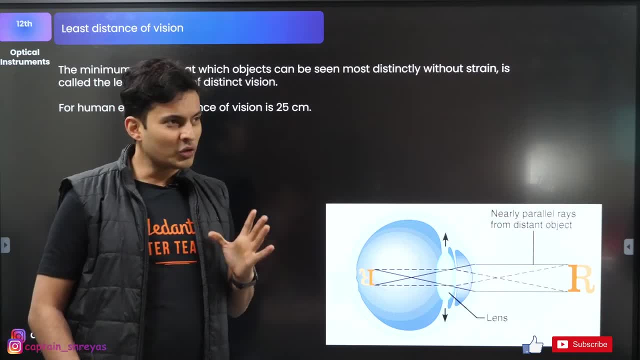 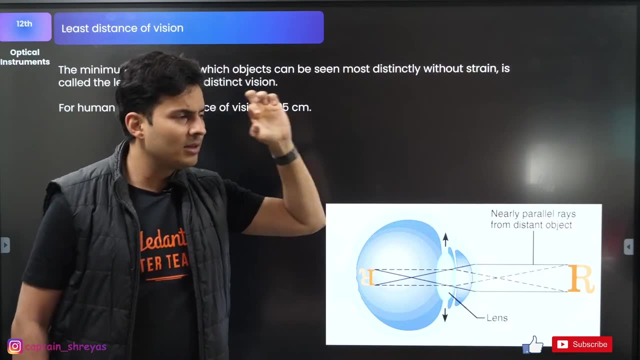 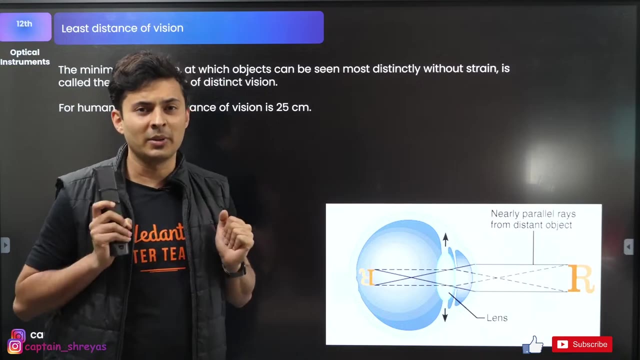 distance is infinity for a normal human eye. so even when the object is infinitely far away, the eyes can still focus on it. even a parallel beam can be focused on the eye in a relaxed state. so that is the standard, normal, average functioning of a human eye. so the farthest distance is infinity. the closest or the smallest. 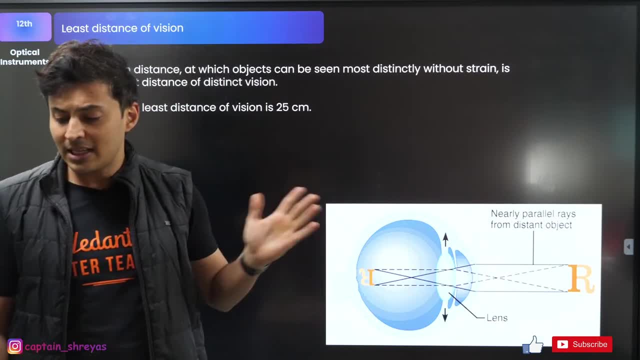 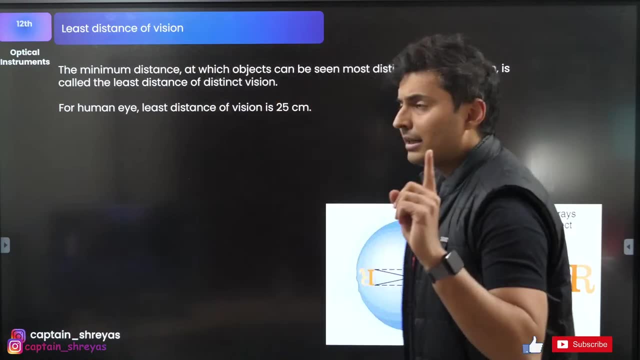 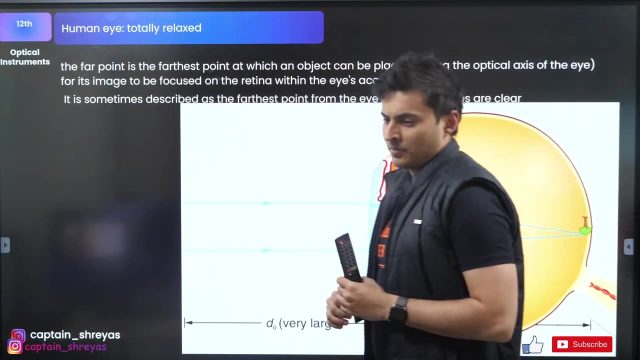 distance is 25 centimeters. everyone with me. yes, Meena Ram, that is one shot, only that is one shot, only everyone with me. clearly understood least distance of distinct vision and the total relaxed eye, which is also called as the normal vision. so least distance of distinct vision is 25 centimeters closest. 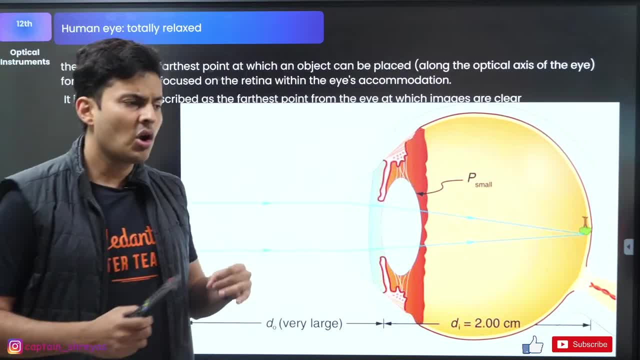 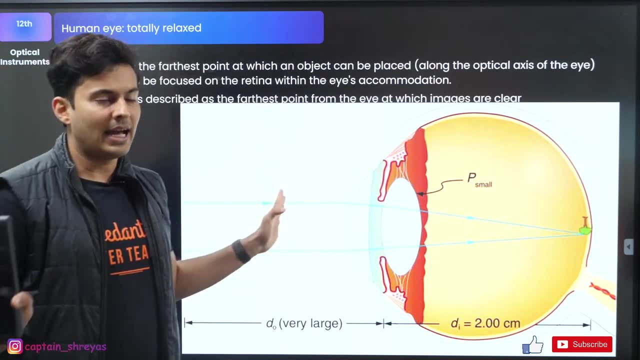 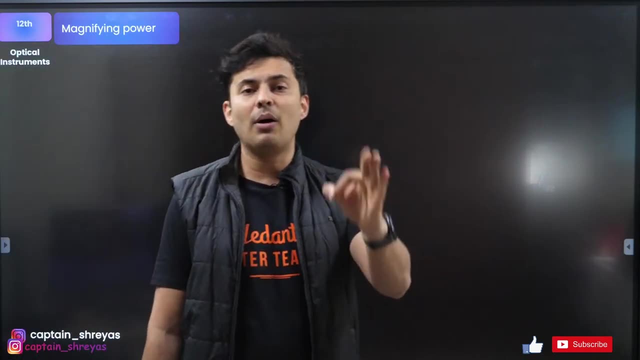 farthest is also called as far point, or relaxed eye, or normal vision, which is at infinity. okay, ciliary muscles are very chill, okay, relaxed, all right. so, having said that, let us talk about the magnifying power of any instrument. magnifying power of any instrument. so what is this magnifying? 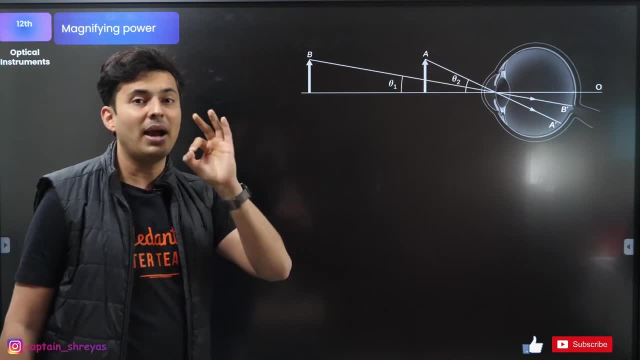 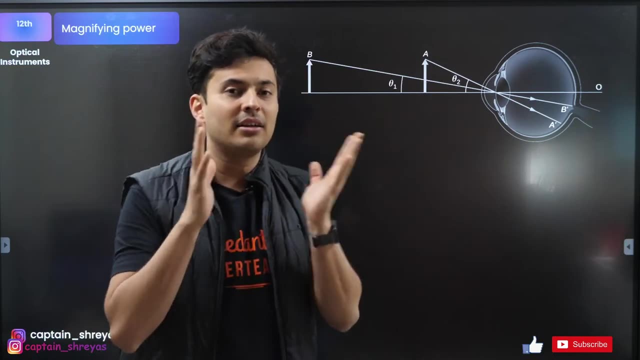 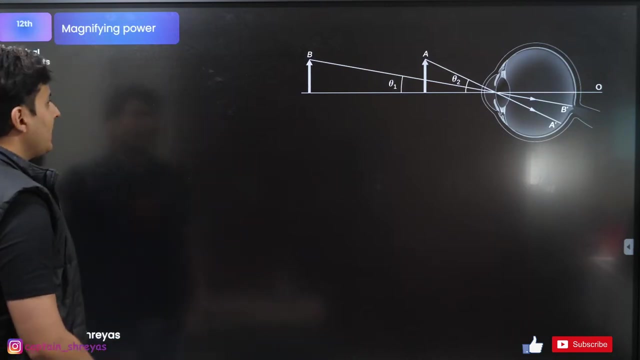 power. like I told you, the angle subtended by the eye matters a lot. the angle subtended by the object on the eye- sorry angle subtended by the object on the eye matters a lot in determining how clear, how clear and crisp the image formed is. so let me write it down over here, let me write it down over. 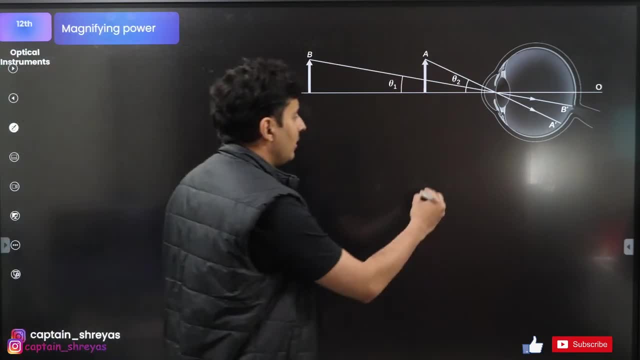 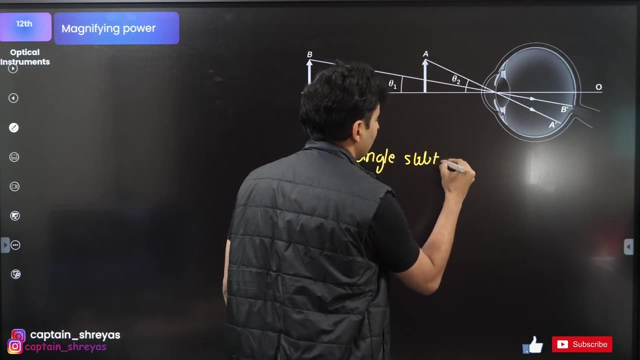 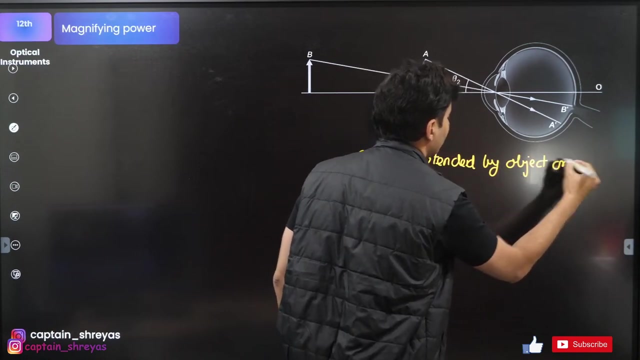 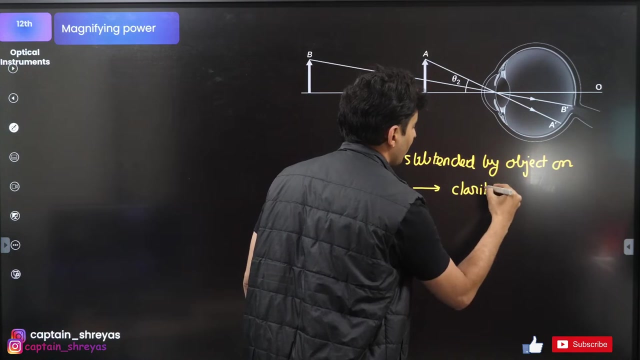 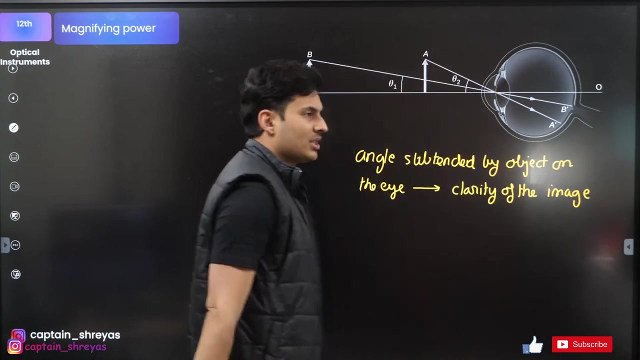 here. okay, yep, the angle, the angle subtended, subtended by the object on the eye, that is the one which determines the clarity, the clarity of the eyes, image which is formed around the sky, as we natural eyes are not just eyes, not just eyes, but the whole map of the chicken sky. looking back to theetéieren, apache br attacker, Isso é uma camôclara. ob otro can ver queouched underground of hisMicro lens on the eye. that is the one which determines reactions to clarity of the image which is formed享 mel0吃 모� PayPal de uma imagem se determina comoDisemña na compreensão de uma imagem somente? It is not clear how clearly you can think. Japan. in order to produce news, it is not possible to become do something lucratory. 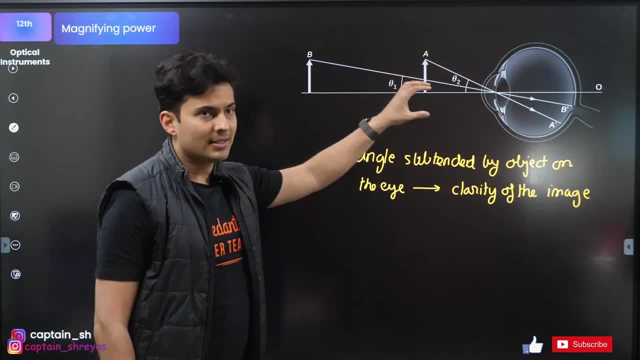 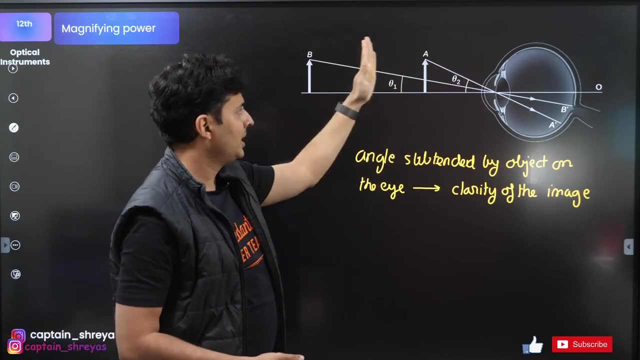 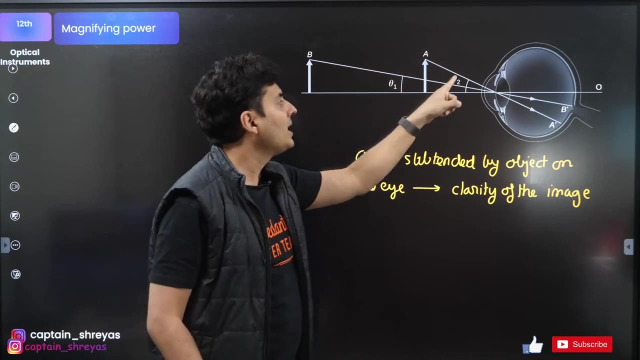 see things. so imagine, imagine, guys, when an object is over here. when an object is over here, the angle subtended is less, not so clear. the same object brought here, the angle subtended is larger. height has not changed. height has not changed, only angle has increased. that's why it is more clear when the 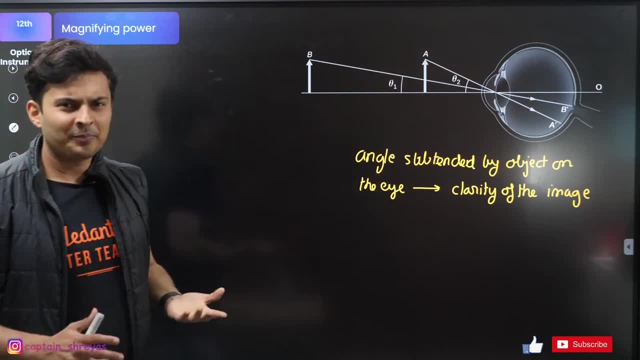 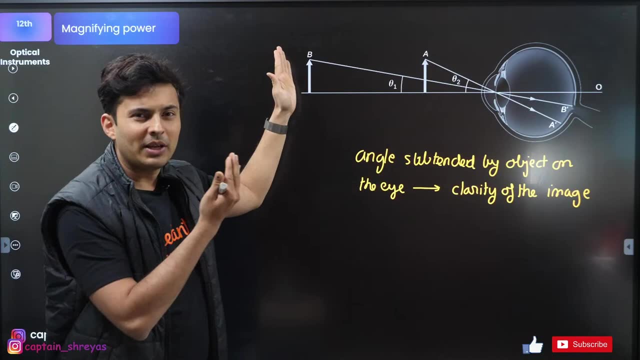 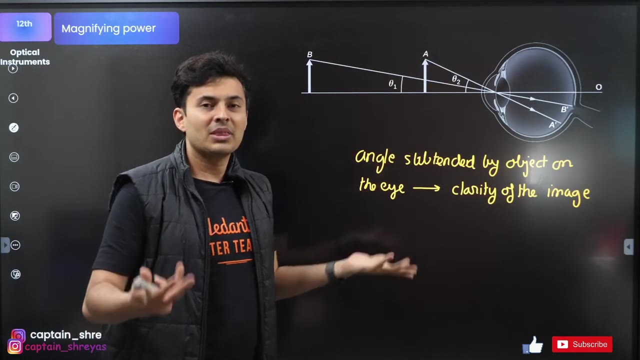 object is brought closer now. just imagine now, just imagine that the problem in most of the situations is: you might be like, sir, i can bring the object very close, very close now, sir. so then it will appear very clear. true, but beyond 25 centimeters, if you bring it also, then what will? 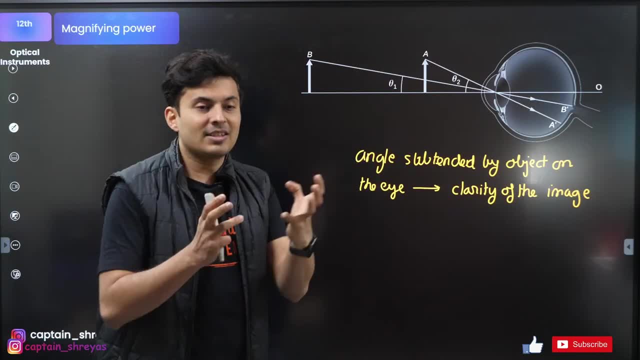 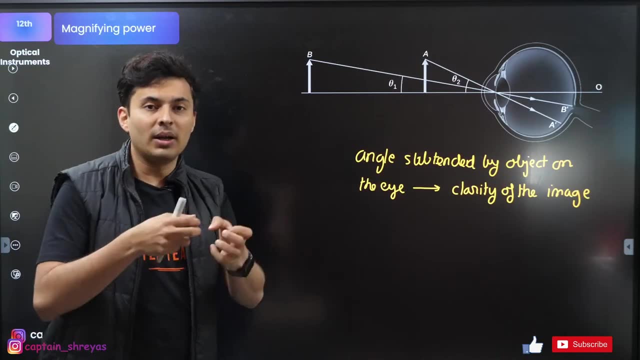 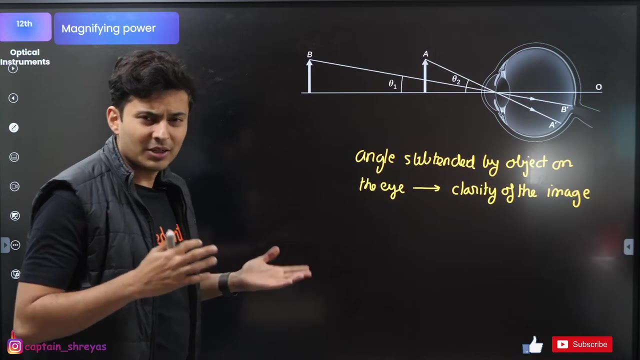 happen, you will not be able to see things clearly because that's the least distance you can bring the eye to. below that, the eye can't focus clearly because of the additional strain involved in you know what do you say? straining the eyes. so what is done usually is: 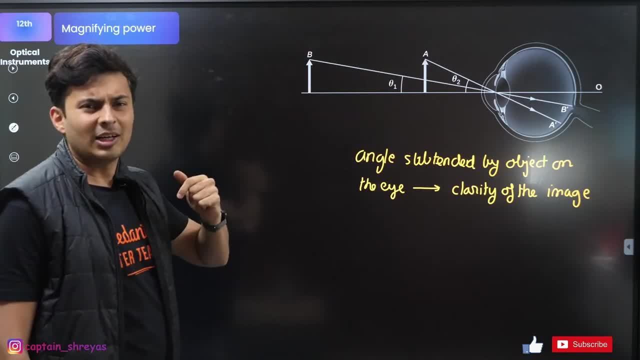 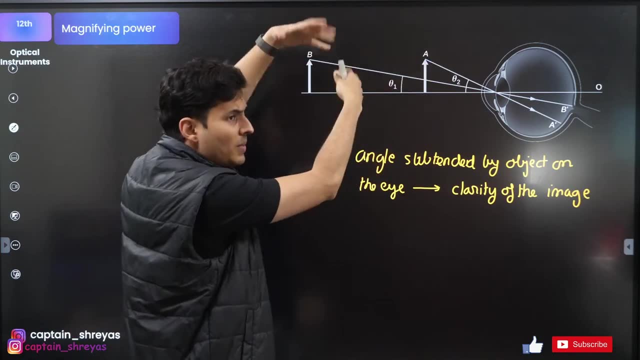 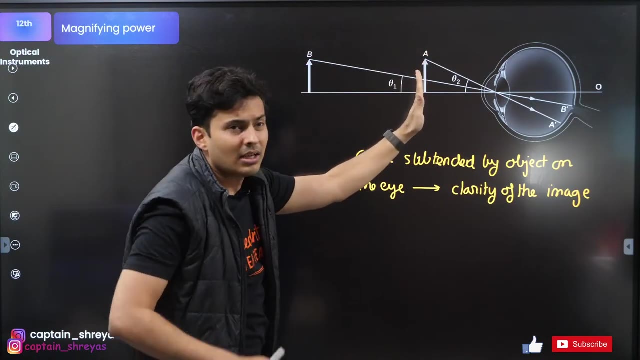 imagine you want to see an object rather than bringing it close. you make some instrument such that the image formed, such that the image formed subtends the larger angle, but it is conveniently placed at least at or beyond the least distance of distinct vision. i'll repeat, if this is an object. 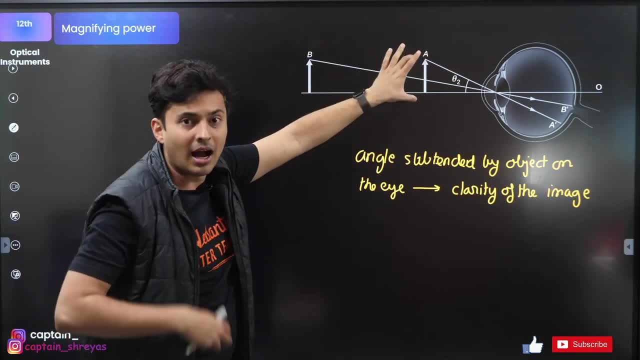 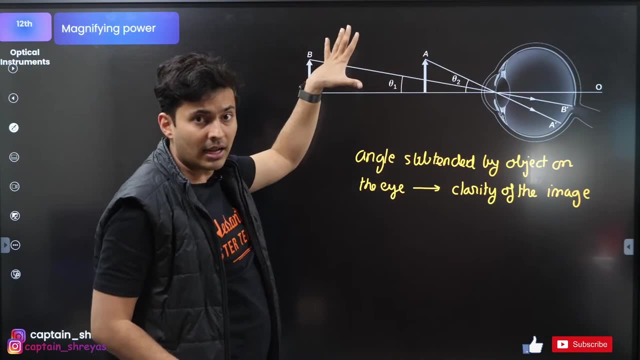 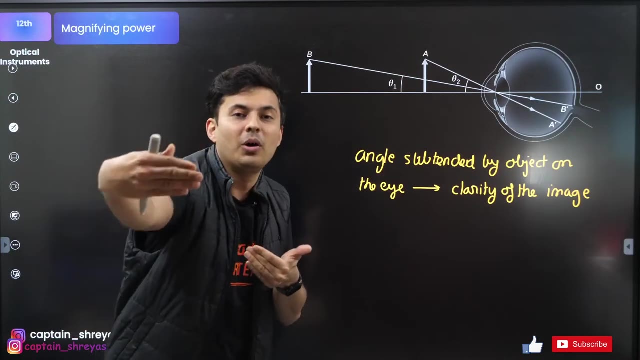 if this is an object, you make the image formed here. after some lenses, reflection, refraction, something happens. the image is formed over here such that it subtends larger angle and the image is at least after the least distance of distinct vision, because you can only focus at or beyond the least distance of. 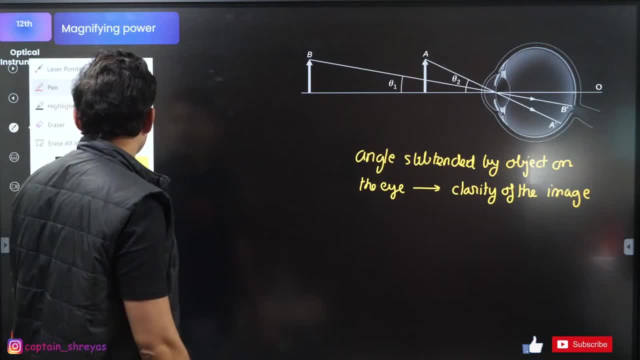 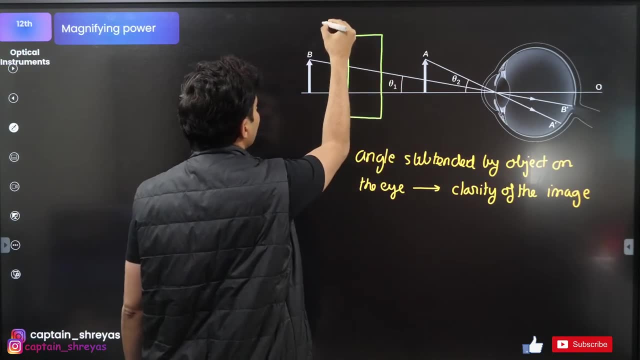 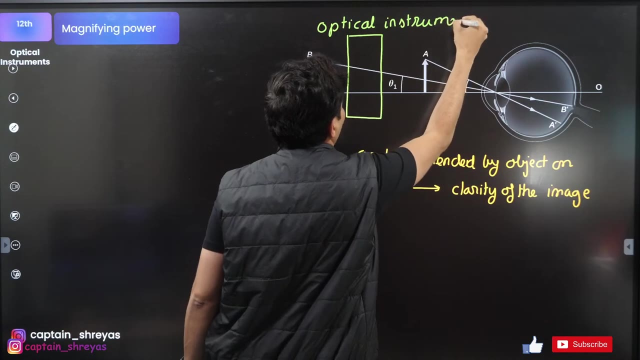 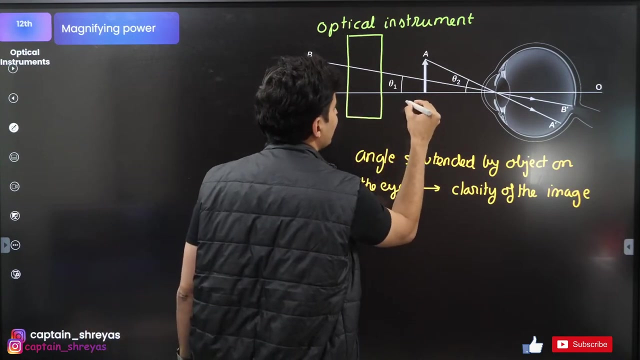 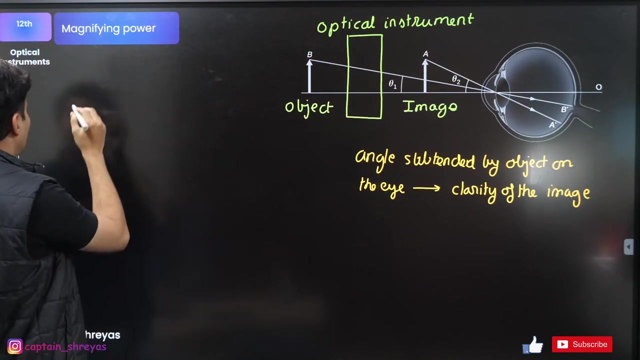 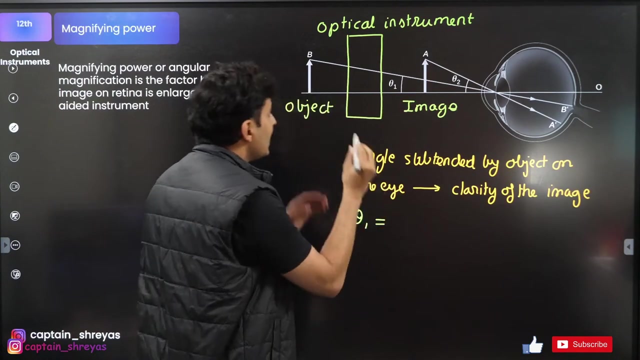 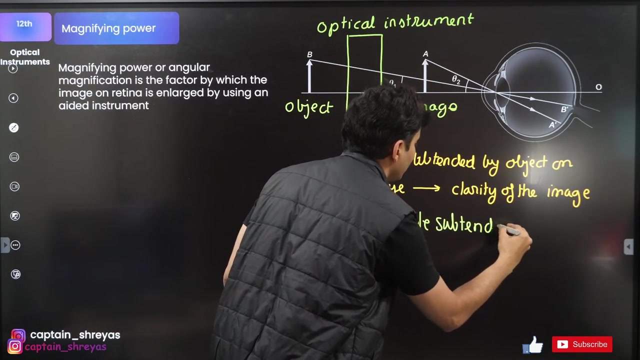 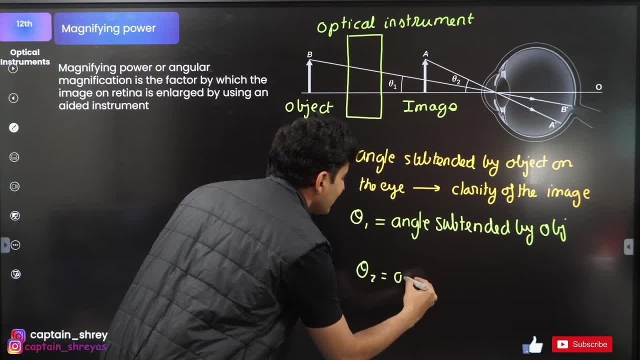 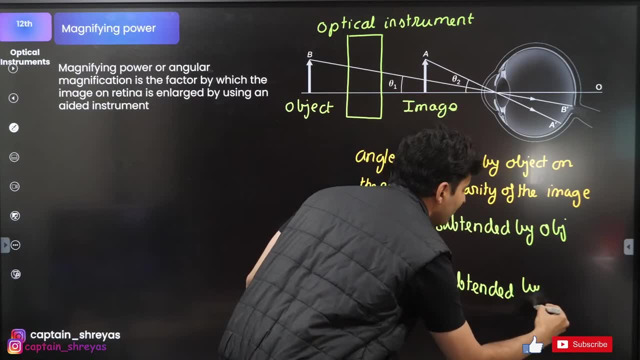 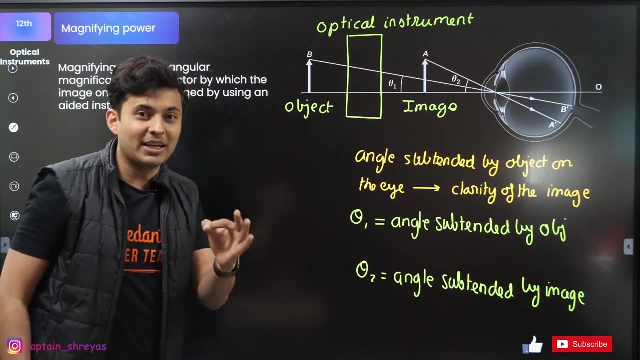 object. okay, theta 2 is basically the angle subtended angle subtended by the image. obviously it is larger by the image then the magnifying power. this is not magnification. a lot of people get confused, thinking magnification and magnifying power are the same. no, they are not the same. 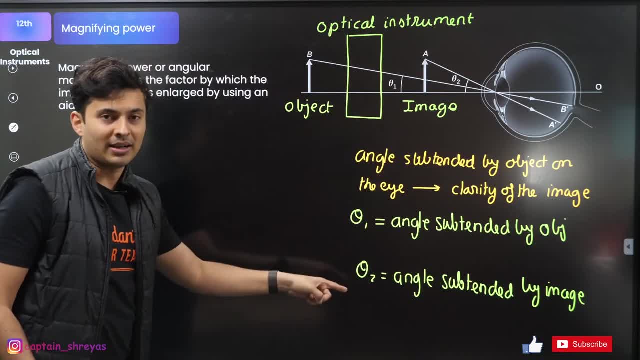 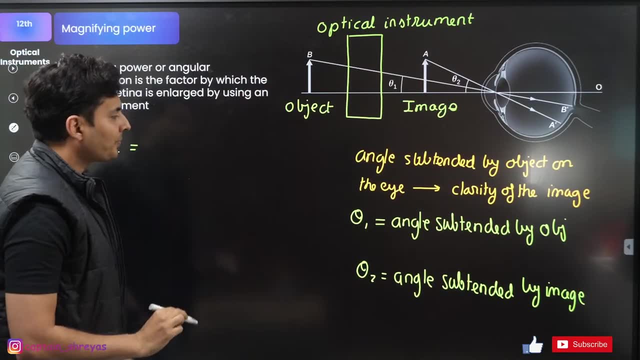 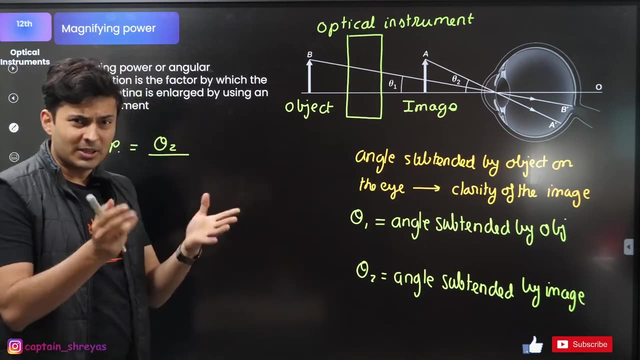 the magnifying power is the ratio of these two angles, the larger by the smaller. so the magnifying power of that optical instrument is given by the angle subtended by the image, which is in this case theta 2, upon the angle subtended by the object, which is smaller. so that is nothing but theta 1. 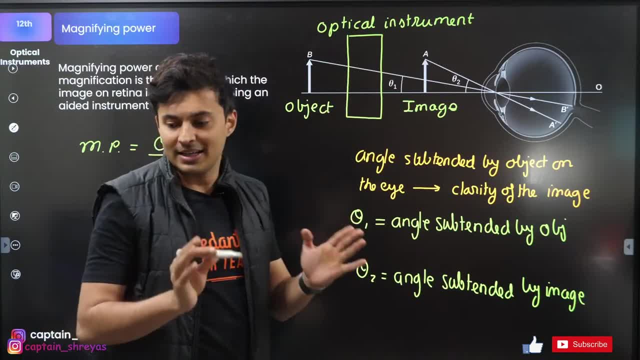 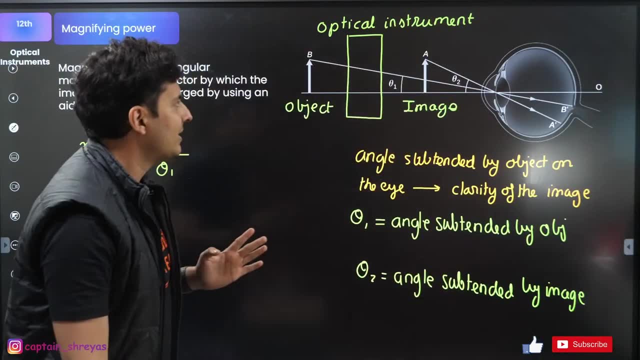 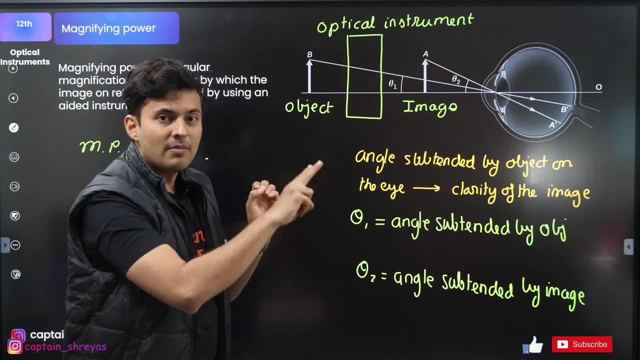 so that is what magnifying power is. that is what magnifying power of any optical instrument is. if imagine, just giving you an example- if this was 10 degrees and this is 2 degrees, the angle subtended by the image is 10. object is 2, so 10 by 2 is 5, so the magnifying power is 5x. so you would have seen telescopes or microscopes. 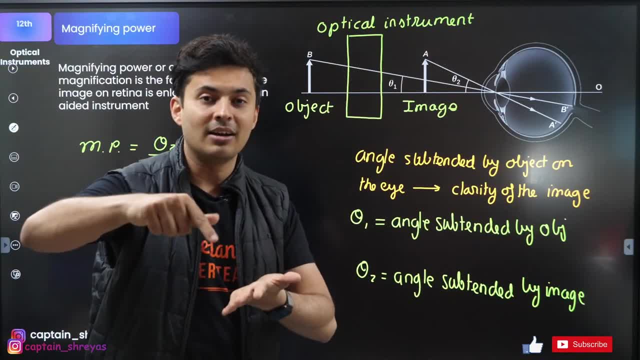 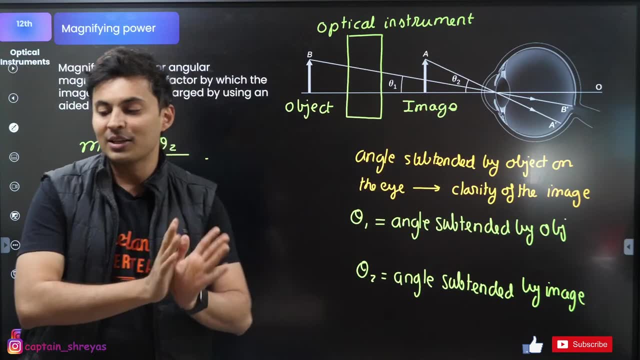 they have some number written on it- 5x, 2x, 100x, 300x, so that 300x, 200x, 100x. what is it? it is, how many times is the angle getting expanded. that is what it is. okay. i hope this is clear. 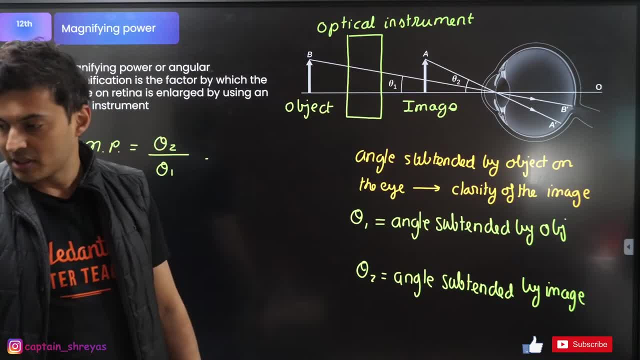 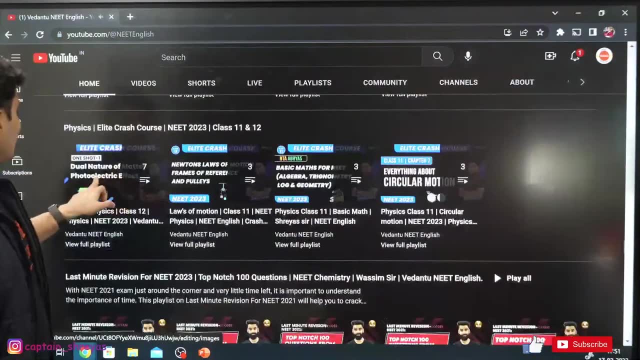 meena, it is there in the home screen. only if you see on the home screen, only right, you will be able to see it. so, as you are watching this lecture, you just go over here, just go down, you will see playlist, playlist, playlist, playlist. so i think kinematics playlist. 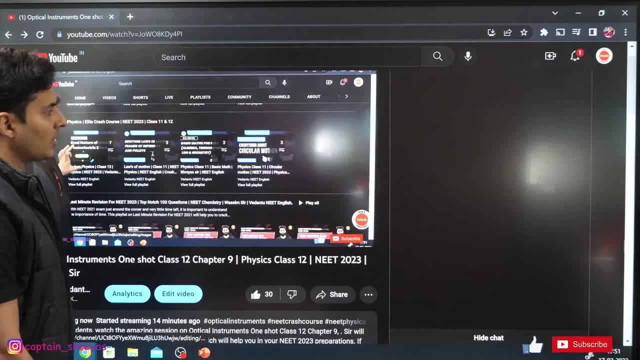 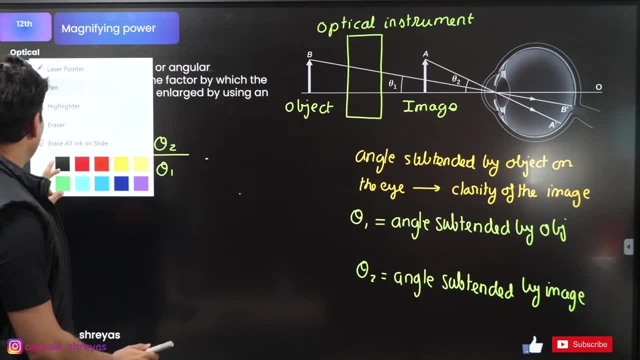 is not yet made. i'll just make sure that that is made as soon as possible. okay, after the class is over, is that okay? let's concentrate on this lecture now. so once you know this formula, let's move ahead to the next part. now, these definitions are very, very important. these definitions are: 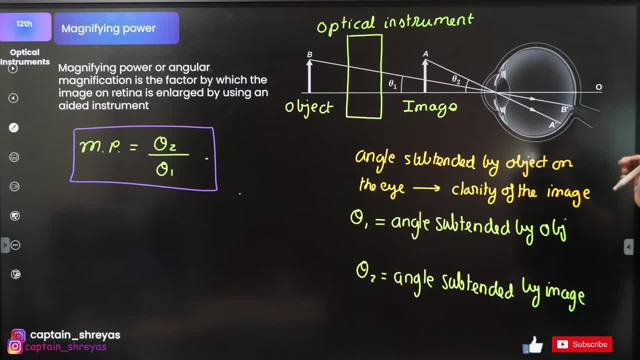 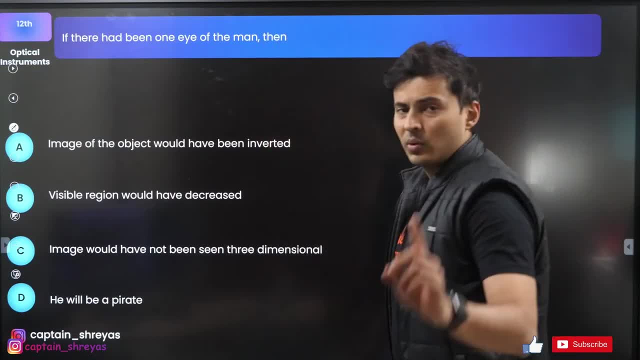 very, very important. everybody has written it down, has understood it or added to the notes more than enough. if imagine there was only one eye for a person and if you look at the person, if a person had only one eye, then which of the following will be true option? 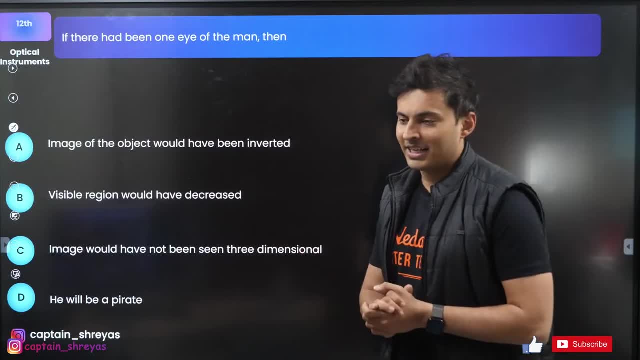 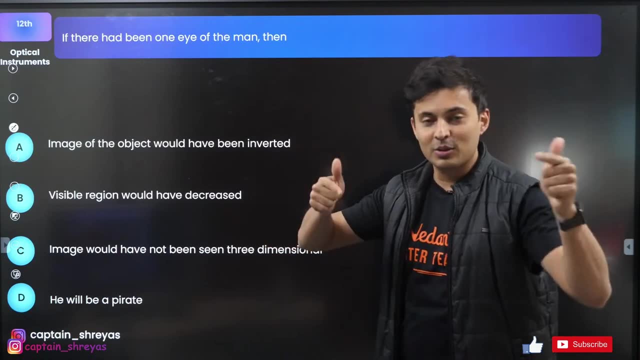 one option b, option c, option d- more than one option can be correct. come on, i want everybody to spam the answer in the chat box and if you have not yet smashed the like button, please do that right away. and if you are not yet subscribed, also go hit the subscribe button. 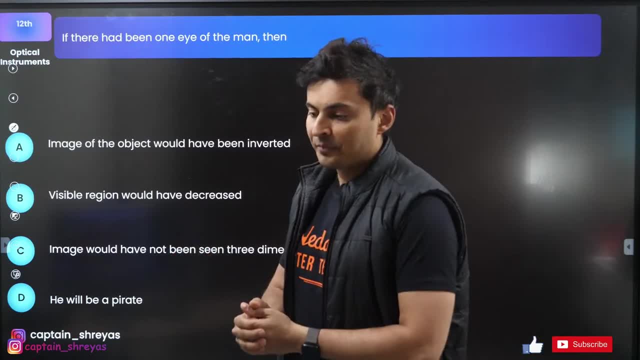 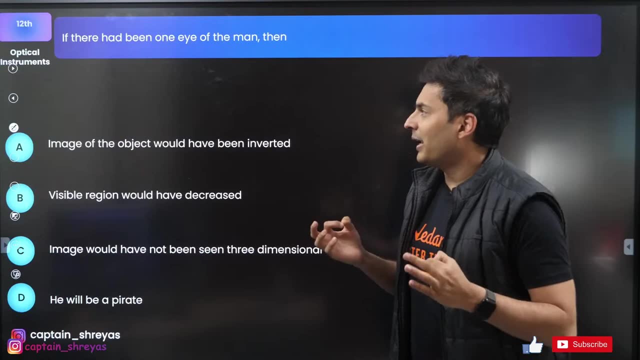 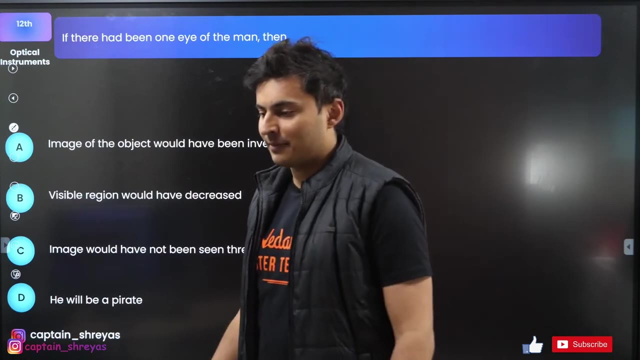 what are you waiting for? come on, you should be a part of this channel, proudly no number one neat english channel of our country. all right, so if we had only one eye, then which of the following do you think will be true? more than one options are correct. more than one. let me tell you more than one, more than: 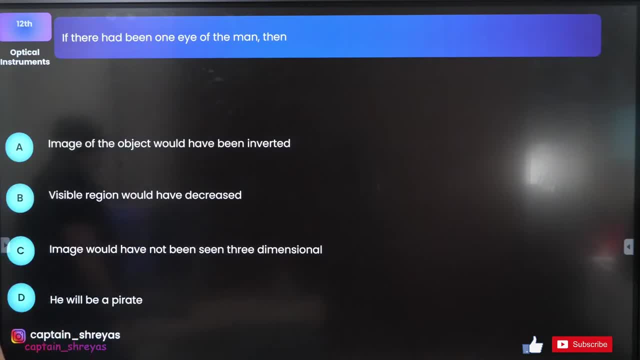 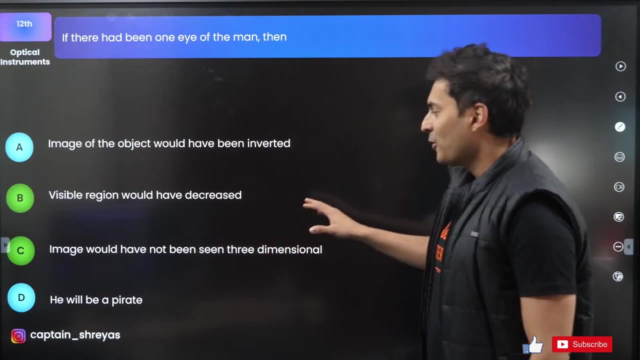 one options are correct. guys, come on, think about it. what do you think should be the correct answer? everybody is saying b visible region would have decreased. okay, i think you guys are wrong. okay. so, guys, there is one more answer: image would have not been seen in three dimension. 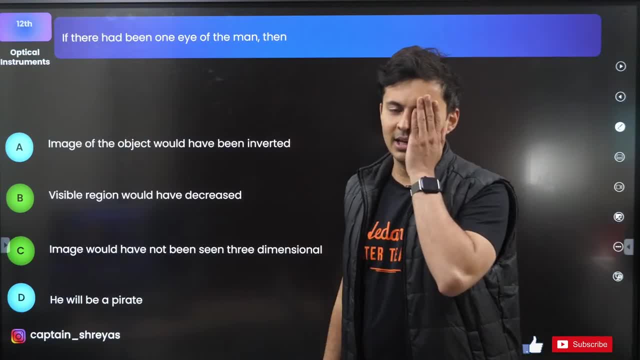 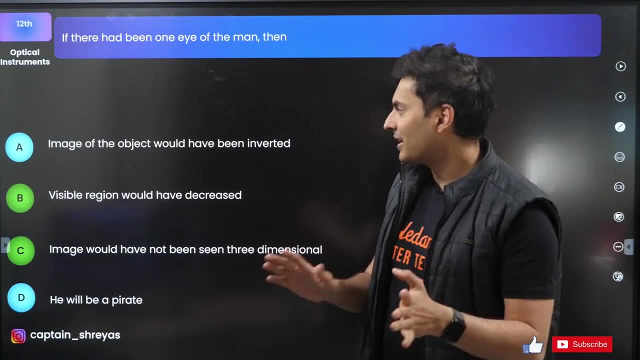 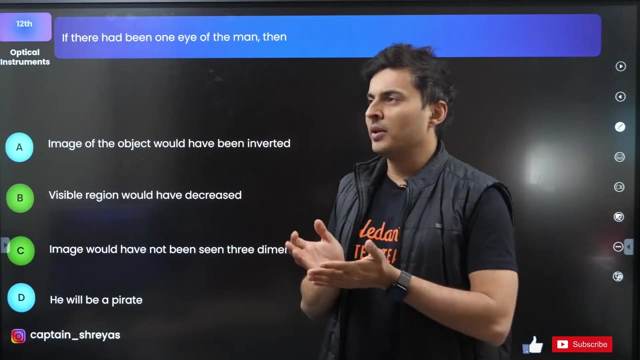 image of the object would be inverted. how is it possible? you can just close one eye and see. does everything invert? no right, nothing. images are not inverted just because you are seeing through one eye. so that is not the case. visible region would have decreased. yes, now just see anything around you with two eyes open. now just close one eye, you will. 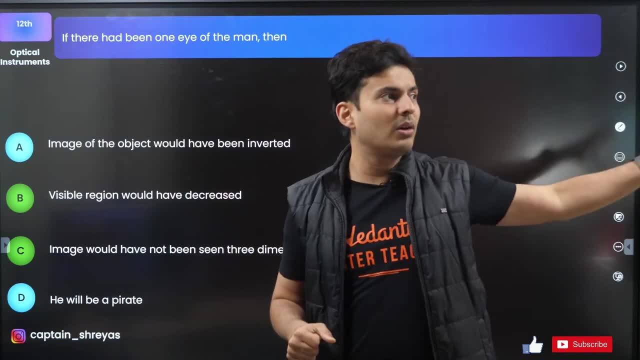 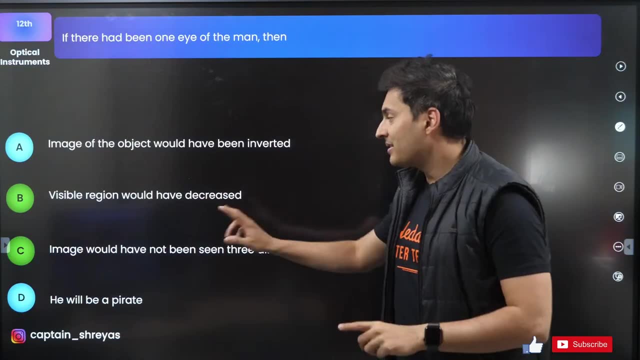 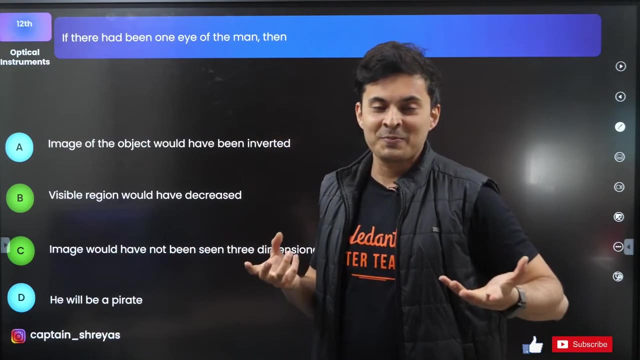 see relatively lesser number of things. a part of the things will be blinded, so your field of vision reduces. definitely correct. lot of people miss the c option. image would not have been seen in 3d, 3d, 3d effect. the depth effect comes only because you have two eyes. you get even better depth. effects if you have multiple or compound eyes, like flies or mosquitoes have. i am pretty sure you have learnt about it in your biology. so because we have two eyes, we get the sense of depth, like this eye, you know, focuses from this side. this eye focuses from this side. 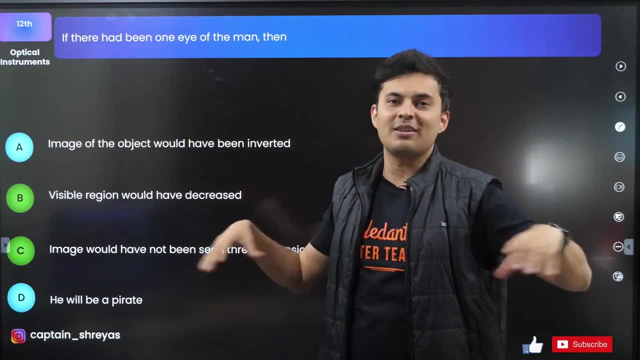 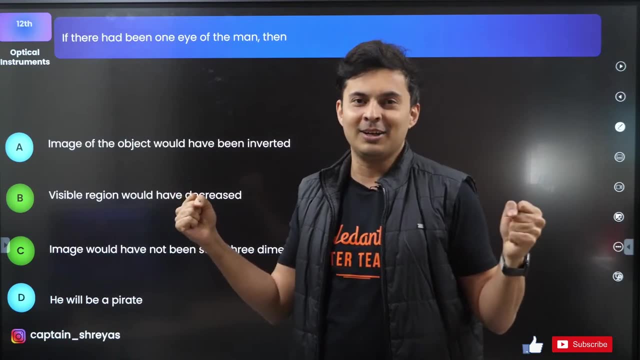 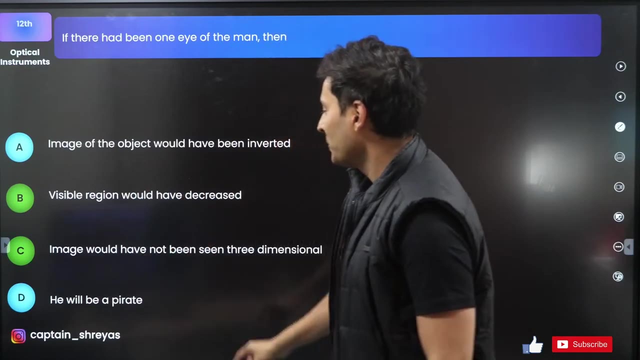 the brain fuses these two images, makes a 3d space around you internally. so the brain is capable of doing that because it has two points of accuracy accumulating the data. if there was only one point, it cannot get the sense of depth. seeing from here and here, it knows what is the depth of field. understood, he will be a pirate. what? 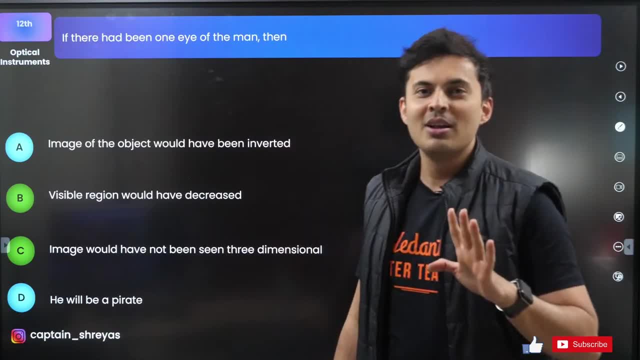 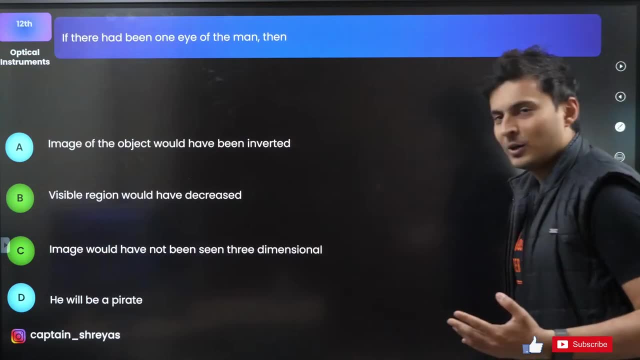 is this nonsense? no, obviously just a funny option, just kept for you. so obviously it's not necessary. but in the movies they show, pirates always have one eye. but that does not mean. but it does not mean he will be a pirate. ok, great. now let's talk about the first. 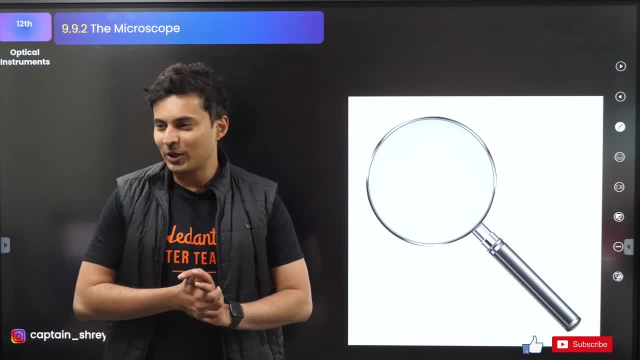 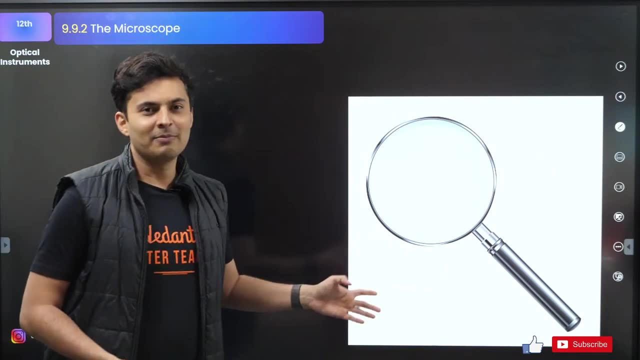 instrument bnd. Okay, yes, Vicky, not Microscope. Now, microscope has two types. One is simple, second is complex or compound. Simple one is really simple. What is this? Have anybody used this anytime? Definitely you would have used this. 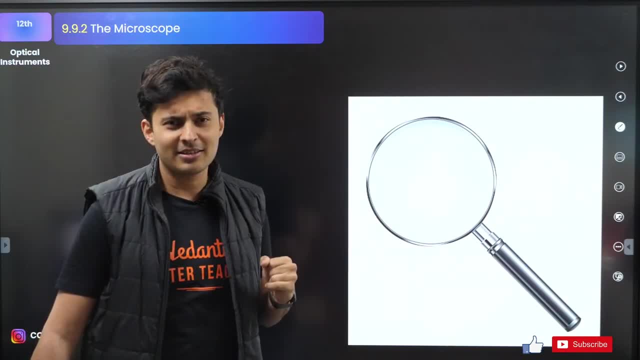 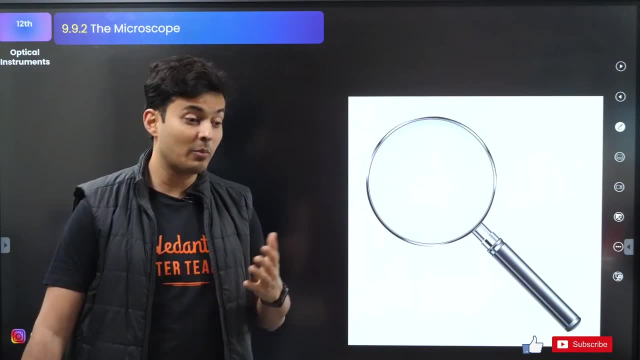 What I have seen in movies. detectives use this. What is it called? Magnifying glass? So simple microscope is nothing but a simple magnifying glass. You might have also heard about this experiment, or maybe you have done this. If you have not done it, please do it. 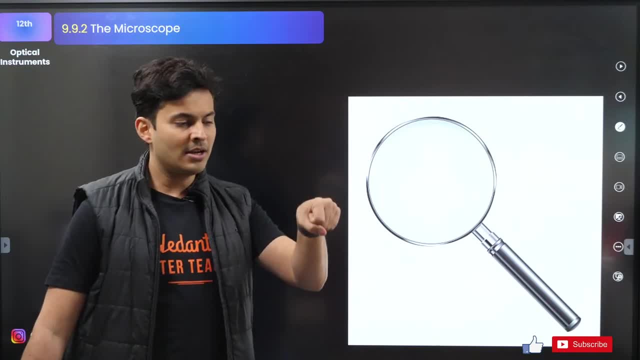 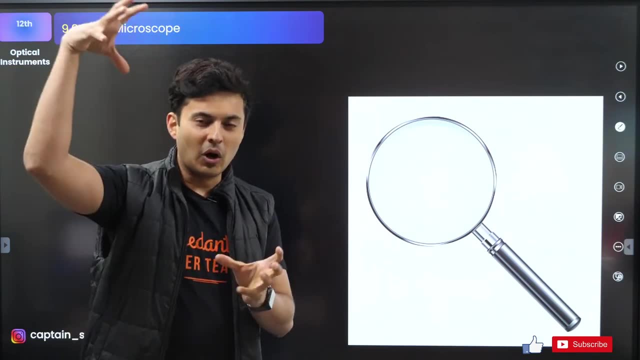 Okay, so you take a magnifying glass and make sure that the rays of the sun are falling onto it and keep a paper close to the focus. So all the rays will accumulate at a point, You will see, because all the energy gets concentrated at the point. 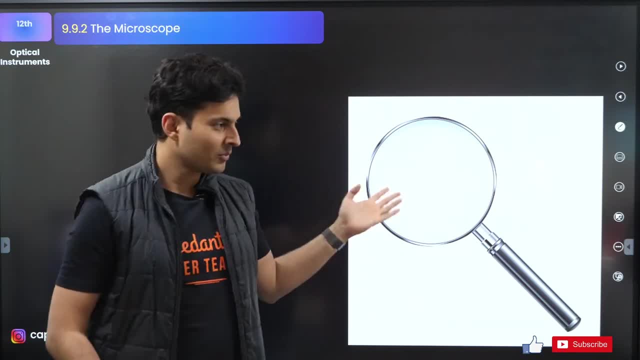 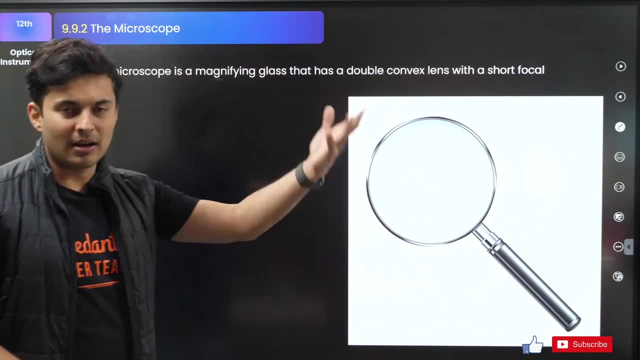 you will see, lot of heat is produced and the paper starts to burn. So that's your simple magnifying glass. and a simple magnifying glass can magnify objects around you because the angle subtended increases when the magnifying glass is on, When the rays pass through it. 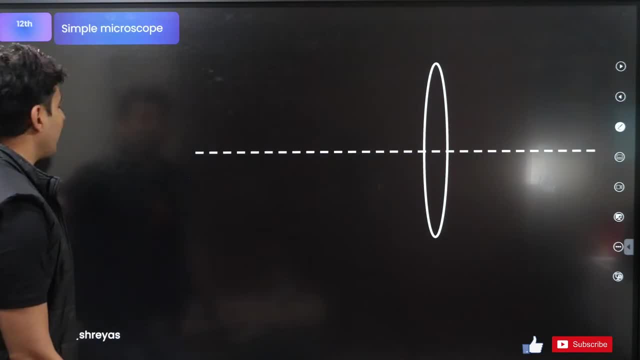 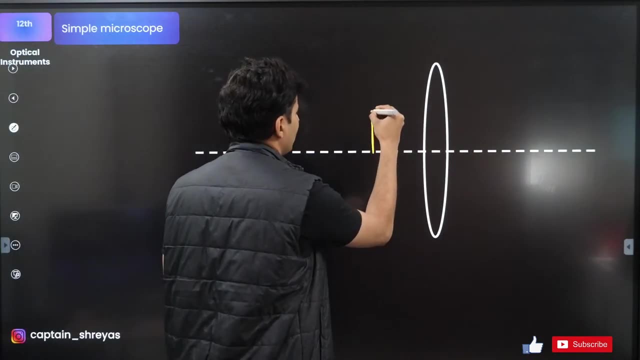 How does it increase? I will just show it to you using a simple ray diagram. Imagine you take a convex lens. Imagine you take a convex lens and let's say you place an object somewhere over here. You place an object somewhere over here. 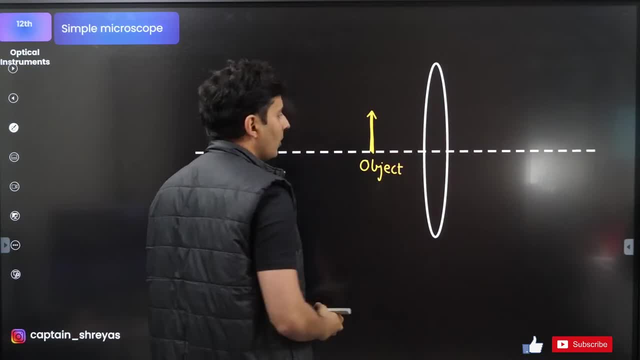 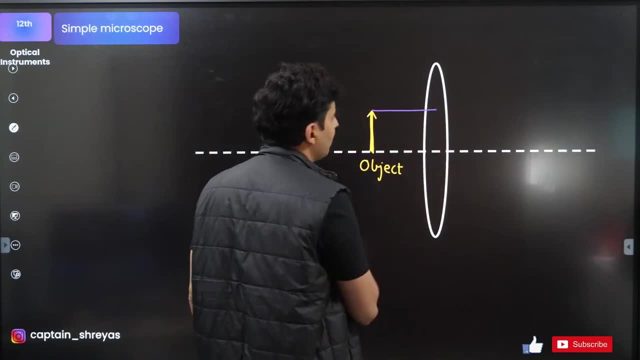 Okay, so this is your object. This is your object and the rays of the object will go in all different directions. One of the rays will go parallel to the principal axis. One of the rays will go parallel to the principal axis And after passing through the convex lens, 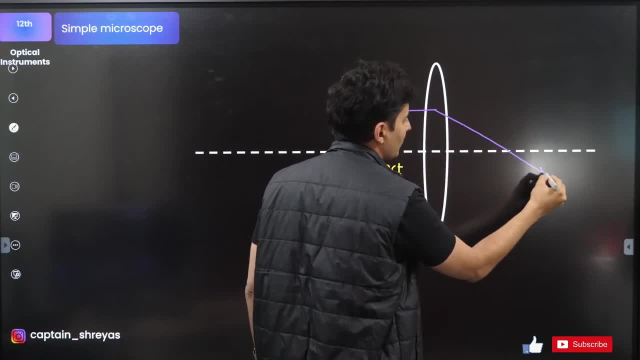 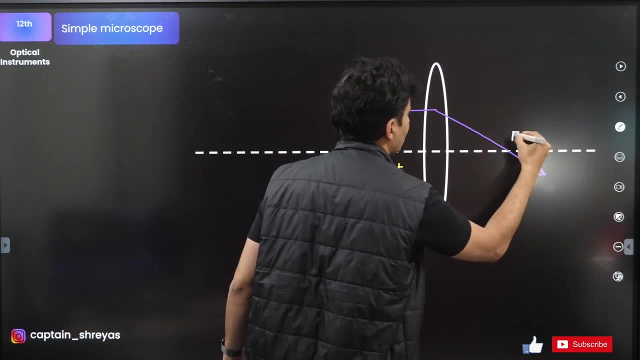 what will happen, guys? It will basically pass through the focus. It will basically pass through the focus, So this happens to be the focus of that particular lens, This is the focal point, or, from here to here will be the focal length of that lens. 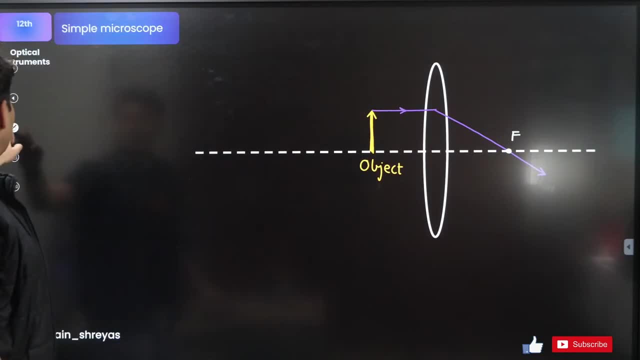 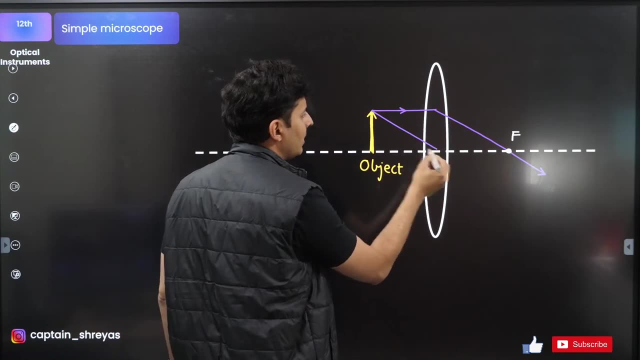 You can take many more rays like that. Let's say, I take one more ray like this which is just going to go through this center or the pole. You will see the ray which passes through the center. because the ray passes through the center, Basically it goes undeviated, like this only: 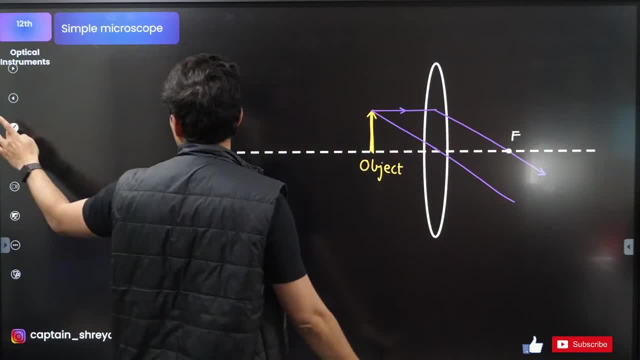 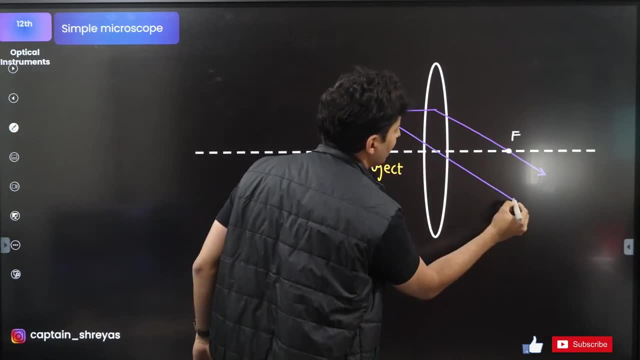 Now I know the rays are looking almost parallel. That's just because of the drawing, But actually they will not be exactly parallel. So let me just do one thing. Let me just show one of the rays over here And let me just redraw this, which will suit my purpose. 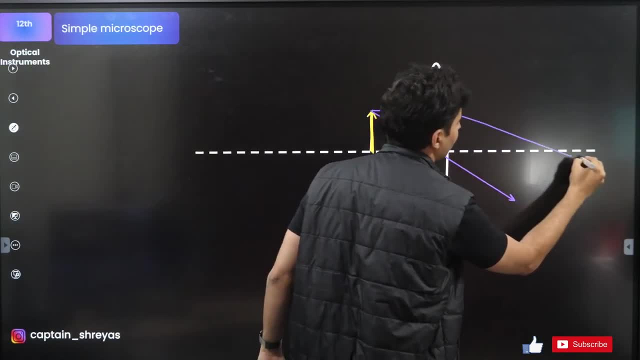 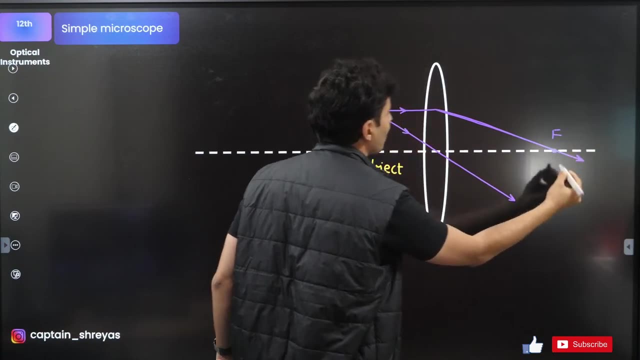 Which will suit my purpose, So maybe I will just show it like this. Okay, so now I think things are little bit better. They are not looking parallel so much. Now these two rays are diverging rays And you will see that when extended backwards. 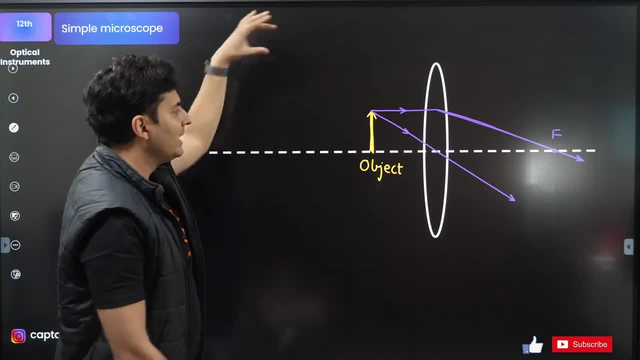 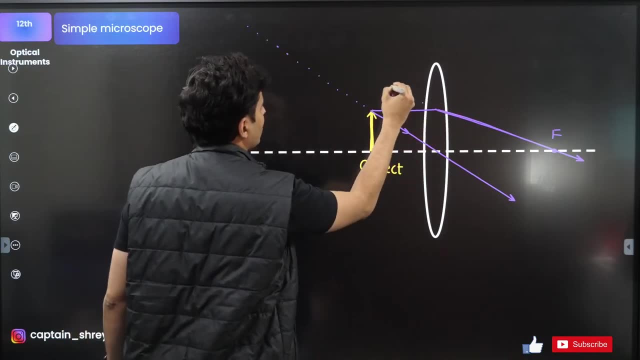 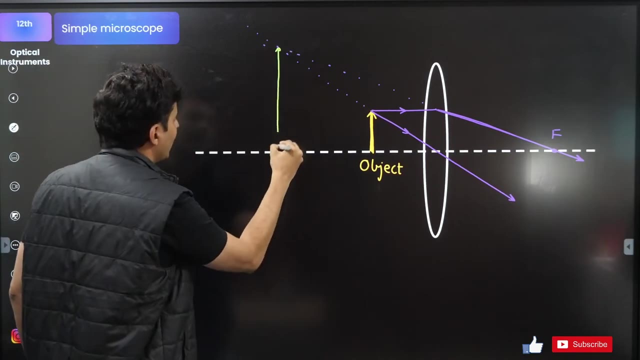 When extended backwards, what will happen? They will meet somewhere. So if you extend this backwards somewhere over here And if you extend this also backwards somewhere over here, You will see that they meet somewhere. So this is the location where you get. 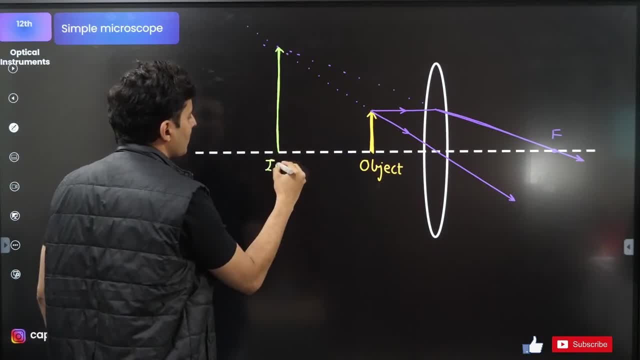 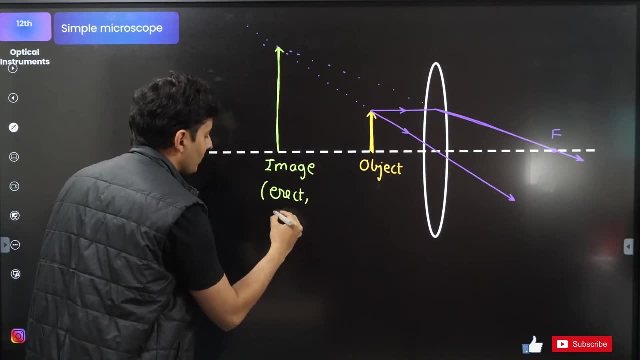 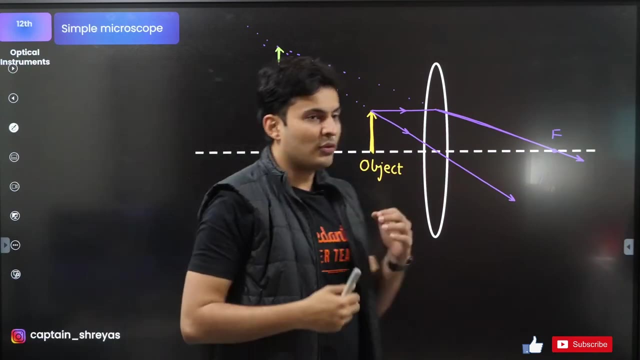 What kind of image guys? Look at this. This is your image. This image is Not only erect, But it is also enlarged. That means magnified. It is enlarged And because it is behind the lens. So if you are seeing from here, 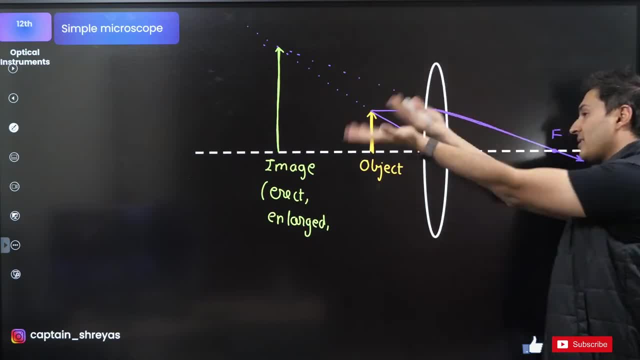 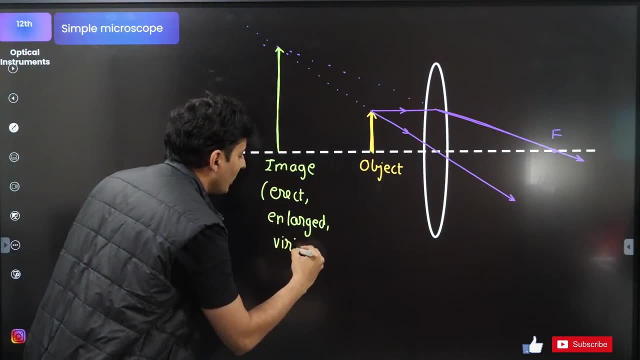 Look at this object, You will see its image little bit bigger on the same side. So you don't need a screen. It's a virtual because you have to extend these lines. So it is also virtual in nature. It is also virtual in nature. 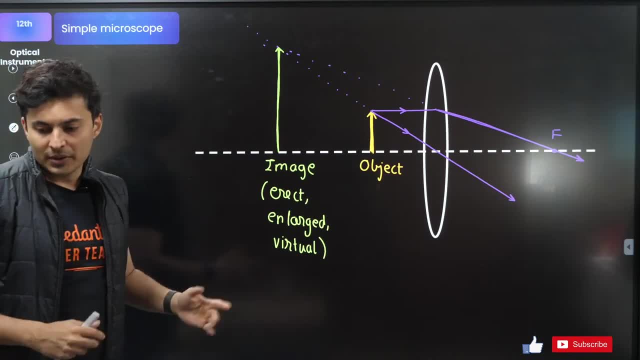 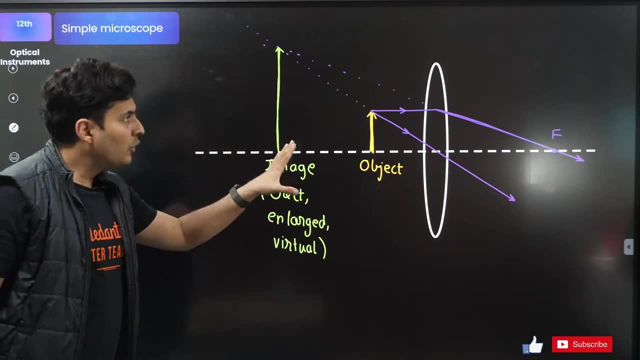 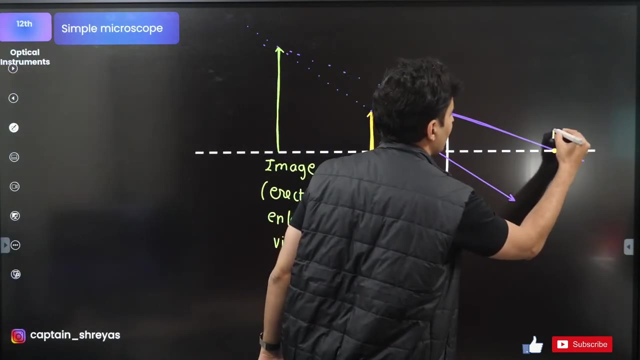 Everybody with me, Everybody with me. Very good, Good evening, Jaya. Yes, Excellent Now. Now, If you notice where the object is placed, Technically, the object should be placed. This is the focal length. This is the focal point. 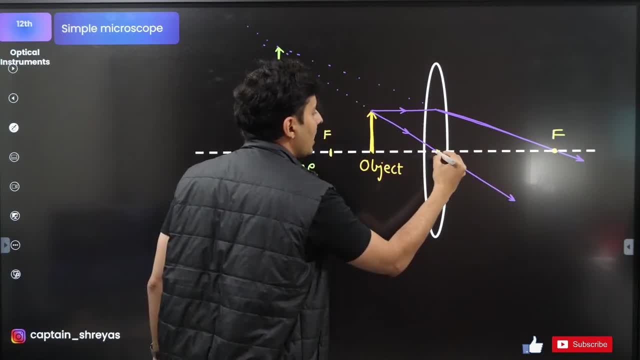 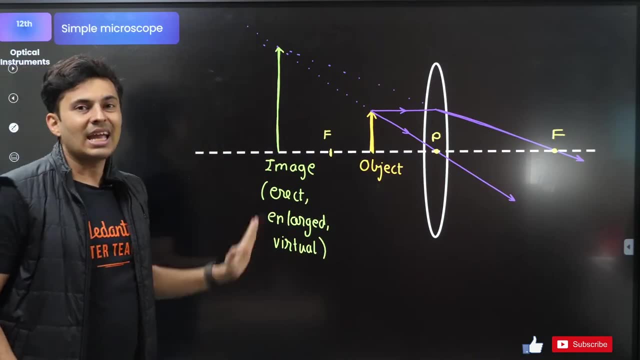 Then the object should be placed between the focal point and the pole, Between the focal point and the pole. Only then the image formed will be basically enlarged, Magnified, basically erect and virtual. If you place it at focus, then no image is formed. 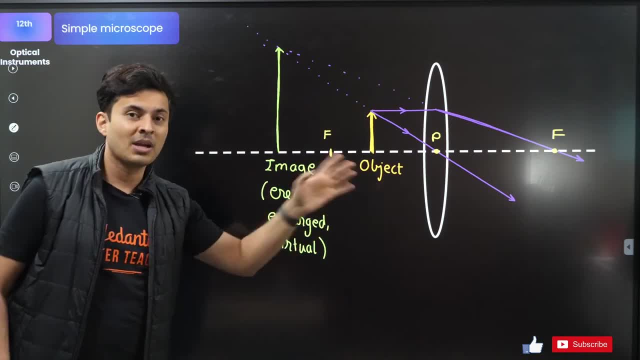 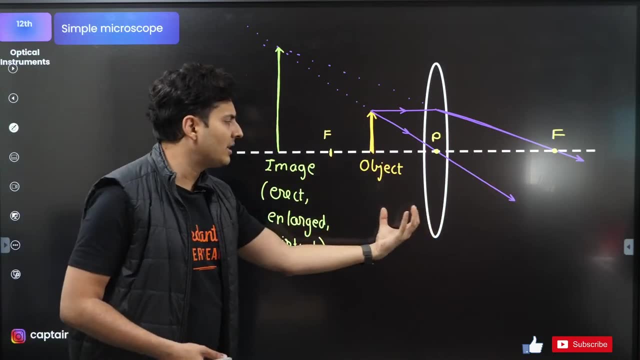 And if you place it beyond focus, then a real image is formed. I don't want a real image, I want a virtual image. So this is what happens Now: if you change the object's location or if you change the lens's position. 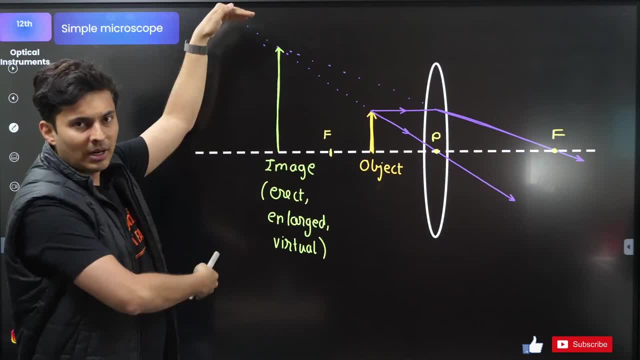 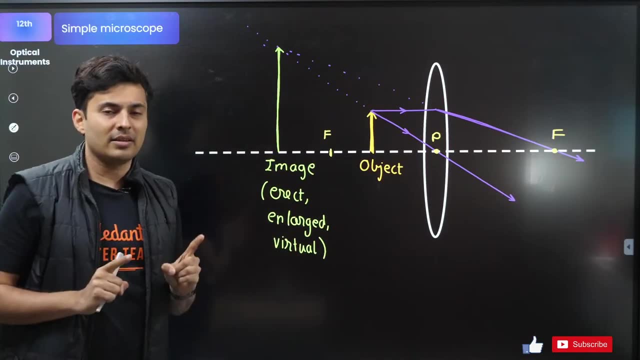 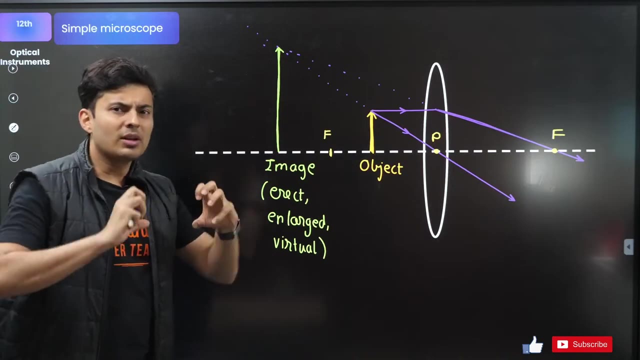 You will see the image size will keep on changing. It might become big or small, So you can change the magnifying power of it. Now there are two special cases, Two special cases For a simple microscope. The first case is when you strain your eye. 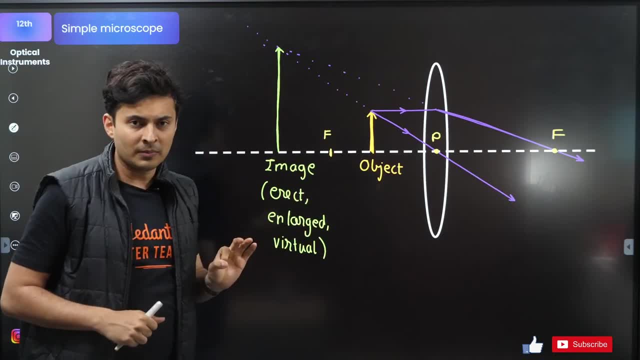 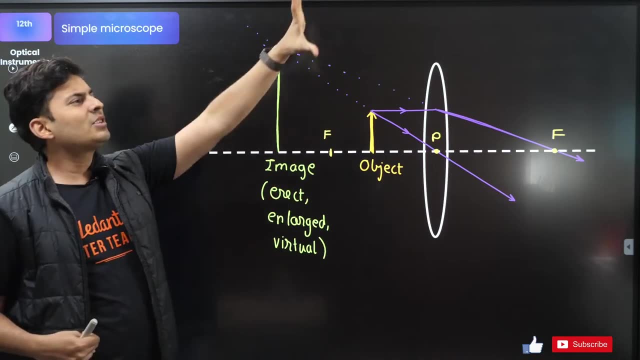 That means the image is formed at least distance of distinct vision. The image is formed at the least distance of distinct vision. And the second case: You are looking at that image, But the image is formed very far away, So your eye is relaxed. 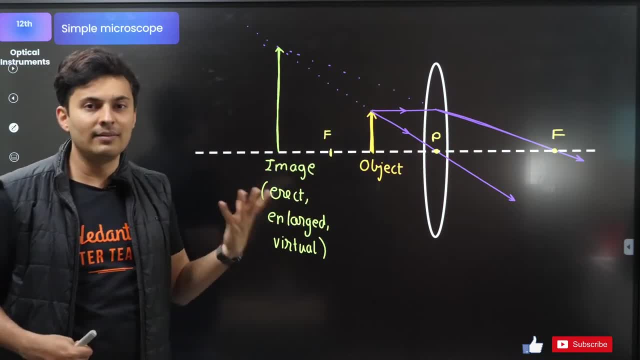 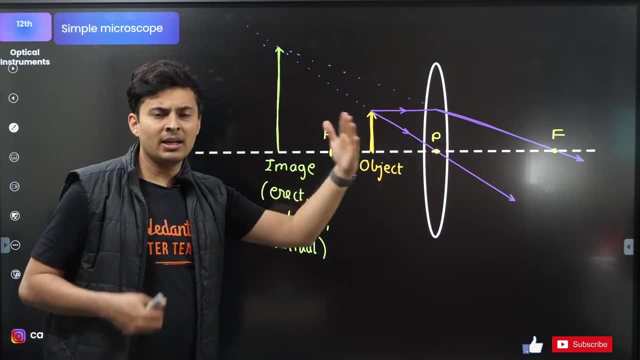 That means it is a normal situation, Normal vision. So two situations: You strain your eye By making the image Very close to the eye, That is, at 25 cm. That is the maximum limit. And the second case, which is normal vision. 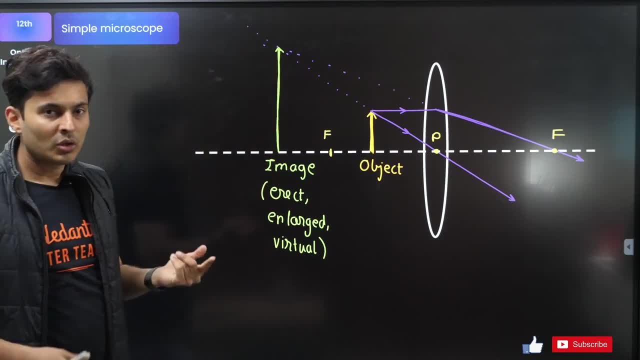 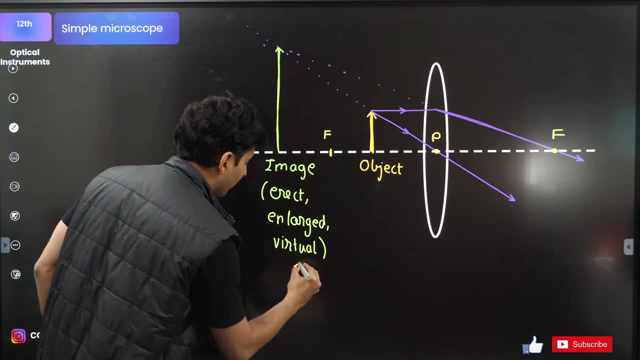 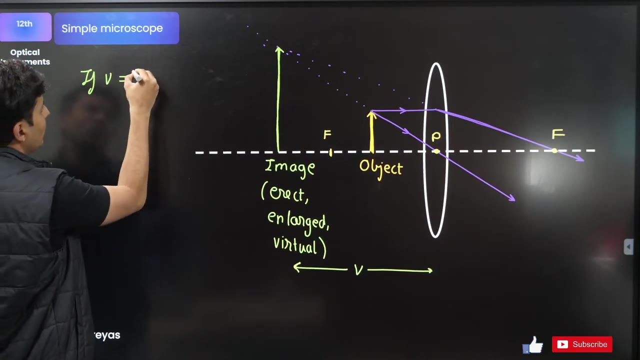 That is when it is really really far away. So here is what I will say. If this is the image distance, Wait a minute. If this is the image distance, If V is equal to capital D, Capital D is nothing but 25 cm. 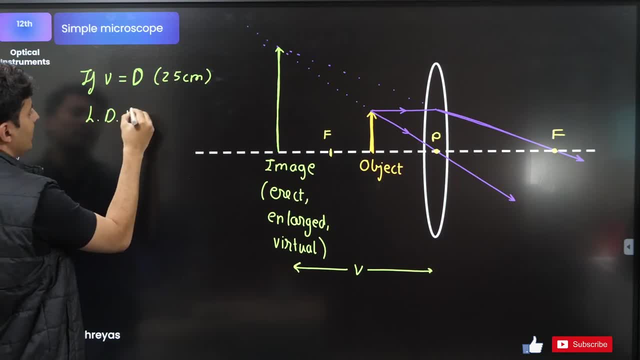 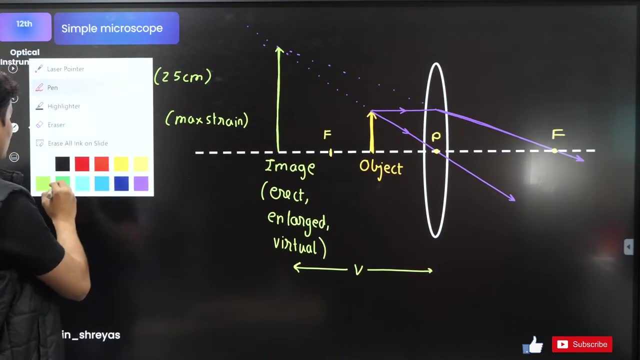 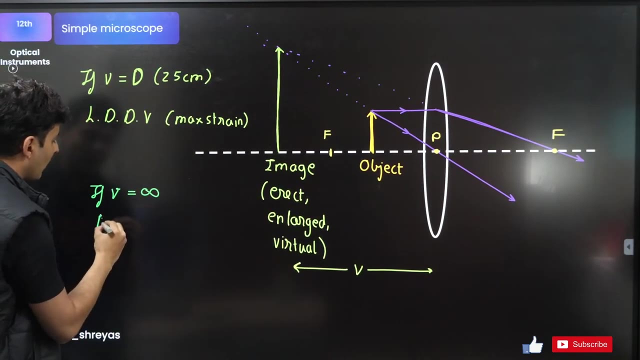 Then it is for the least distance of distinct vision. This is max strain on the eye. This is the maximum strain on the eye. The second situation: If the image distance is basically infinity, That means this is for normal vision. This is for normal vision. 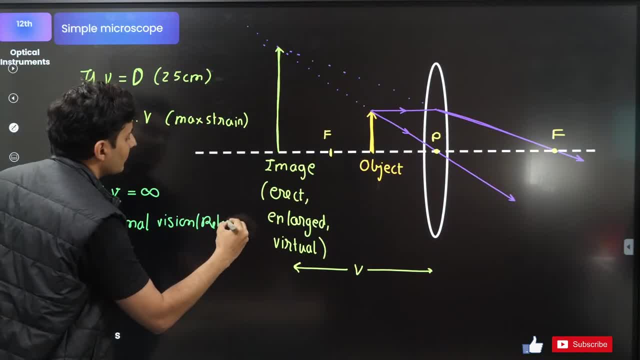 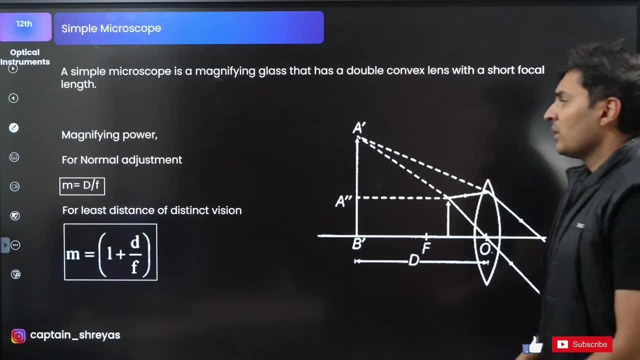 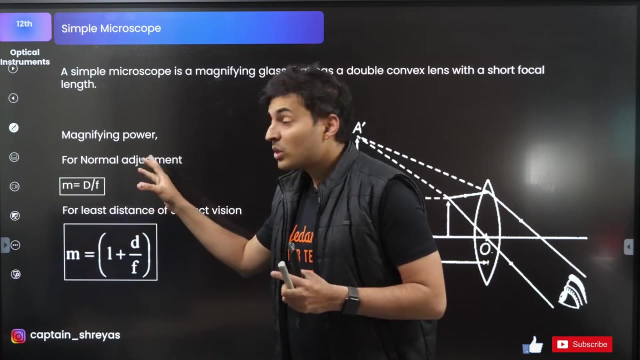 And it is basically relaxed condition. This is the relaxed condition, The magnifying power formula For both the situations you should remember. The first one is just D by F, Least distance of distinct vision by the focal length Which is for normal adjustment. 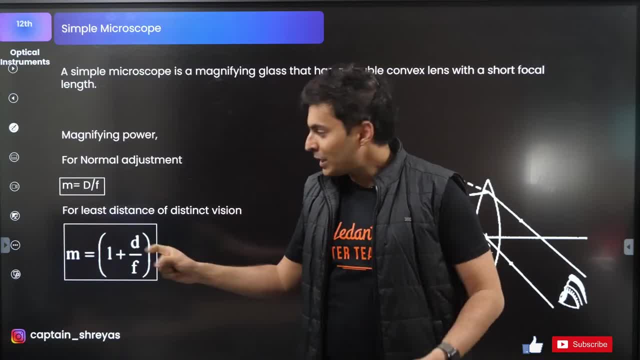 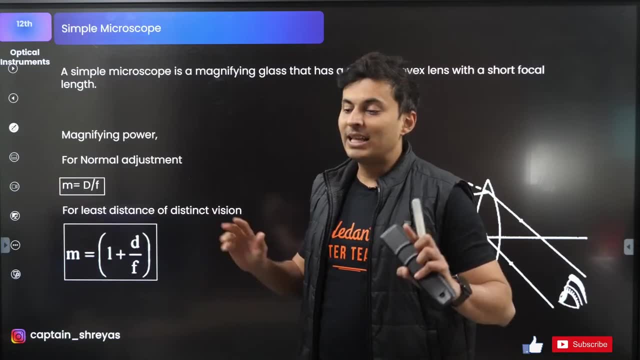 That means relaxed condition, But when you strain, The magnifying power increases by 1.. So 1 plus D by F. That is the change. That is the change, Tharshan, I told about LDDV before. I think you have joined the lecture little bit late. 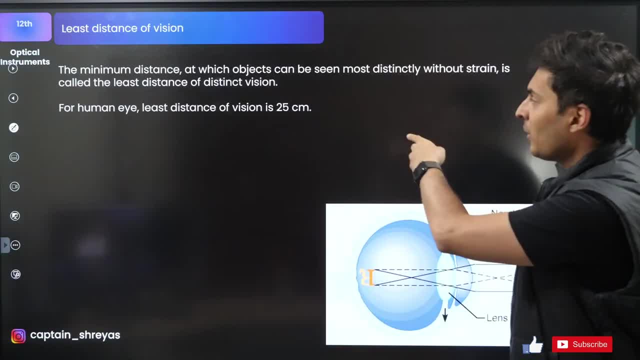 I have talked about what is least distance of distinct vision Right over here. Okay, 25 cm. So just rewind the session back, You will be able to get it. Okay. So I explained that. What is LDDV? 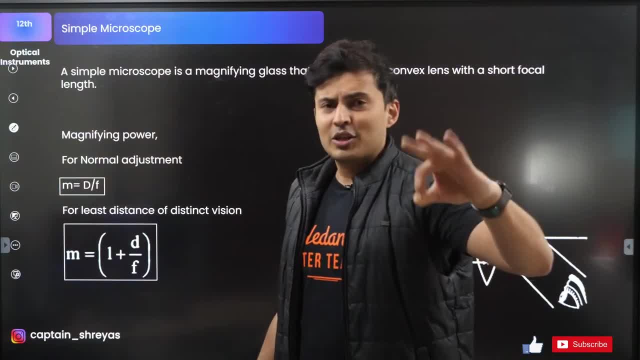 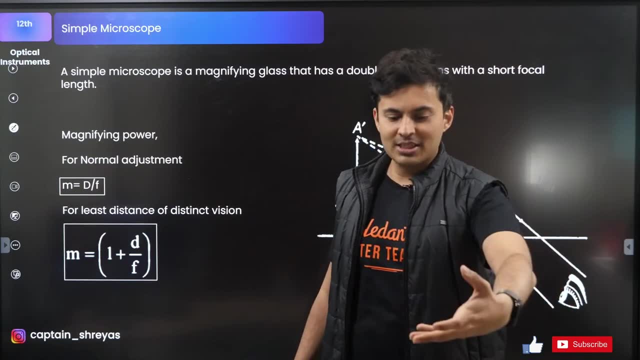 Okay, So when you relax, It is not that you will not get magnification, You will get, But it is less. It is D by F. But when you strain, Obviously, when you put in that effort, You are straining yourself. 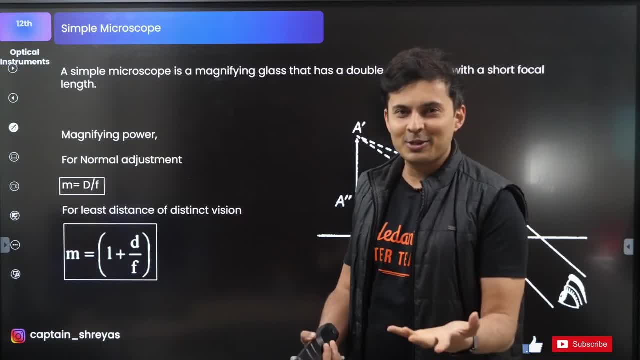 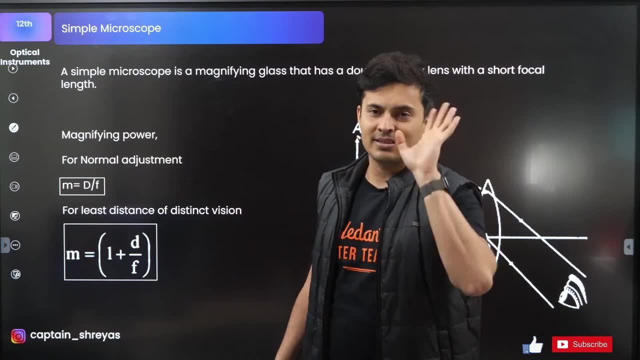 The outcome is also better, Just like in real life also. So when you work hard And you strive harder, Definitely the results are also better. So when you strain the eye, It is 1 plus D by F. Everybody with me on this. 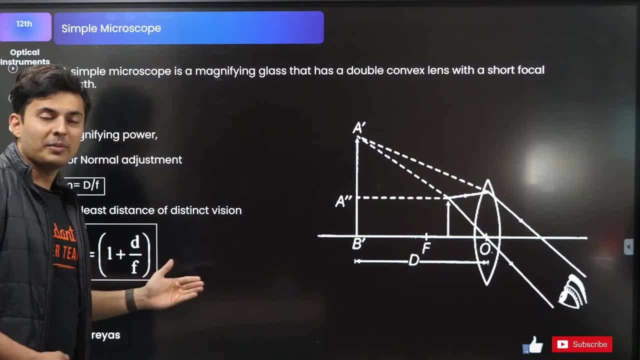 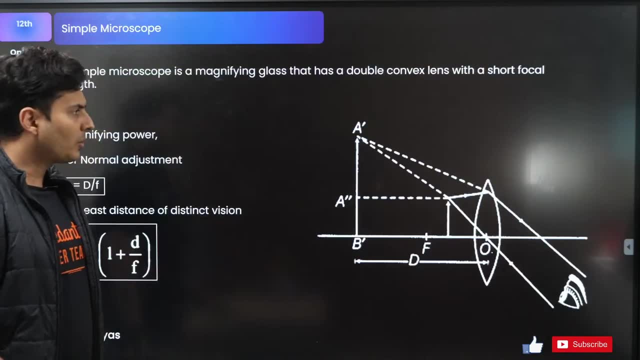 Clear. Okay, So these are the two main formulas for a simple microscope. You should know how to draw the ray diagram. You should also know the definition of what is magnifying power. So probably we can solve some questions based on this. 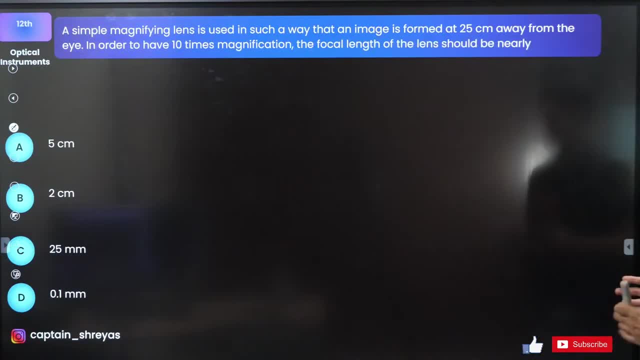 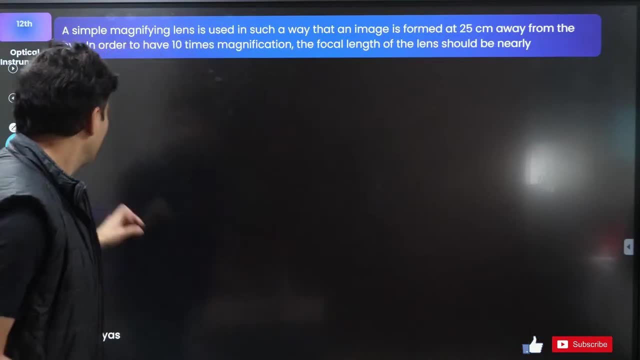 Okay, A simple magnifying lens is used in such a way that the image formed is at 25 cm from the eye In order to have 10 times magnification. The focal length of the lens should be how much? Okay, Let's try to understand the question, what it means. 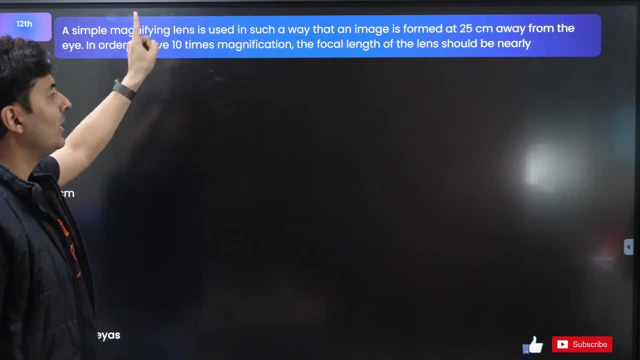 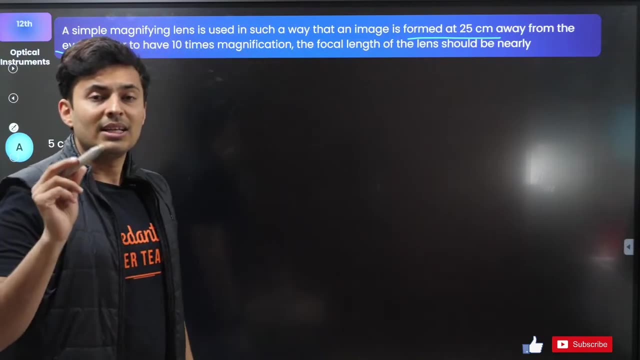 The simple magnifying glass. The simple magnifying glass is used in such a way that the image is formed 25 cm away from the eye. So quickly think and tell me: Is this the case of normal vision Or is this the case of least distance of distinct vision? 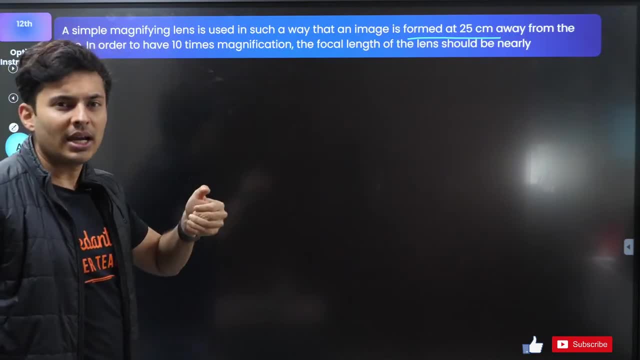 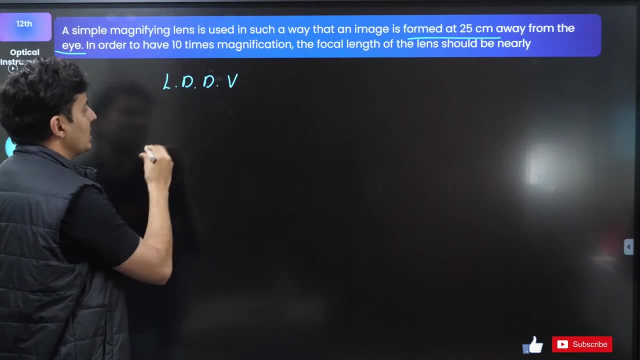 Because the image is formed. 25 cm, That means very close to the eye. So this is the case of least distance of distinct vision. Yes, And when there is least distance of distinct vision, The magnifying power formula is 1 plus D by F. 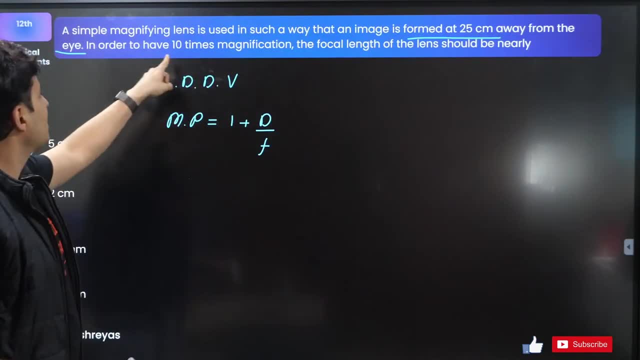 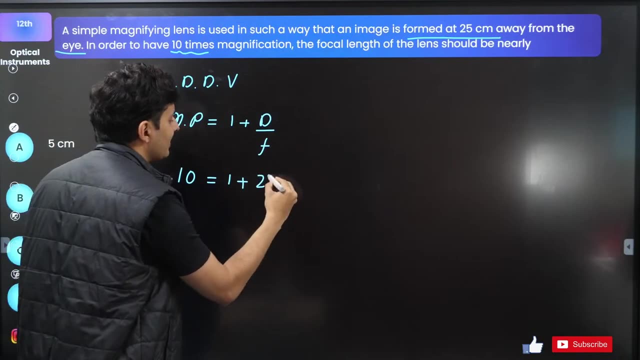 Right Now, what is the magnifying power? It is clearly mentioned 10 times. 10 times is the magnifying power, So magnifying power is 10.. Least distance of distinct vision is 25 cm by focal length. 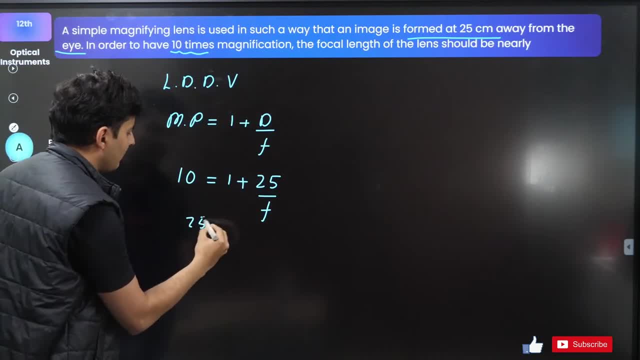 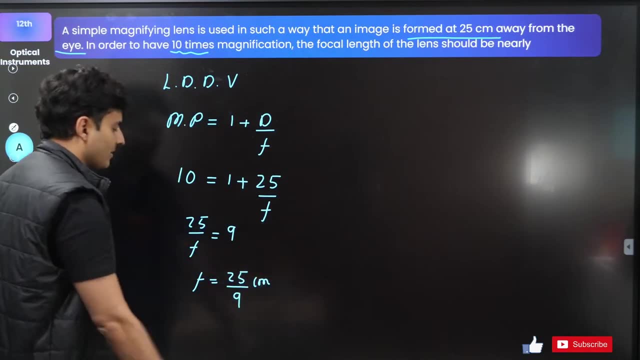 Great. So now shift the term So you will get: 25 by F is basically 9.. So F is basically 25 by 9 cm. Now 25 by 9 cm. I can also write it in mm. 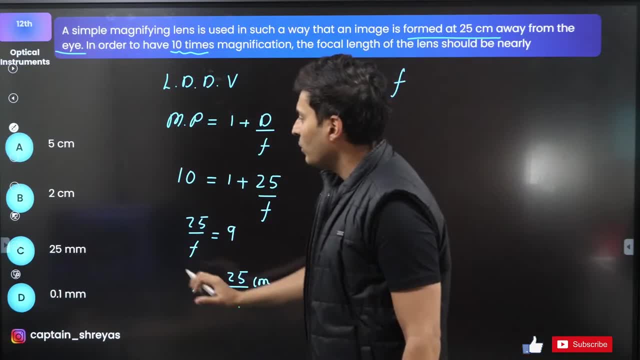 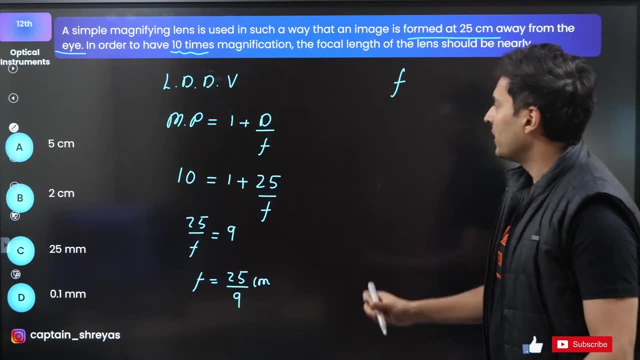 Because Some of the answers are in mm. I don't see 25 by 9 anywhere in option A or B. It is 2 and 5.. Obviously it is not them. Either it will be C or D, So think about it. 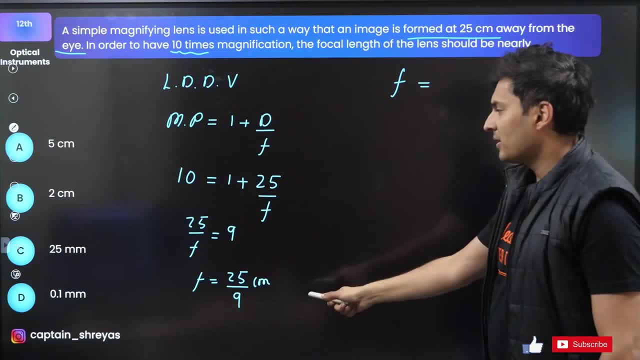 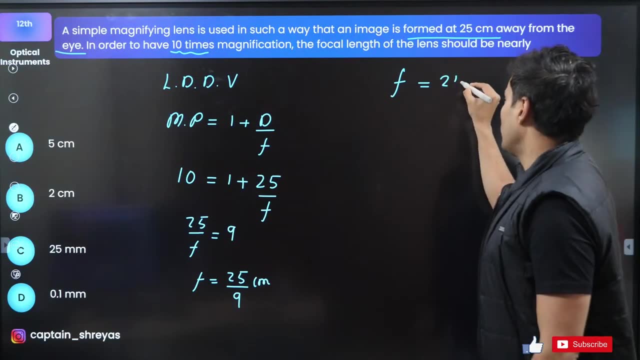 What I can do over here. What I can do over here, Because, Because this is in cm, To convert it into mm, What I need to do Multiply by 10.. So this will be nothing but 250 by 9 mm. 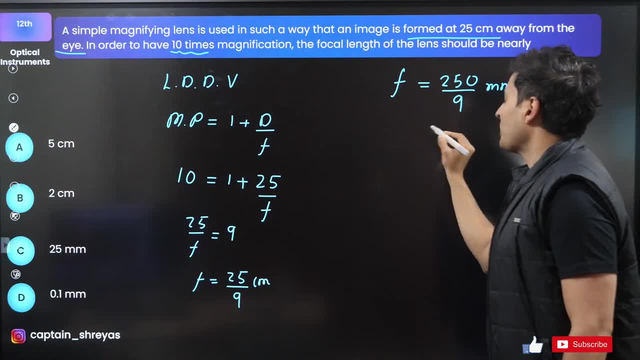 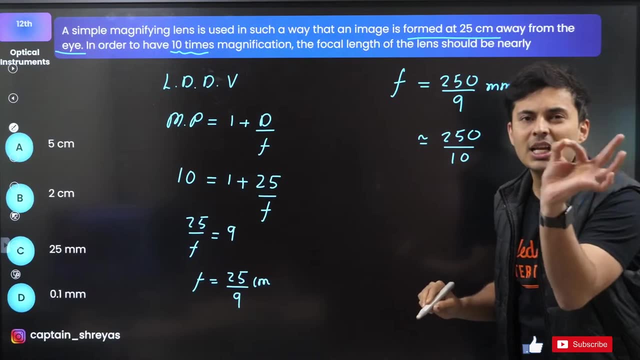 Everyone with me Now: 250 by 9.. 250 by 9.. Isn't it almost same as 250 by 10?? 9 and 10 are very close. 9 and 10 are very close numbers, So instead of 9, I can write it as 10 mm. 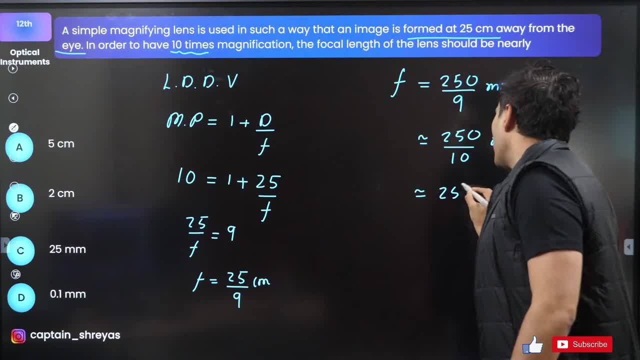 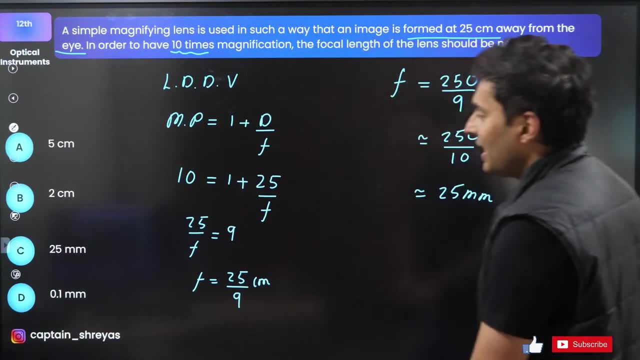 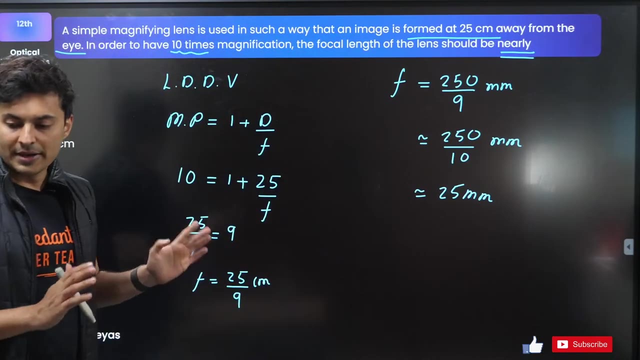 00 cancels. So what will you get? Approximately 25 mm Nearly. The question said nearly Approximately 25 mm, Hence the correct answer will be C. Everybody got this. Everybody got this Understood Clear. 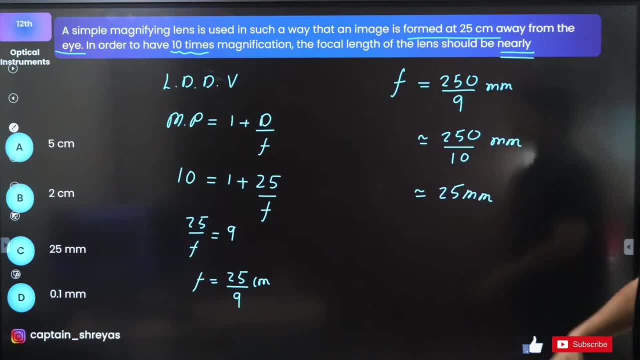 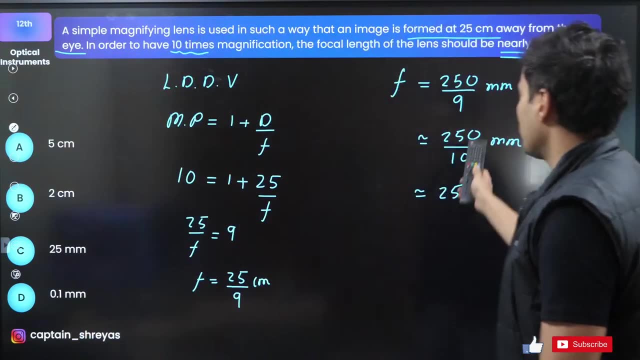 Let me know in the chat box by thumbs up, Then we will move on to the next question. So simple microscope question. The magnifying power was given, Focal length was asked, But you had to convert it into mm, So that was the tricky part. 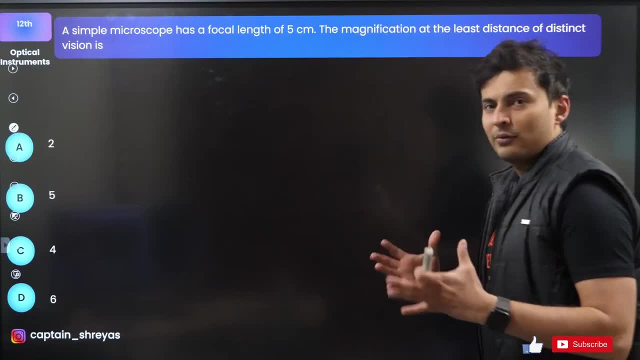 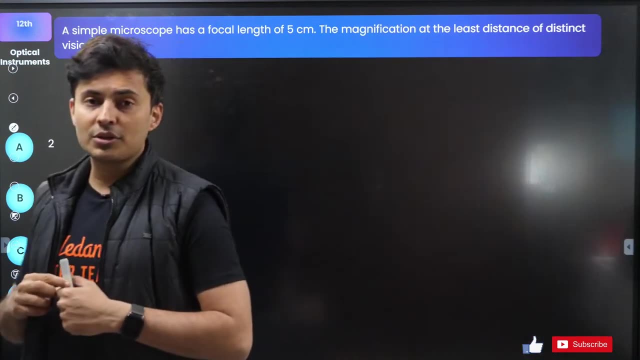 Let's do one more question. If there is a microscope having focal length of 5 cm, Magnification at least distance is how much? Let's try to do this question. Question says: what is the magnification at least distance of distinct vision? 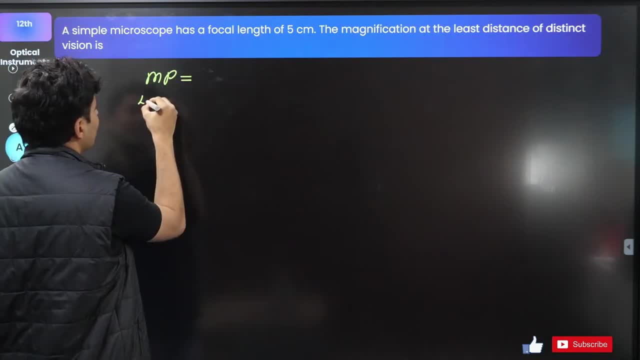 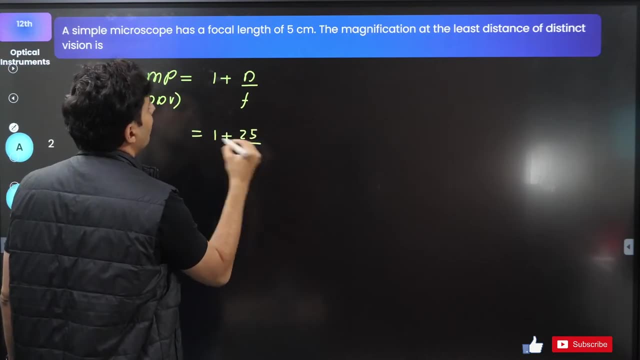 The magnifying power, at least distance of distinct vision, is given by 1 plus d, by f, So d is 25.. Focal length is 5.. 25 by 5 is 5. So this will be basically 6.. 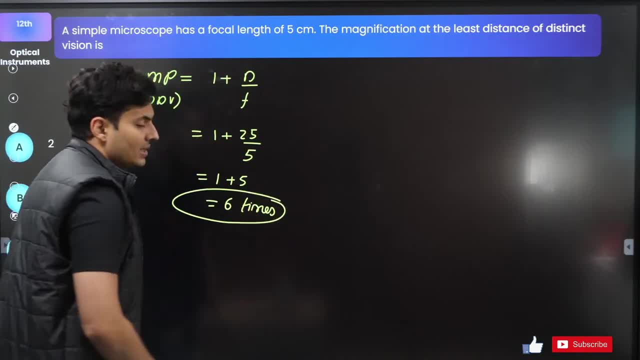 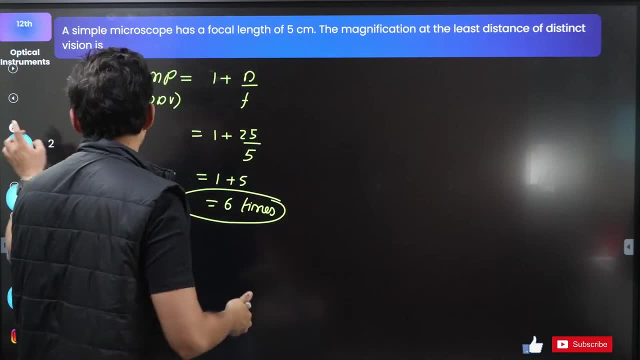 So 6 times is the answer. Where is such an option? Where is such an option? Yes, option D: Perfecto, Perfecto. If the question said normal vision. If the question said for normal vision, So for normal vision. 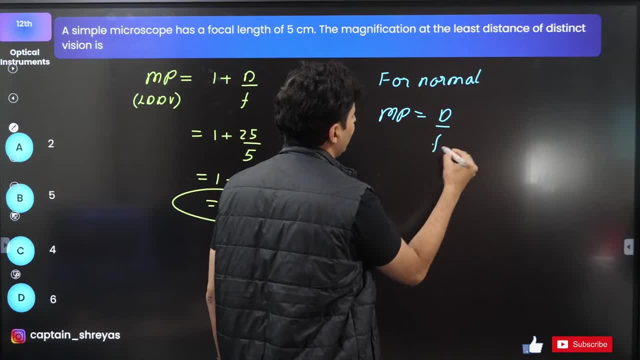 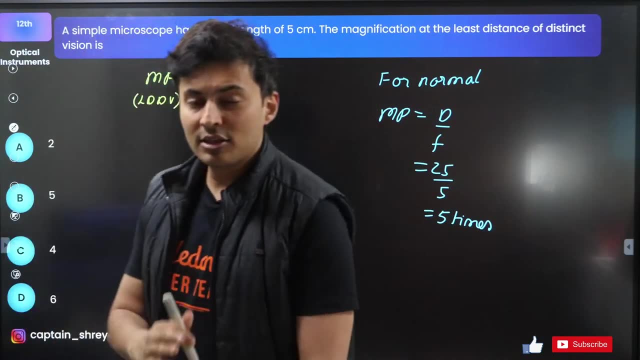 Then the magnifying power will be just d by f, So it will be just 25 by 5. That means it will be just 5 times. So read the question Whether it is normal vision or whether it is least. distance of distinct vision. 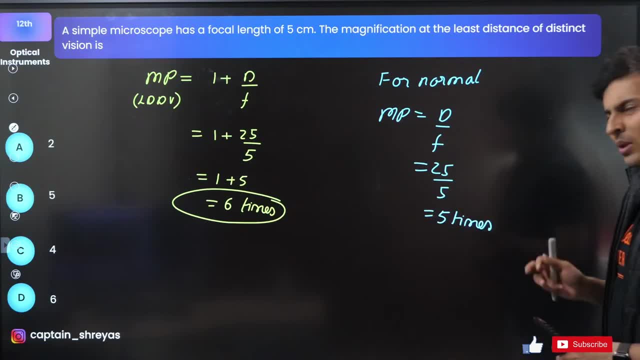 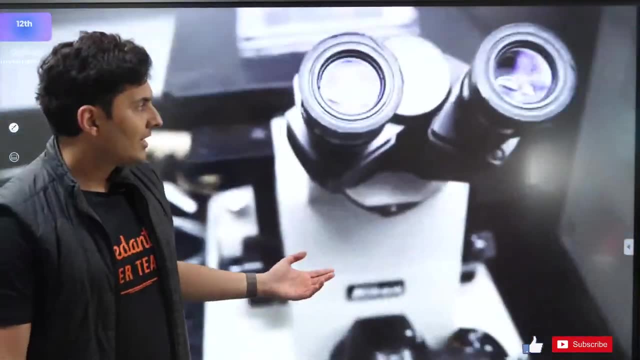 So, accordingly, you are going to use the suitable formula. Cool. So that's how simple the questions are. from simple microscope, Let's go on. Let's go on to the compound microscope Shakufanta's real and virtual image. Please watch my yesterday's class. 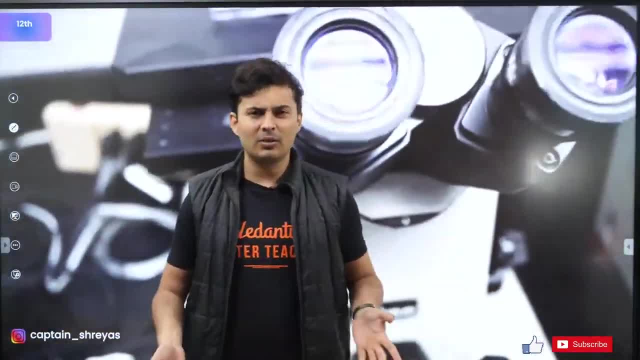 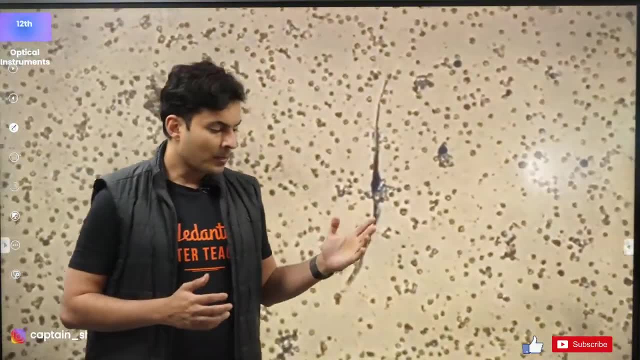 I have explained in detail what is the meaning of real and virtual image in the starting part of the class May be in the first 10 minutes or 15 minutes only I have explained it. Watch the yesterday's class Now. imagine I want to see things which are even smaller. 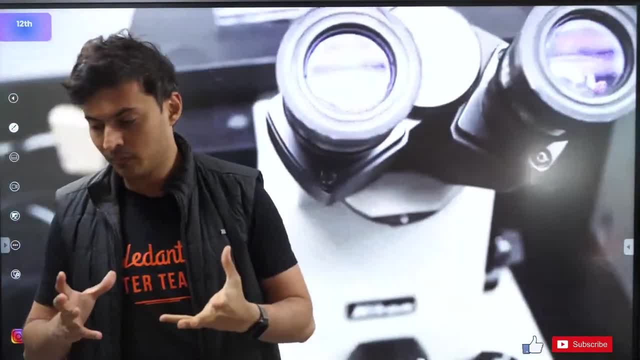 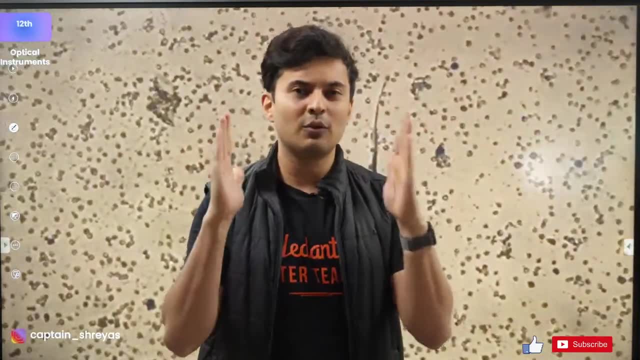 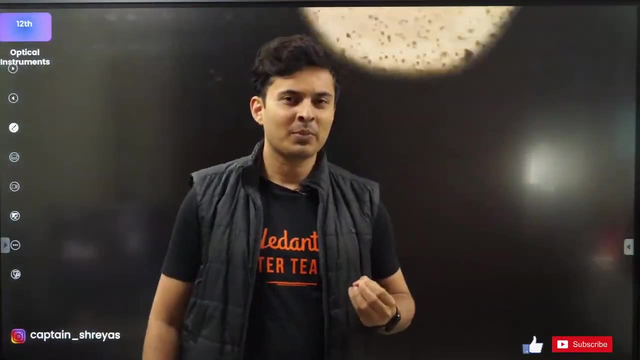 Which even a simple magnifying glass cannot zoom into. So for that I use a combination of two lenses. Using this combination of two lenses, I can magnify even further And I can see even a small bacteria virus as well, Which is what you see in labs like this. 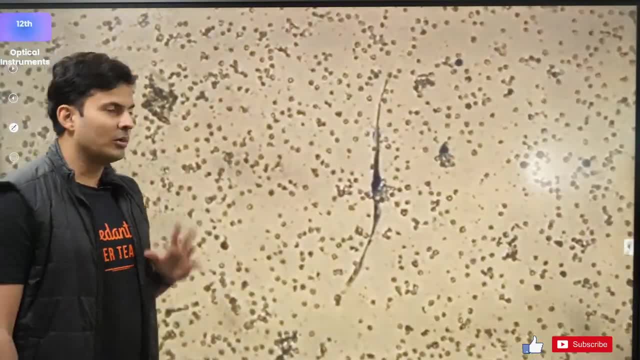 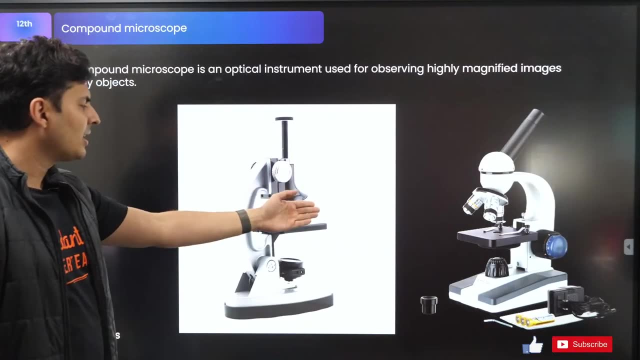 Like a cell, a virus or a fungus or some small object. Now the idea behind a compound microscope, or just your microscope, which you see in your day to day life or may be in a lab, Is You have two lenses, Like I told you. 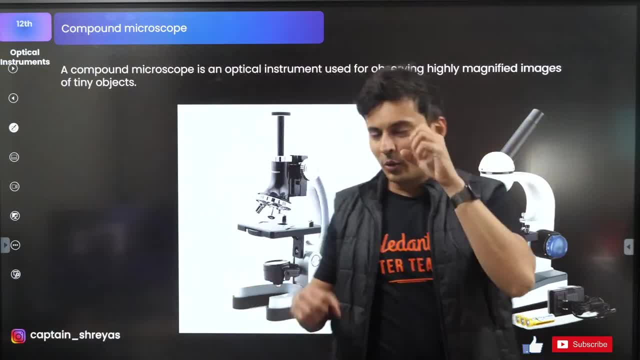 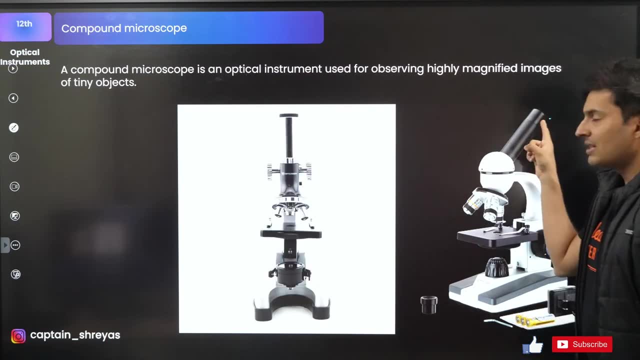 The lens through which you see. You put your eye over here, Okay, You put your eye over here And you see That lens is called as the eyepiece. What is this lens called Eyepiece? The lens which is close to the object. 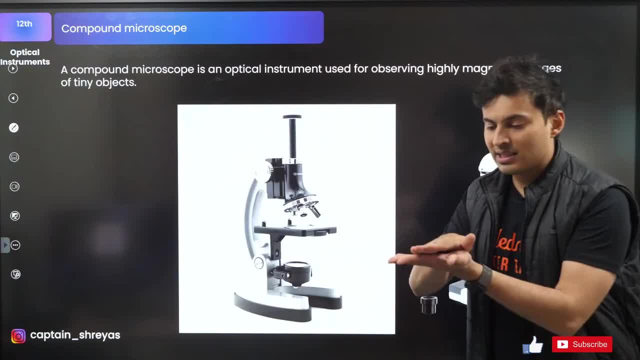 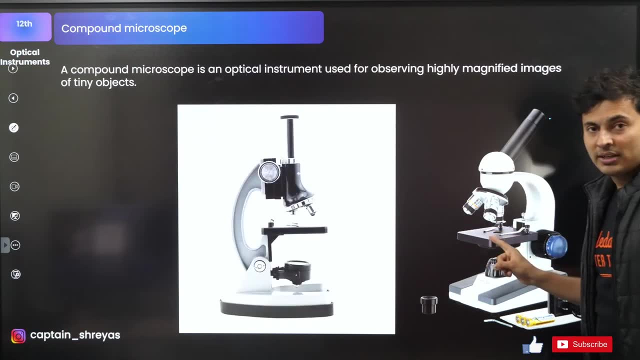 You can see the lens over here. You will have a culture or a slide or some object which you want to magnify. zoom into The lens which is close to the object. What will it be called Objective? So this is objective. 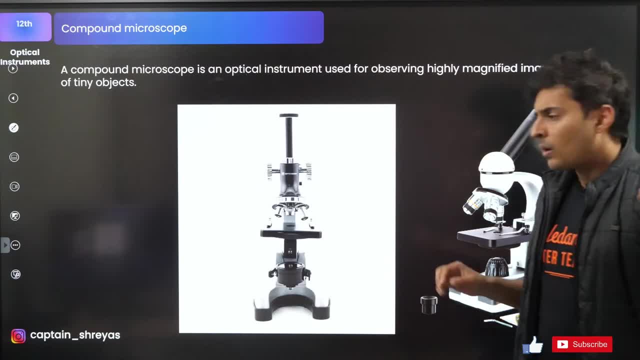 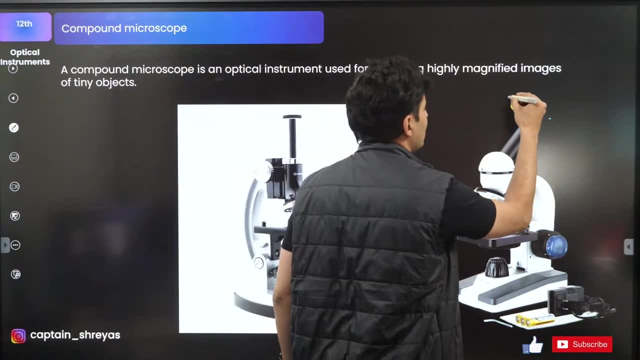 This is the eyepiece. Everybody with me. Objective and eyepiece. Now, Now Imagine. Imagine Just one second. Let me just put it over here. This is the eyepiece. This is basically the objective lens. 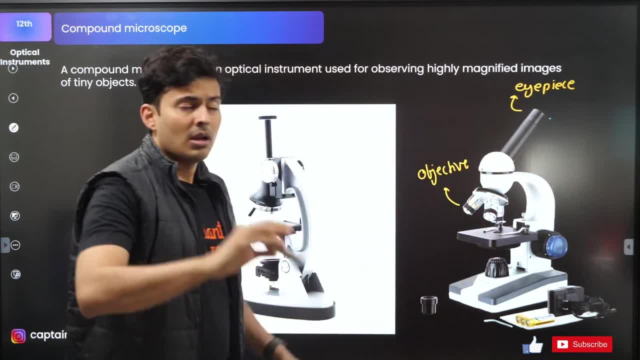 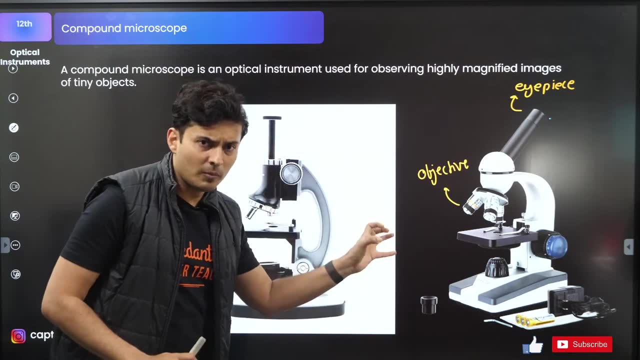 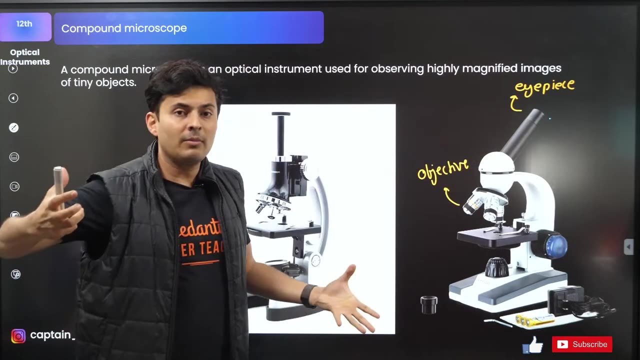 Objective lens. Imagine: The only job of an objective lens Is to make an image Which is big, Is to make an image Which is big. That big image Is further magnified by this lens, So two times the magnification occurs. 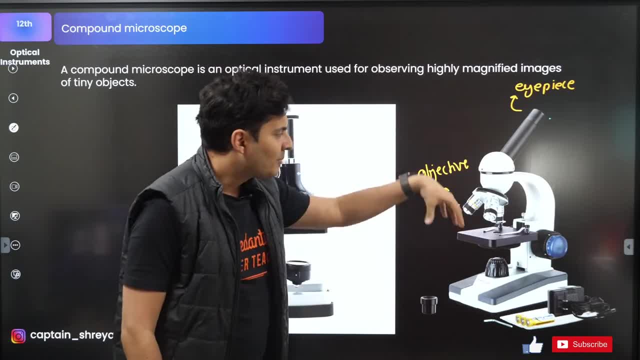 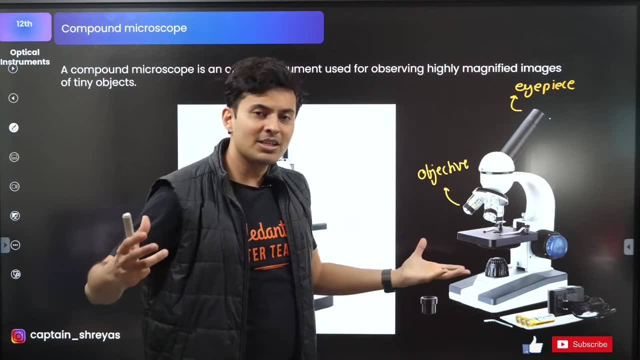 Yes or no Agreed Objective Makes a big image Somewhere here Inside the lens, I am sorry, Inside the microscope- Makes a big image. That image is further zoomed by the other lens, Which is the eyepiece lens. 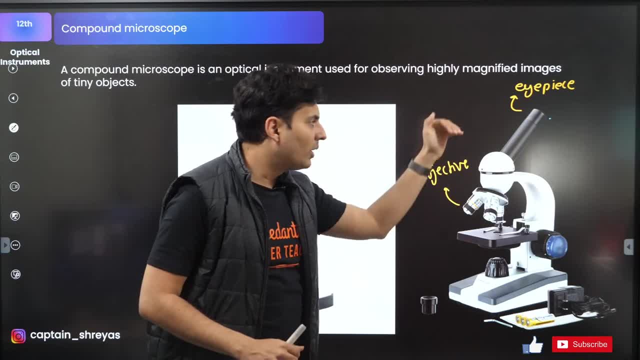 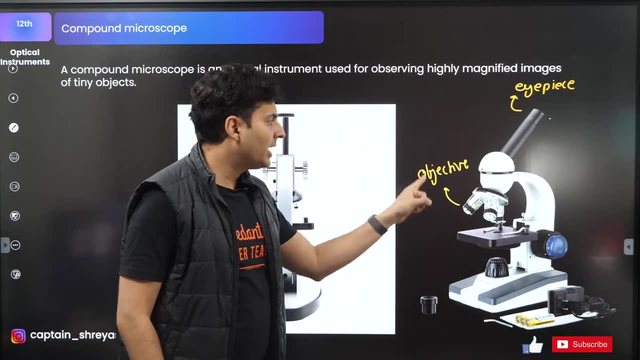 I will tell you what: Because you want to make an intermediate image. That also means The image of the objective. The image of the objective Is the object of the eyepiece. Convince yourself, Sir, even for an image at an infinite position. 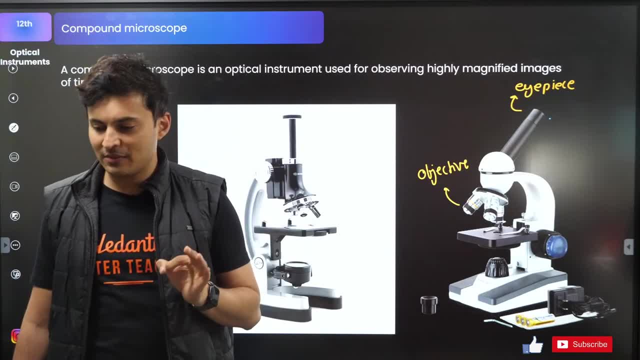 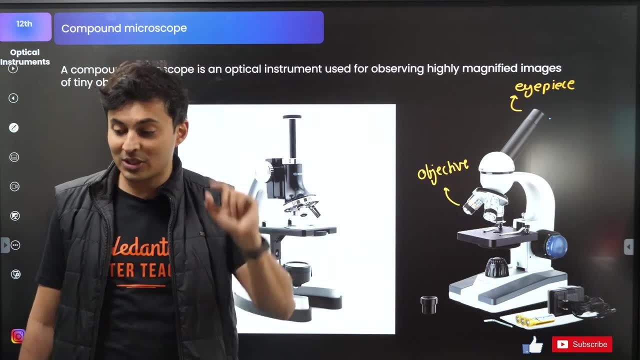 We can use d by f, Exactly, Ashrita, When the image is formed at infinite position. that is when you use d by f, Because that is normal vision. When the image formed at infinity, ie eyes are focusing on infinity, the eyes position. 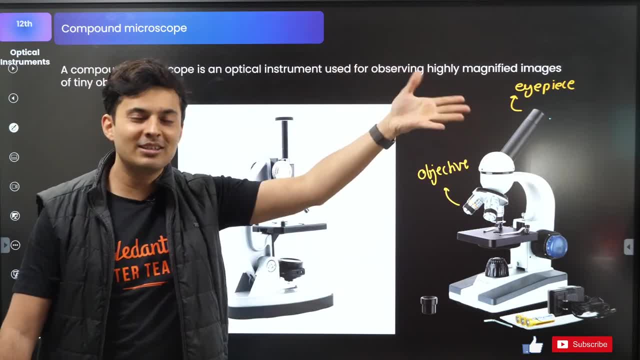 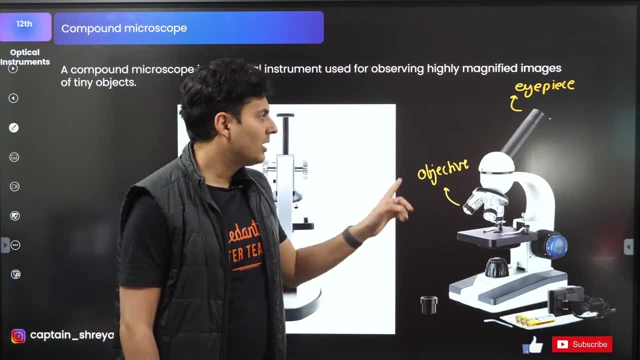 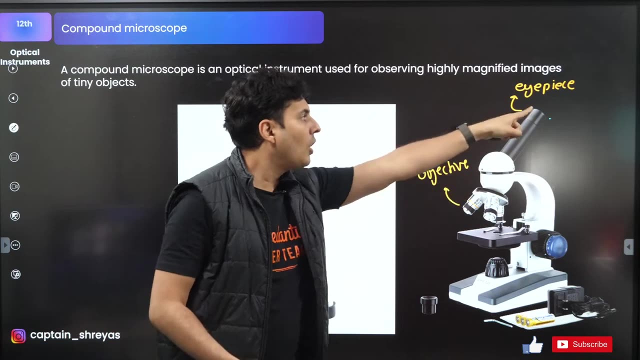 will change on infinity. they are completely relaxed, which is itself called as relaxed or normal vision. so that's when you use d-bif for a simple microscope. actually, though, is that okay? okay, fine. now coming back to this, so the image of this objective lens becomes the object for the eyepiece lens. perfect, everybody. 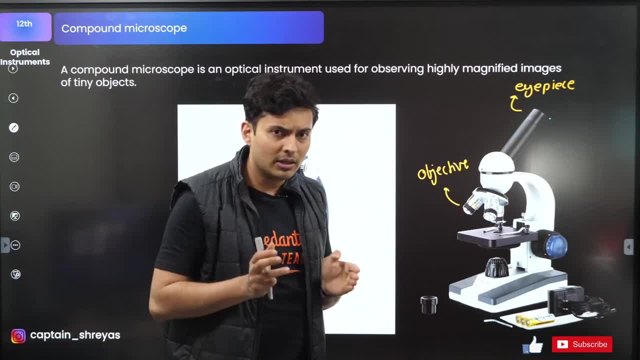 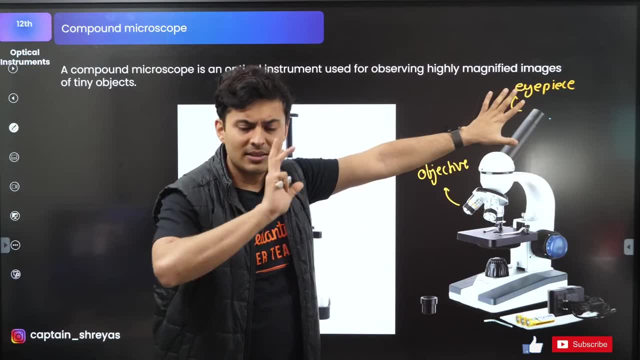 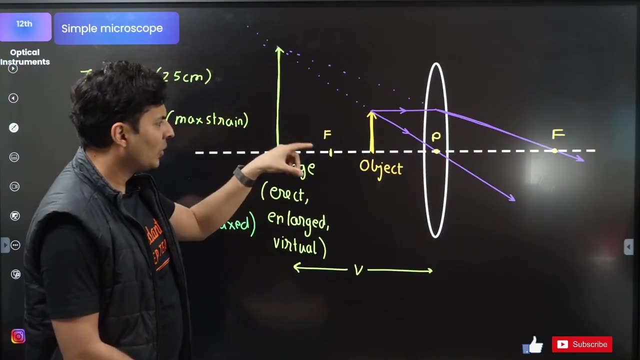 understood this point. so here, in case of microscope or even, you will see, in telescope, the eyepiece actually acts like a simple microscope. the one which is shown over here: the eyepiece acts like a simple microscope, so it will basically zoom into that object, making an even larger image. but this object is 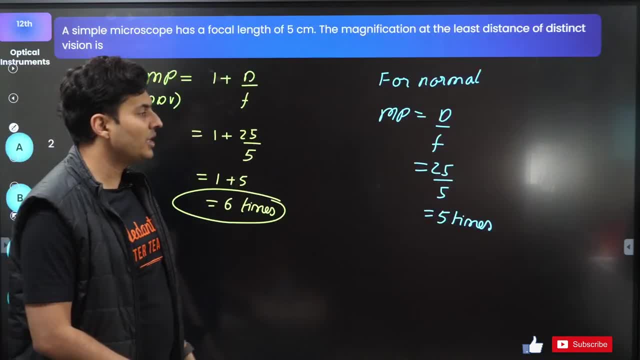 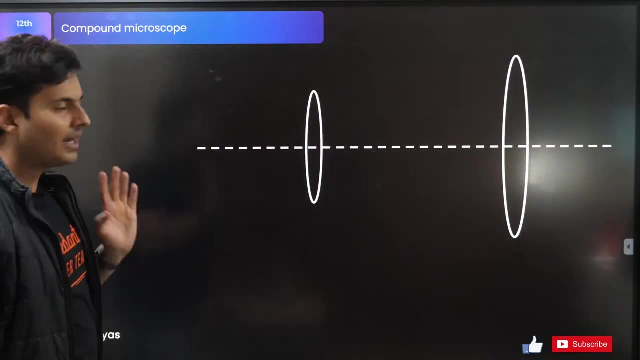 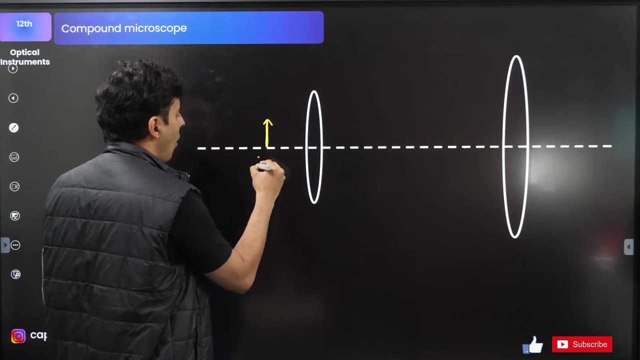 actually the image formed. this object is actually the image formed by this particular objective. so there is an intermediate image which is formed. so how does the ray diagram look like? observe it carefully. okay, I'm just going to draw it. I'm first going to draw all the objects and images, because that will be easy, then draw the ray diagram. 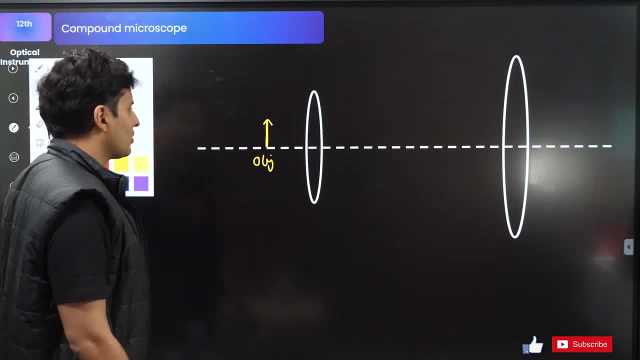 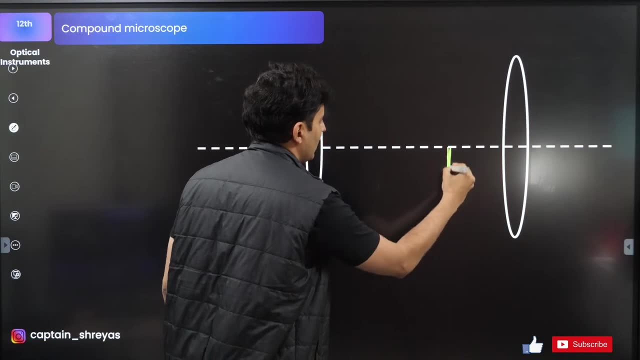 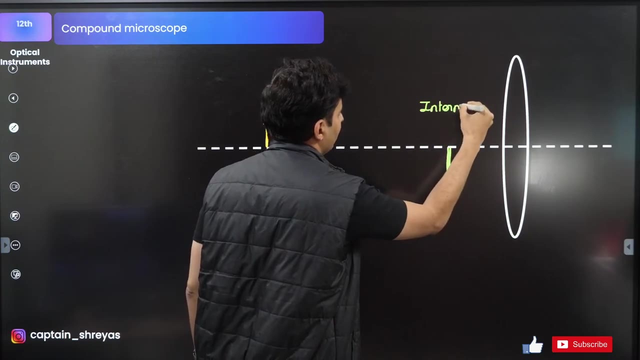 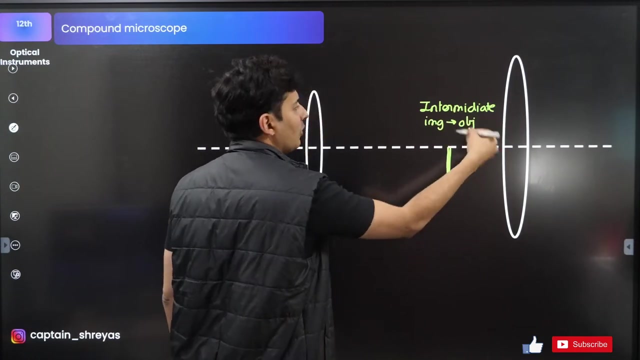 usually that works out well, even in your board exams. that's what you can do. so this is your object. the image formed is basically inverted. it's inverted, it's a real image which is formed. this is an intermediate image, this is an inter mediate image, which then becomes the object for the next lens. this lens over here is: 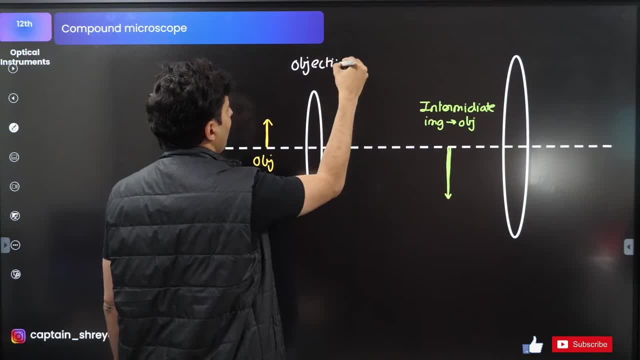 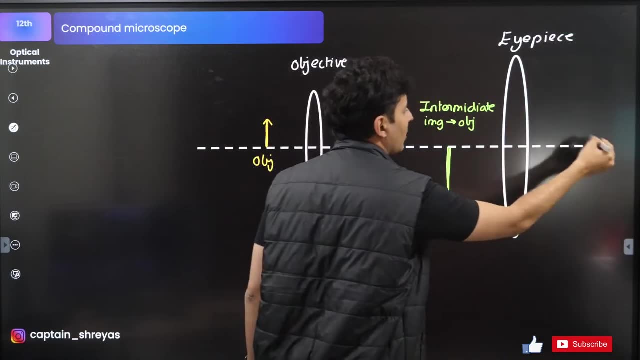 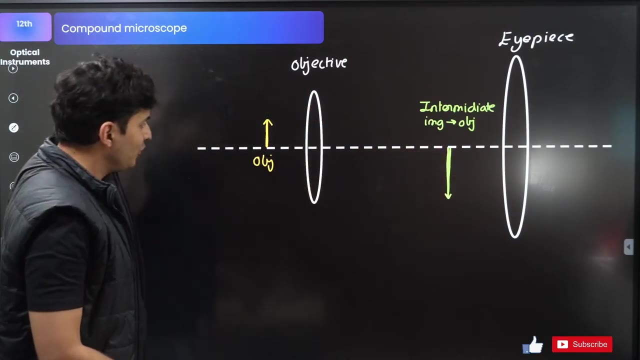 basically your objective and this lens over here is basically your eyepiece. this is basically your eyepiece. that's where your human eye will be okay from that side. now this image becomes the object for this lens and it is further zoomed into and probably you might get at the final image. I don't know the final image. 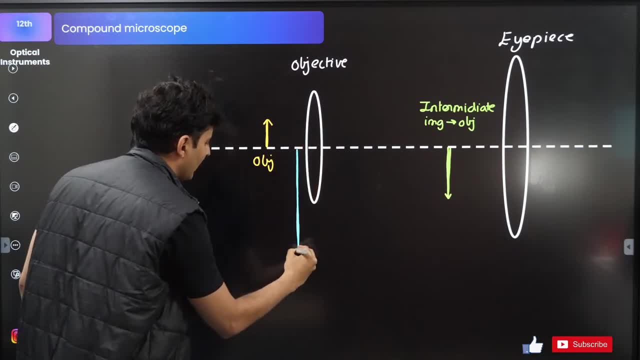 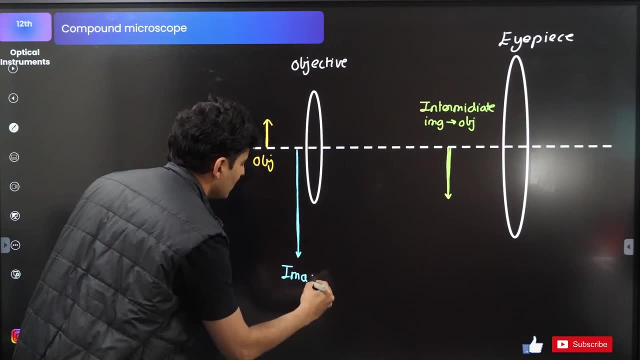 maybe over here just giving you a random diagram. guys, don't take it literally. it can form here here. so different possibilities are there. this is your final image, which is formed. now let me show you the ray diagrams how it will look like. so basically, it will look something like this: 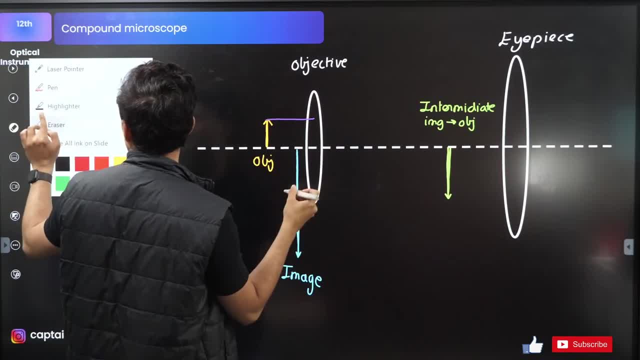 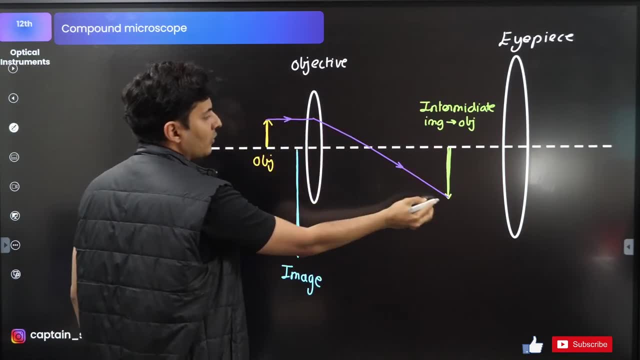 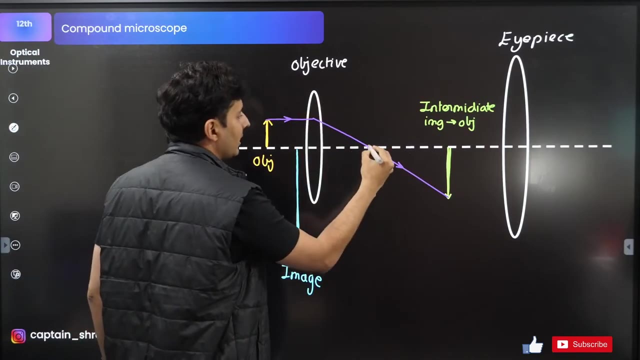 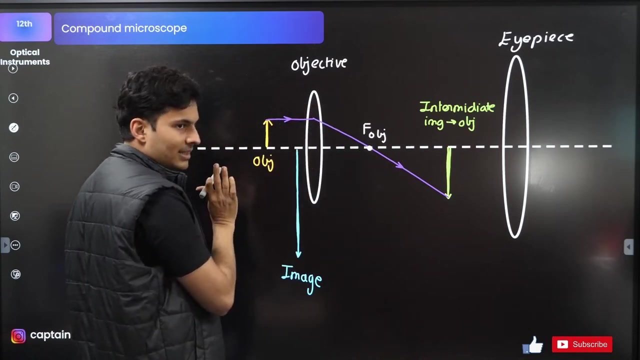 just one sec. so this is how the rays will go to form the image from the object. so it's passing through the focal point. so this focal point is of the objective, so i'm just going to call it as the focal length of the objective. this is the focal point of the objective lens. keep that in mind. 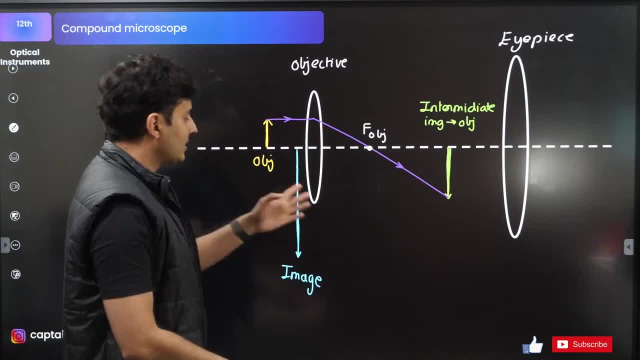 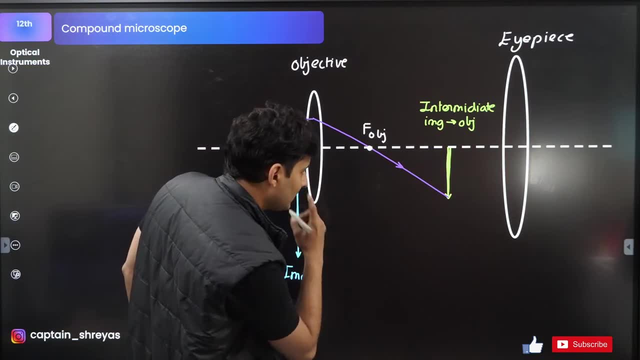 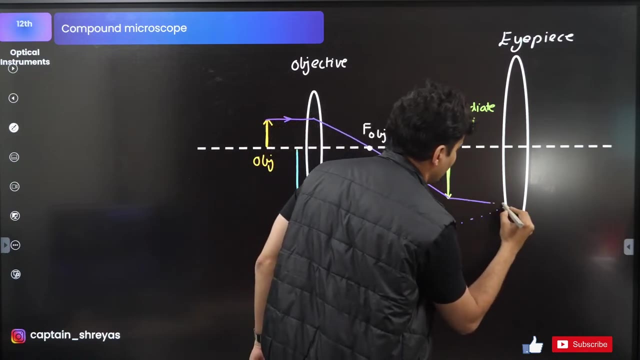 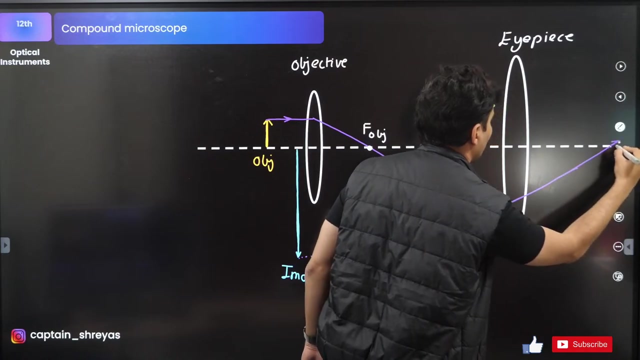 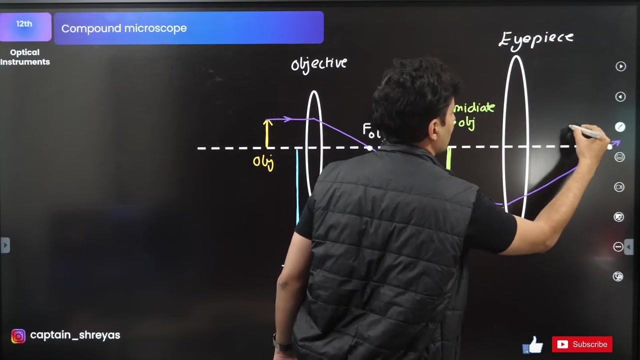 f? o also you can call it. and for the next one, what i can do is probably: this is the focal point of the objective lens. keep that in mind. okay, little bit tricky, but i will try this out. this is a virtual one. okay, one second. we'll go like this and this will be your focal length. just once again, this will be your focal. 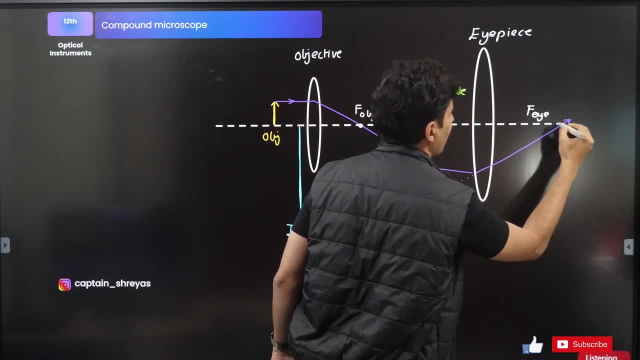 length of the eyepiece. focal point of the eyepiece. oh my god, okay, so this is the focal point of the objective lens. keep that in mind. okay, i think now it's fine. so this is how the ray diagram looks like. see, if you guys have 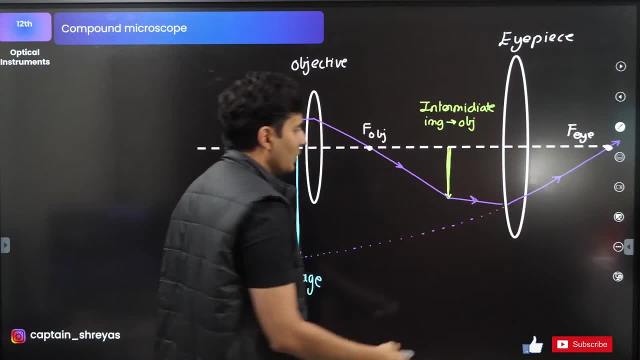 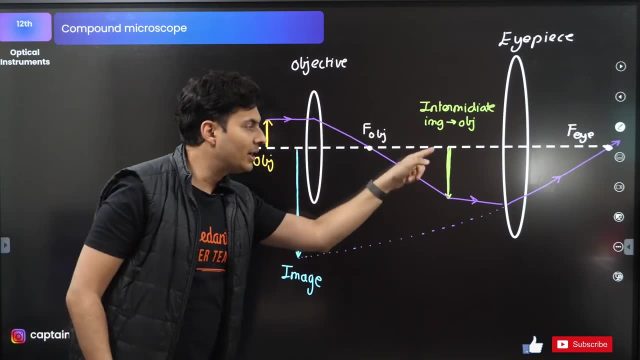 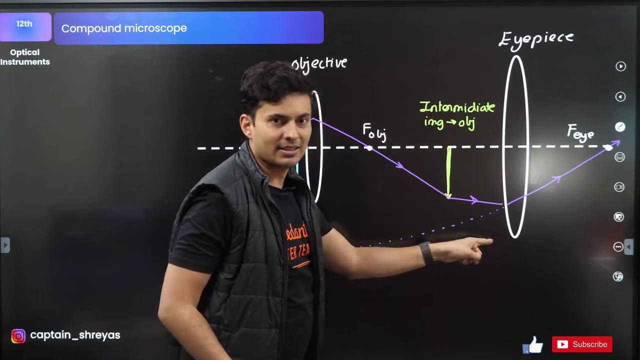 understood this? okay, i'll just explain this to you. this object, this object placed in front of the objective, makes a real inverted image. okay, the rays go like that and form an inverted image. then this image becomes the object for this lens. it is placed in such a way that this lens behaves. 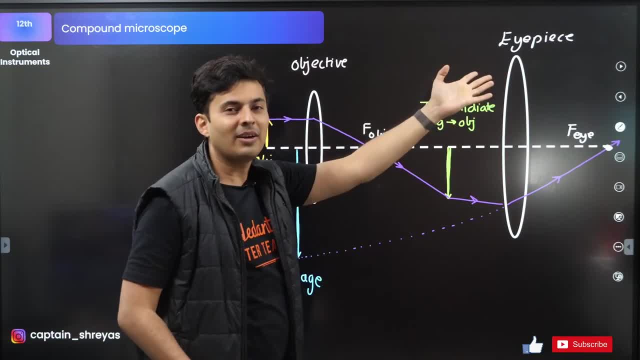 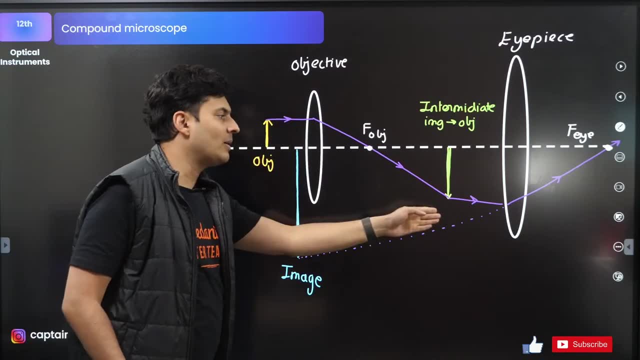 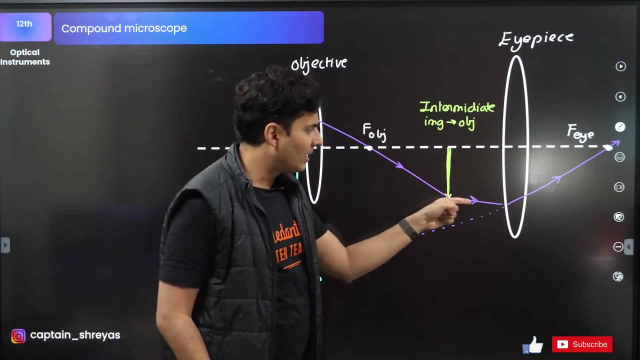 like a simple microscope: your magnifying glass. how does the magnifying glass behave? if the object is between the focus and the pole, you will see a virtual enlarged image behind the, behind the lens. so you will see a virtual image behind the lens on this side. so i've just taken one ray parallel to the principal axis. after passing it becomes: 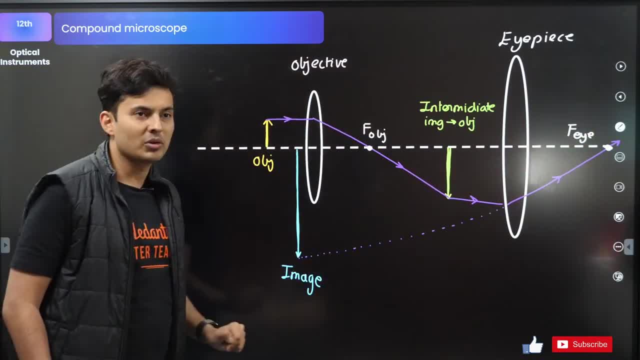 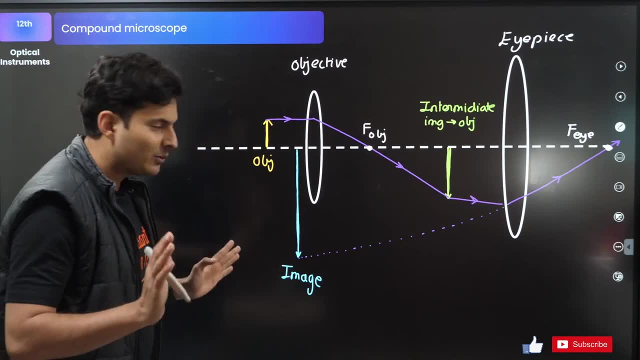 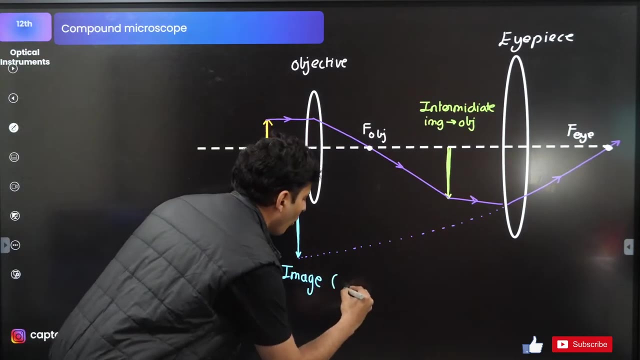 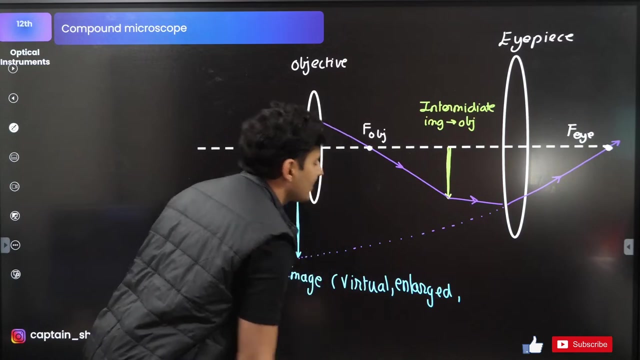 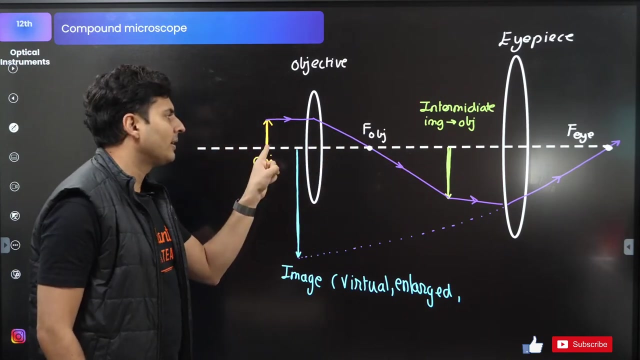 it passes through the focus, so if you extend it behind, it goes over here. see if this is clear. see if this is clear. hello joy, hello puja. okay, everyone with me on this. σου, the person who accepted it is my clone, since it was final. as you can see, it will have the same size as each object, except for the frame. now the 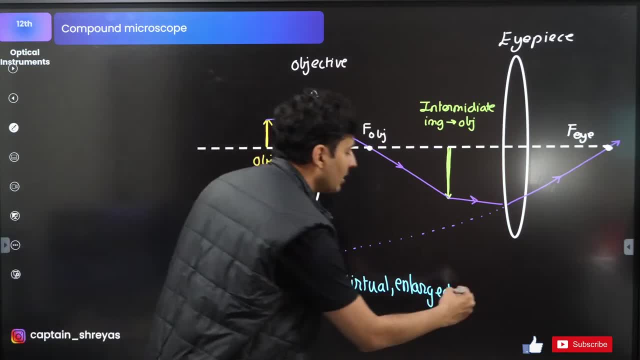 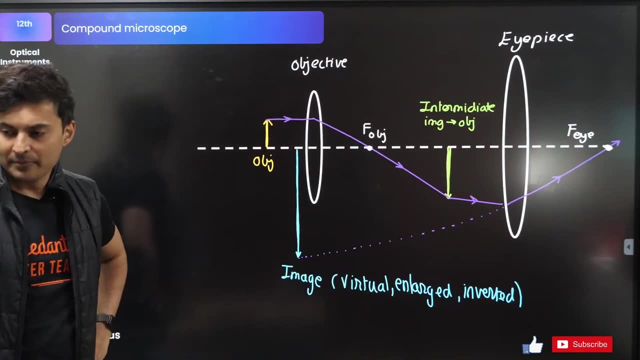 point is, if the final image goes on the second axis, where the target is less than or equal to once a second, the image of that object is going to be inverted as the final image, aujourd going to be inverted. everyone with me clear, oh, understood, perfect. so this is how the final image 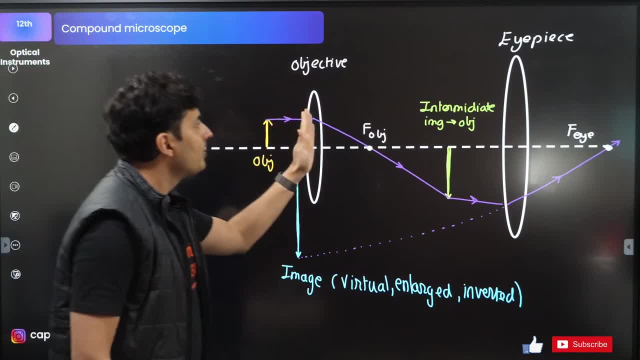 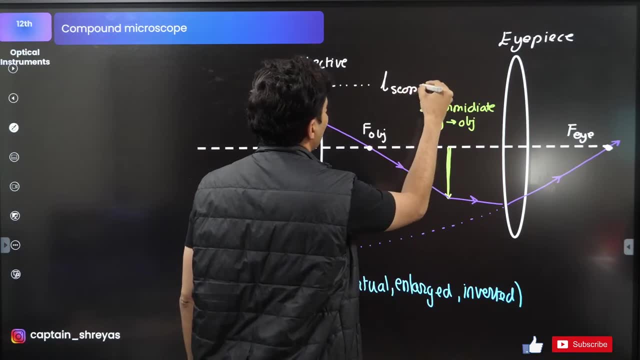 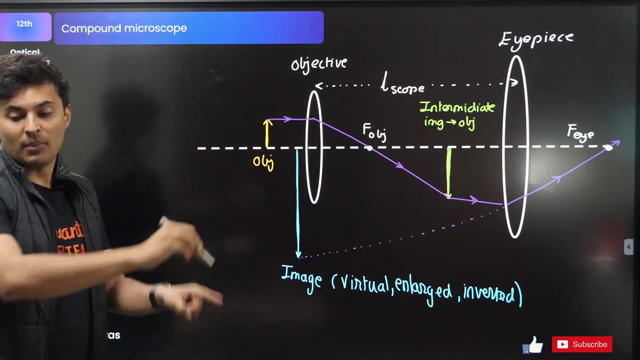 is formed. one more thing: the distance between the objective and the eyepiece. the distance between the objective and the eyepiece, that is called as the length of the microscope. the distance from the objective and the eyepiece, that is called as the length of the microscope. keep these things in. 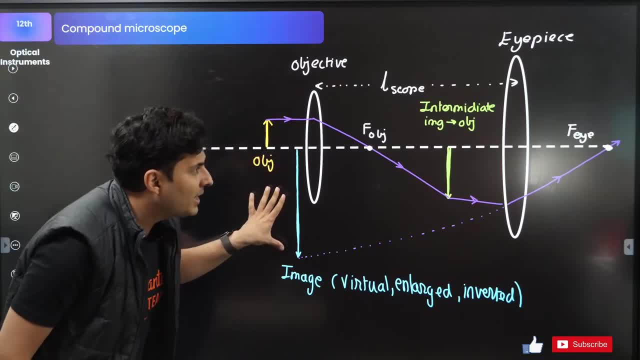 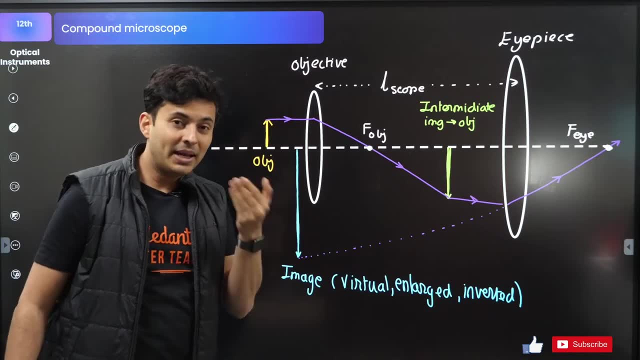 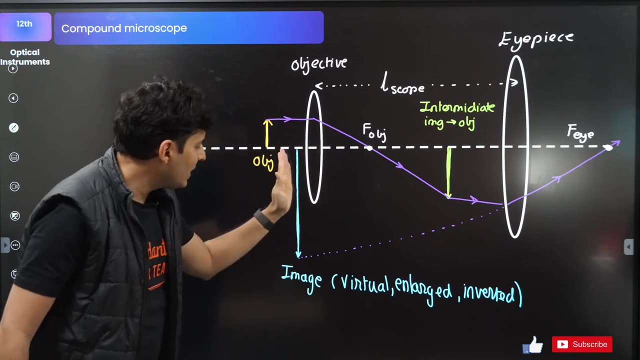 mind. now, if the image is formed very close to the eye, what will happen? the eye will be strained, yes or no, but the benefit will be you will get a good magnification. the magnifying power will be great. if this image is formed very far away from the lens or the your eye, then your eye will become 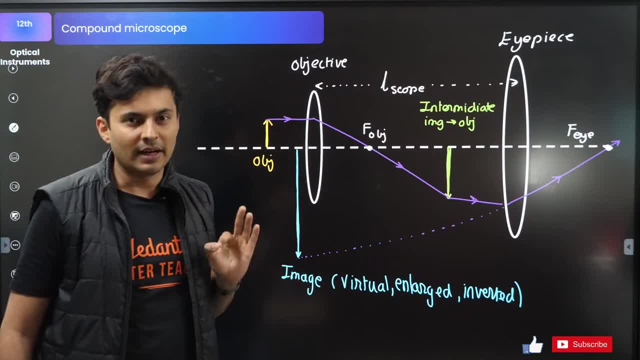 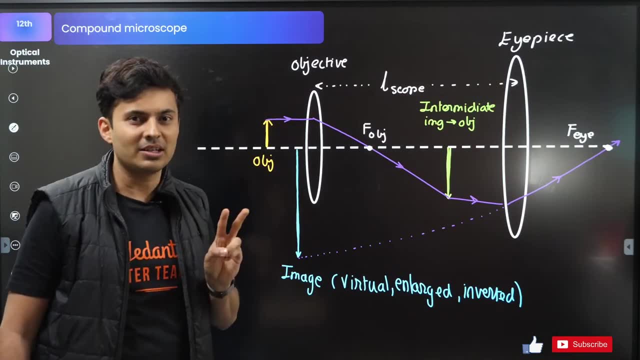 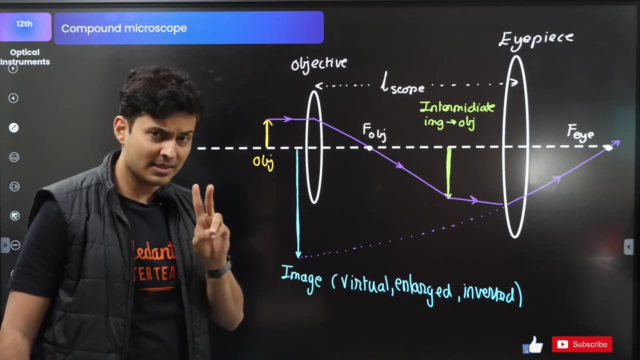 relaxed, but the magnifying power will also reduce. so, just like you had a two situations for a microscope, simple one compound also has two situations: one when the image is as close as possible to the eye, which is least distance of distinct vision case, and the second scenario is normal vision, when the image is formed very, very far away, although it is. 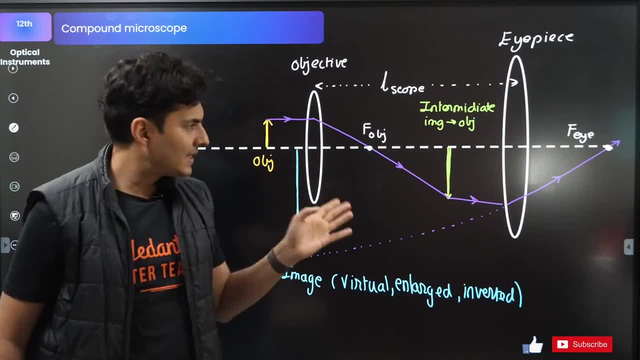 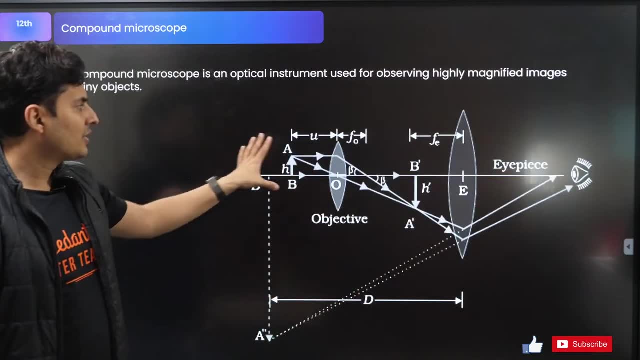 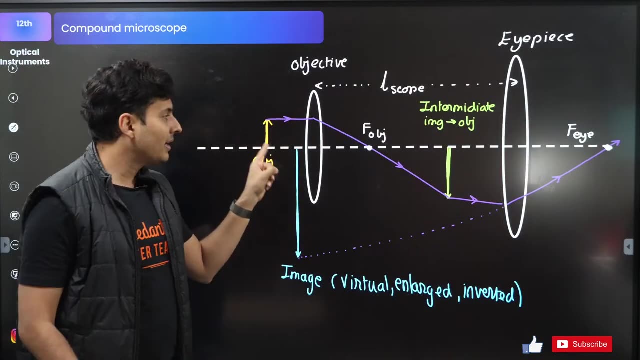 magnified, but you will see, the magnifying power will be slightly less as compared to lddv case. so the two situations. i will talk about it, but before that, this is your final ray diagram, which is usually shown in your books. it's exactly the same as this one. yeah, you might be wondering, sir, why haven't you shown the? 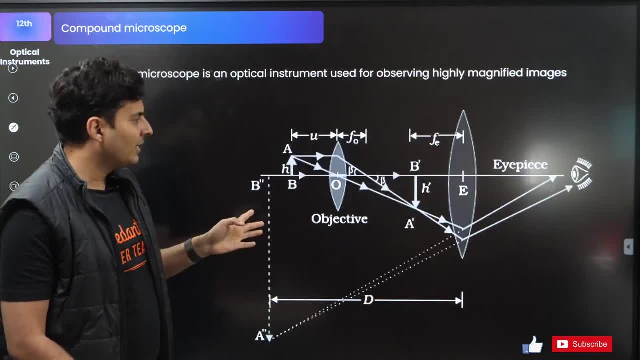 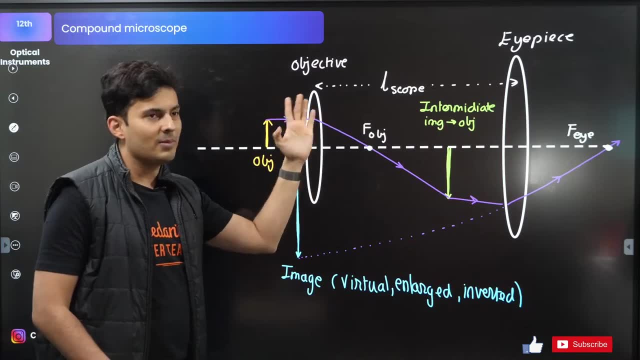 other ray. i could have shown the other ray, but it will just make the diagram very tedious so i had kept it for the other slide. here you basically understand what objective eyepiece length, where is the object, what kind of image is formed, etc. here this is the proper ray diagram. if you show the 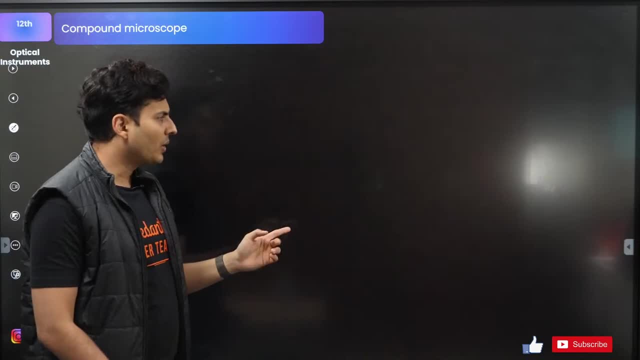 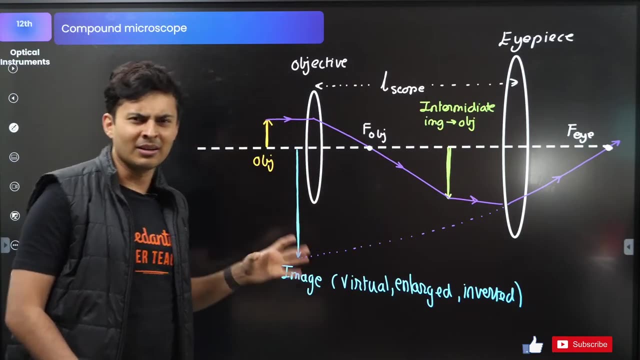 second ray. that is also fine, okay, so if you want, you can also show the second ray, which will make the perfect image here, and you can also show the second ray, which will make the perfect image here, and you can show one more ray going there and extended backwards, will make the image over here. 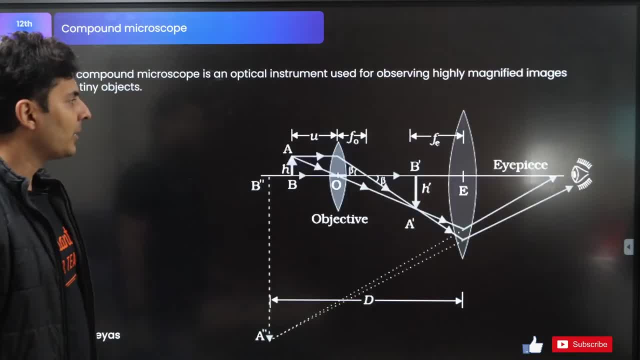 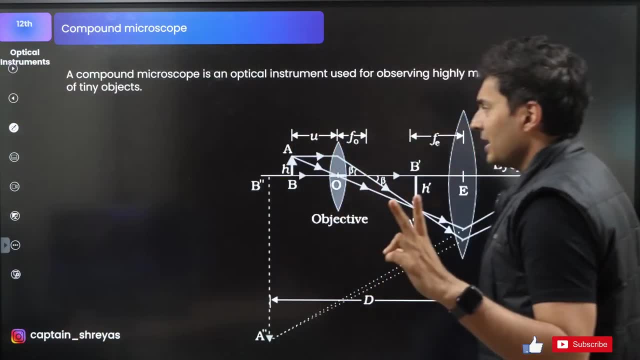 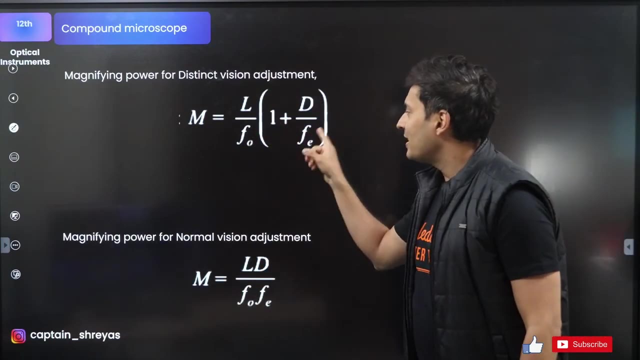 but i have just skipped that second ray. please keep that in mind. okay, now if i ask you what is the magnifying power? you should know the two formulas for both the cases. the first case. first case when it is at least distance of distinct vision. same thing, one plus d by f. 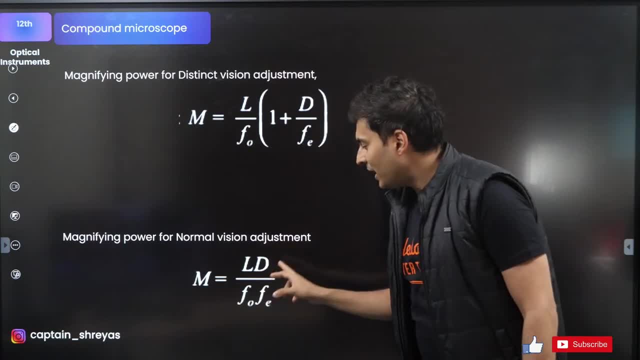 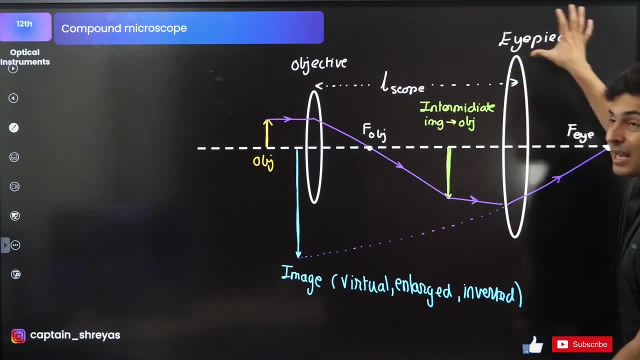 one plus d by f for normal vision. d by f is there, but there is one additional term because you have the lens. remember i told you that this lens eyepiece behaves like a simple microscope. so the formula is also like the simple microscope, only one plus d by f, or just d by f, the only additional. 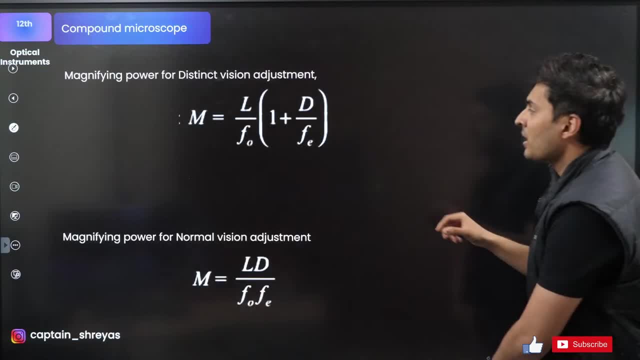 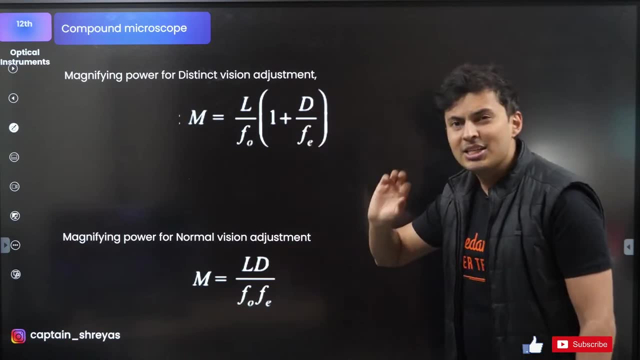 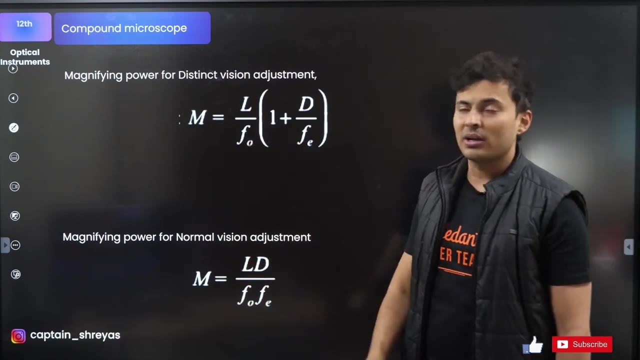 term which comes is for the objective. observe it carefully. one plus d by focal length of the eyepiece, just like your microscope formula. d by f, just like your microscope formula for normal adjustment. the only additional term is l by f naught, l by f naught. what is l? l is the length of the tube, l is the length of the tube, f naught is the. 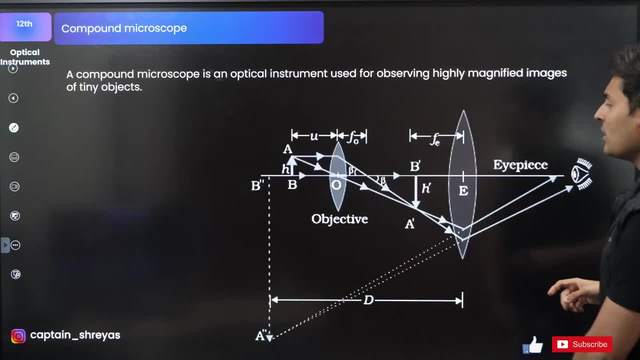 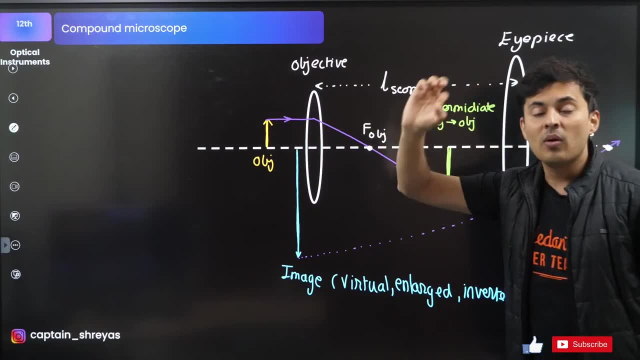 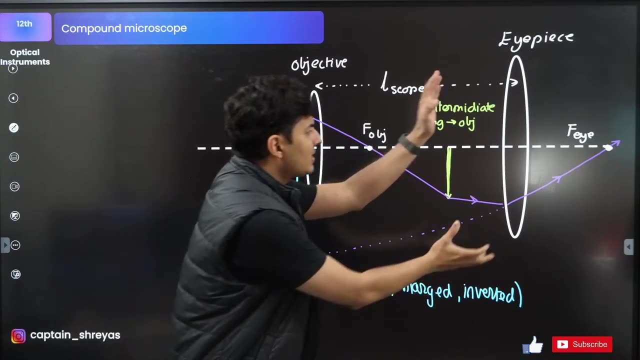 focal length of the objective. f naught is the focal length of the objective you can see over here. this is the focal length of the objective. length of the tube is basically l, so that's the only extra term which will come. so, guys, remember, a compound microscope is a simple microscope. 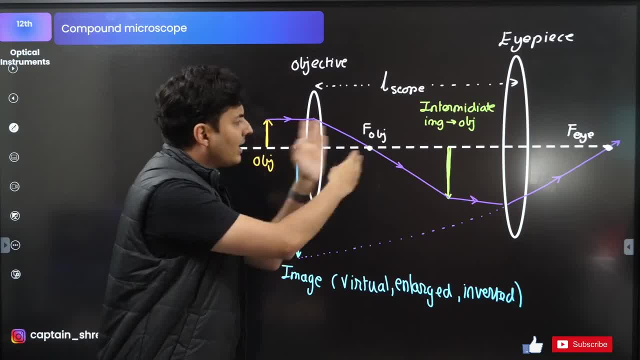 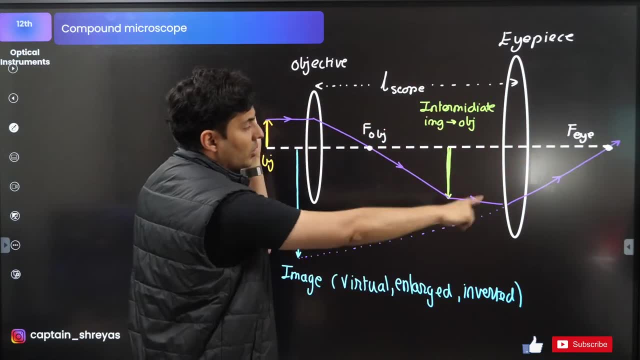 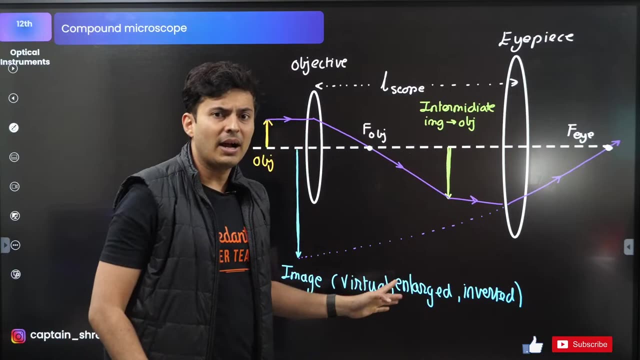 plus an additional lens which creates a real image. that's all. if you just look at ignore this and just look at this part, it just looks like a simple microscope diagram, nothing else. so the formula will be one plus d by f, or just d by f into l by. 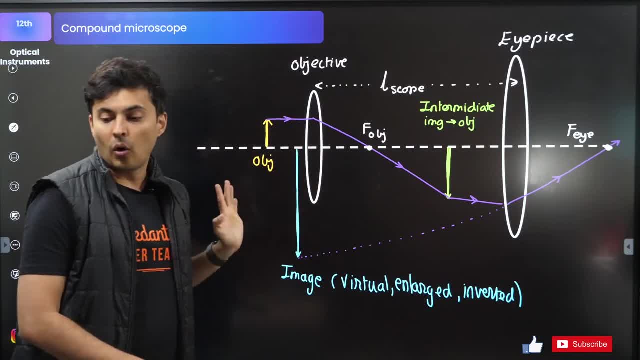 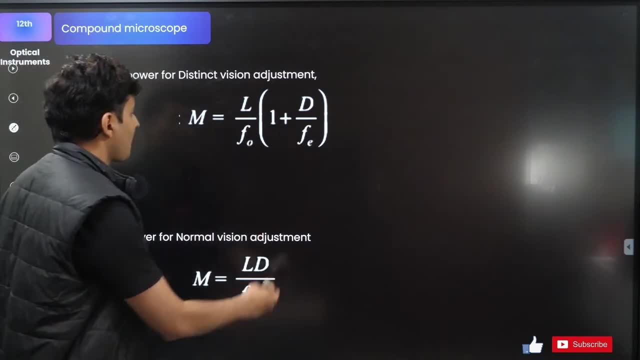 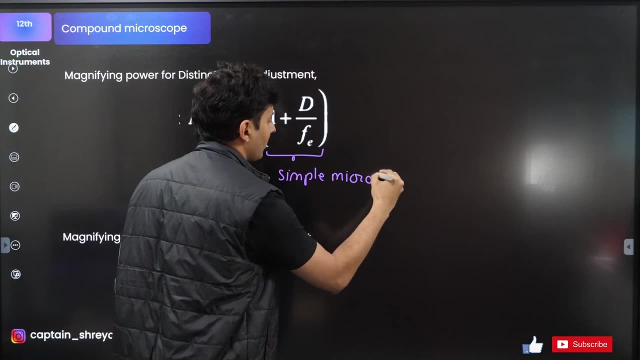 fe? l by sorry fo fo, is the focal length of the objective lens. that's all you can see that. see if this is very, very clear. see if this is very, very clear. so this much part is just like your simple microscope. simple microscope. even this part over here, this part over here, is just like 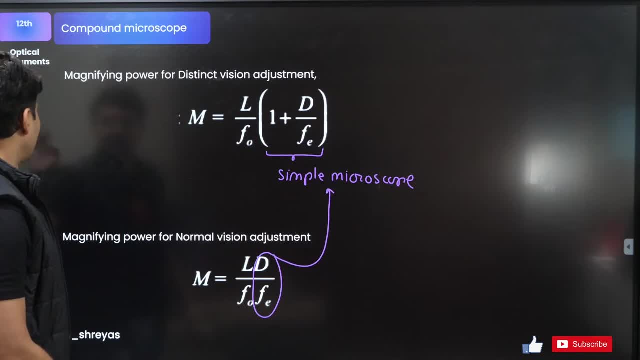 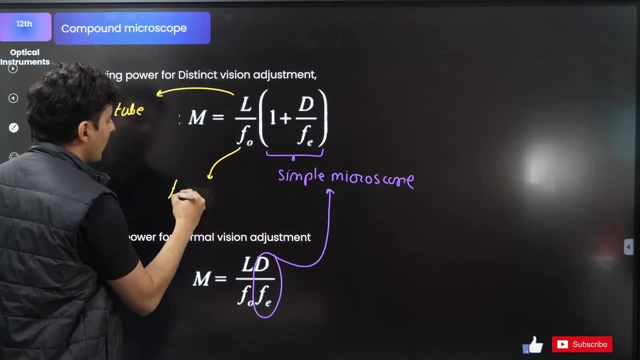 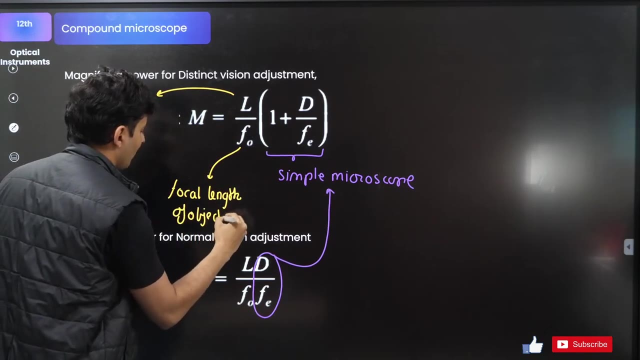 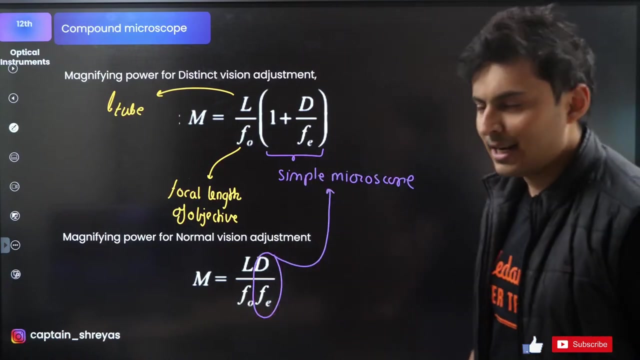 the simple microscope. only this l by f naught is that extra part where this l is basically length of that particular tube. this fo is the focal length of the objective, focal length of objective lens which is close to the object everyone. shall we do some questions ready, excited, put some heart or fire in the chat box. 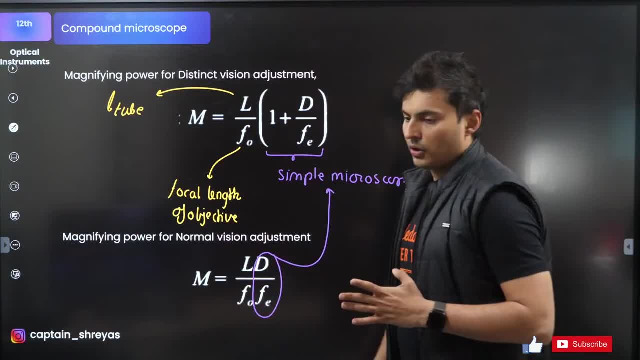 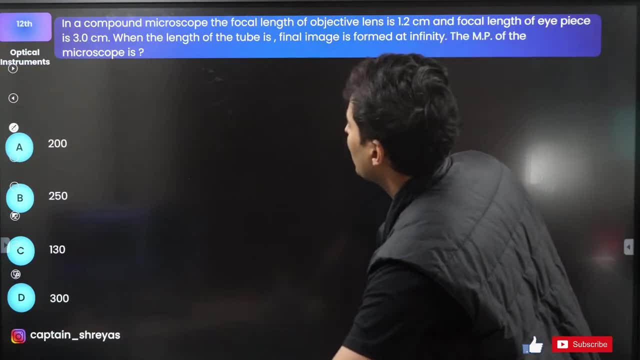 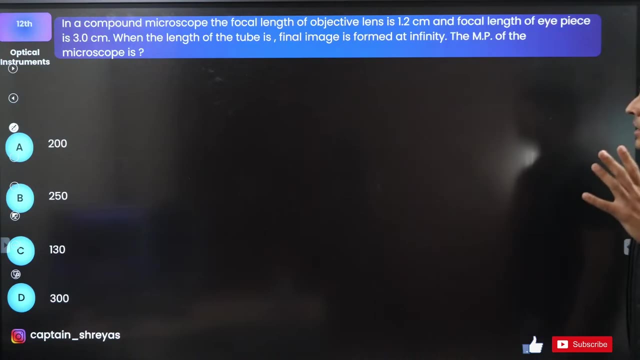 see if you have written this down in your notes or added to your notes whatever points were missing or whatever points you had skipped before this. let's do this question. in a compound microscope, the focal length of objective is 1.2. focal length of ips is 3. the length of the tube when the image 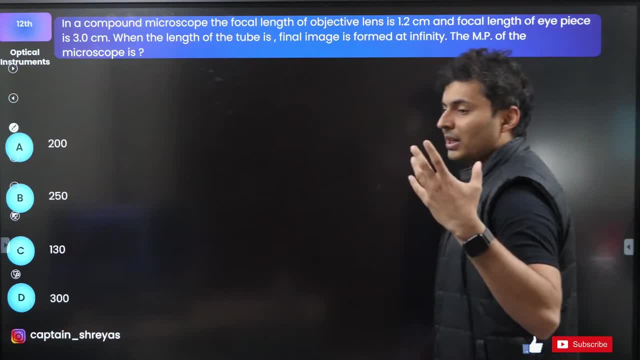 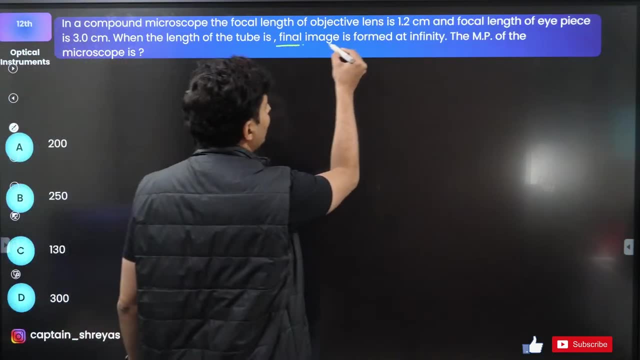 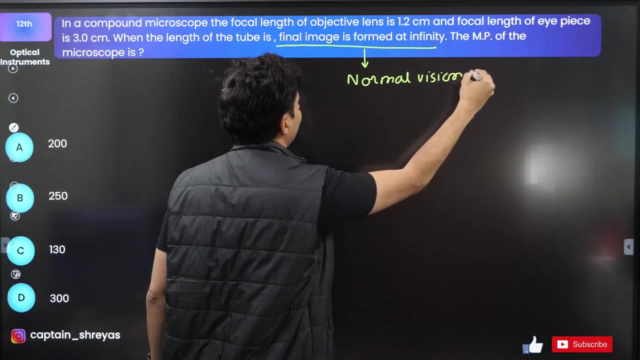 is formed at infinity. the magnifying power of the microscope is how much? let's do this question, guys. come on so clearly. it is mentioned: final image is formed at infinity. that means it is nothing but normal vision. it is nothing but normal vision. clearly it is understood. the question says what. 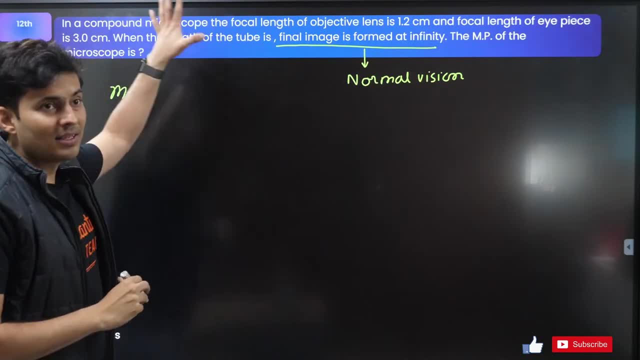 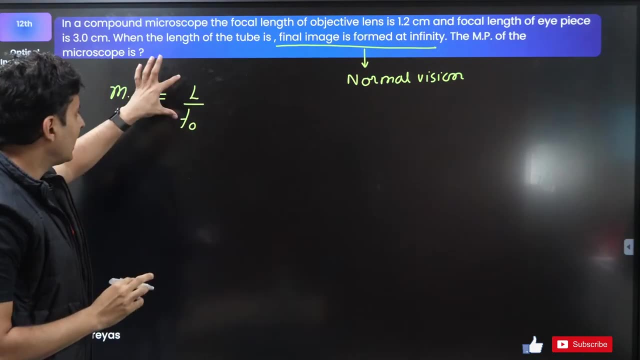 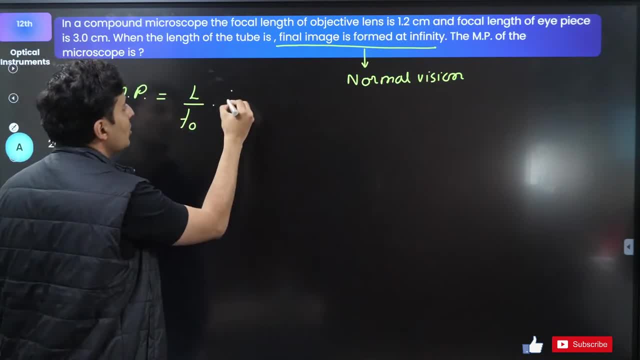 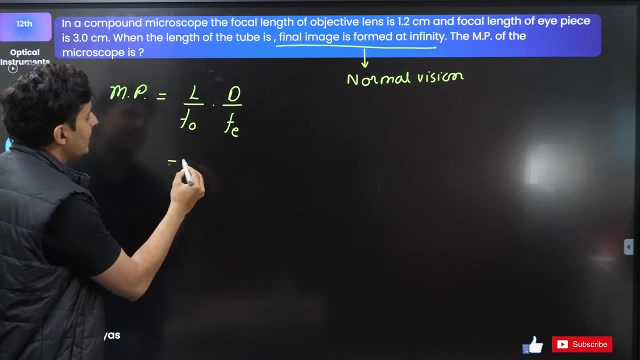 just d by f, because it is normal vision. i'm just going to use d by f. it's going to be slightly less, but this is for the ips, so this is the formula that i need to use. is the length of the tube given? uh, i think the length of the tube was something. i think it was 36. i think that is missing. 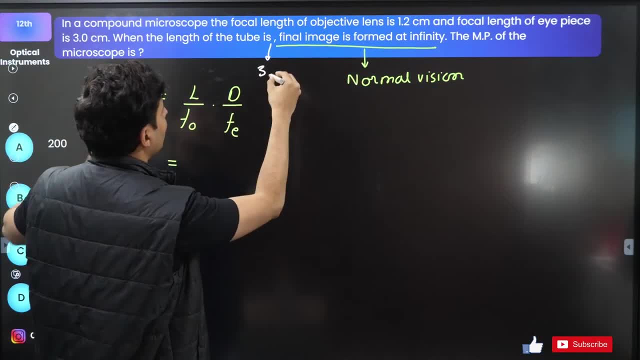 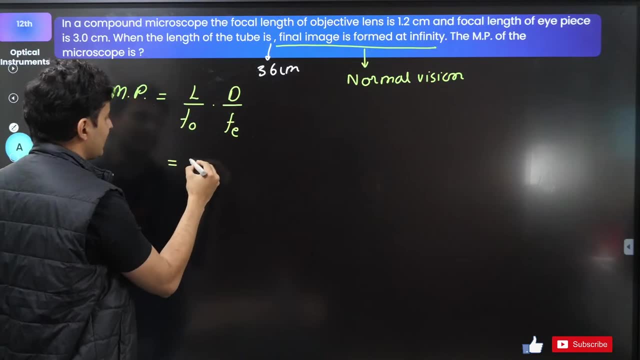 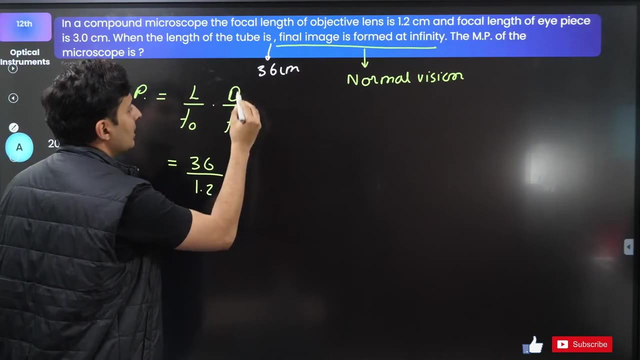 i think, the length of the tube. i can just look at it and figure out. yeah, it shouldn't be 36 centimeters, i guess. so let me just write it and just see what you get. length of the tube is 36 divided by focal length of the objective is basically 1.2 into least distance of distinct. 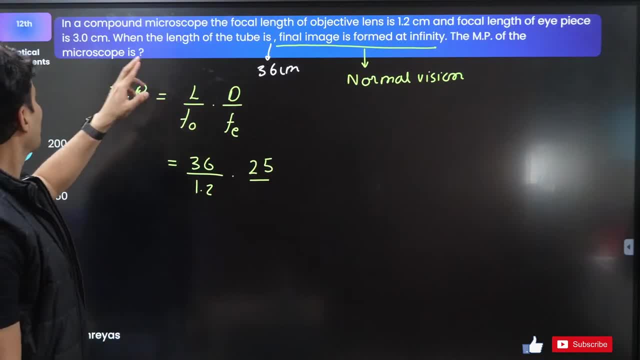 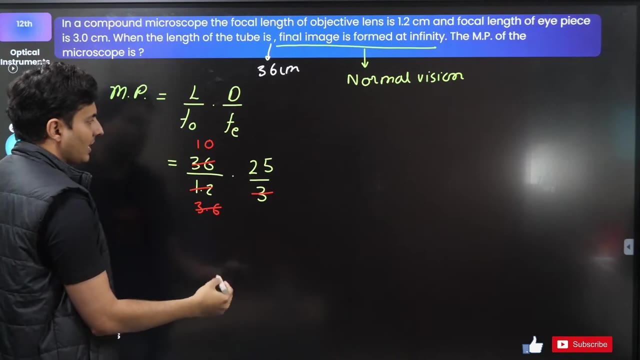 vision is 25. focal length of the eyepiece is basically 3 is basically 3. now you can see: 1.2 into 3 is 3.6. 1.2 into 3 is basically 3.6. 3.6 goes with 36, 10 times correct and 10 into 25. 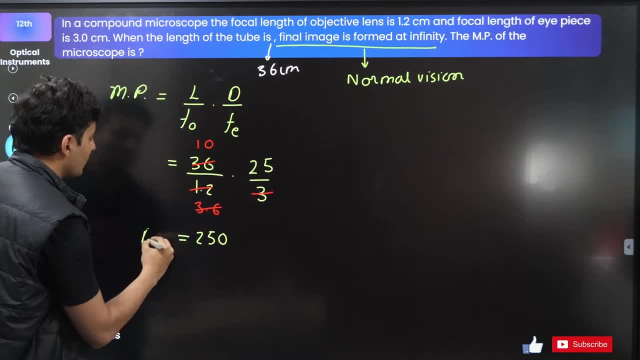 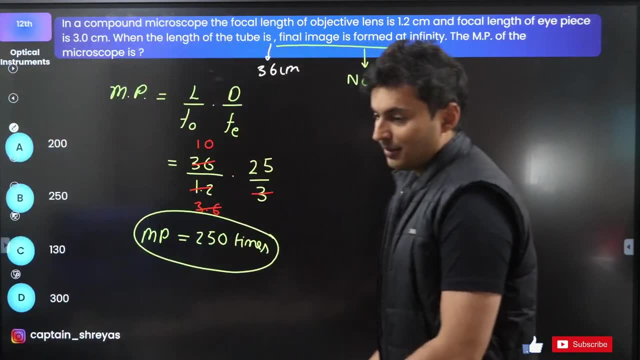 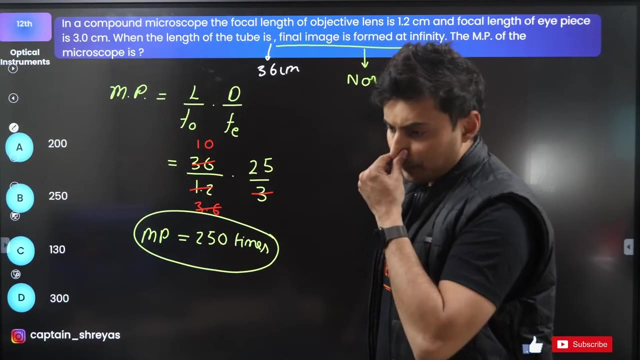 10 into 25 is nothing but 250. so the magnifying power is basically 250 times 250 x. yes, ashwita. yes, perfect, yes, sarvana, it is there. it is there. uh, for j advanced this year. i let me check bacha. i'm not sure, because usually 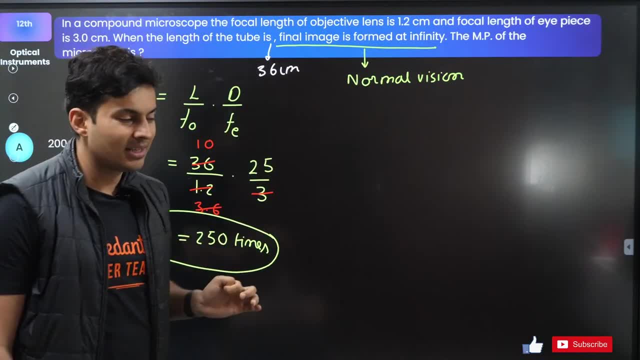 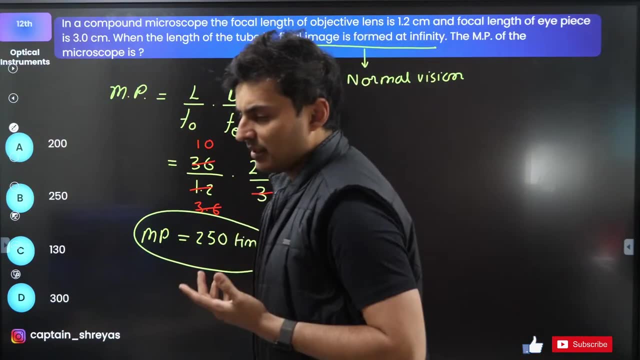 it was not there, but this year i think they added few extra topics. i don't remember clearly whether they added j uh, you know, optical instruments or not, because they added electromagnetic waves and few other things. so i'm not sure, but i think they added a few extra topics. i don't remember. 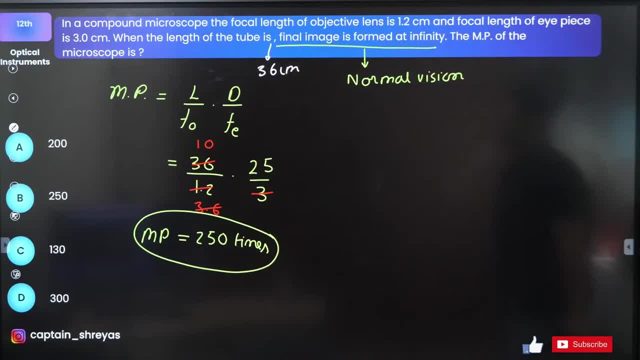 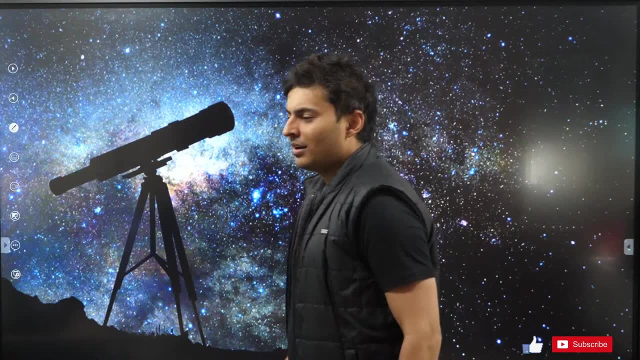 things. i don't remember it exactly. you need to check it. you can just check it online itself. okay, so every year they keep changing the syllabus. yes, option b is correct. now coming to the next part, and that is telescope. so whenever you see a microscope problem, remember. 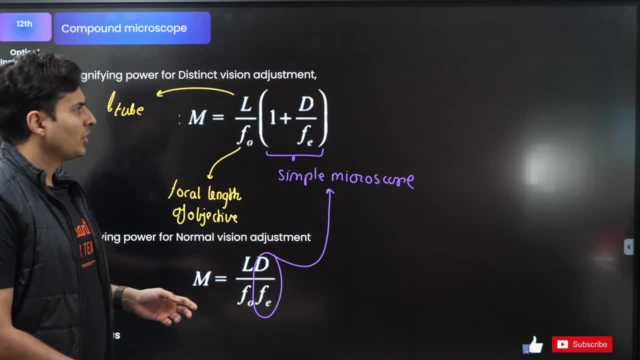 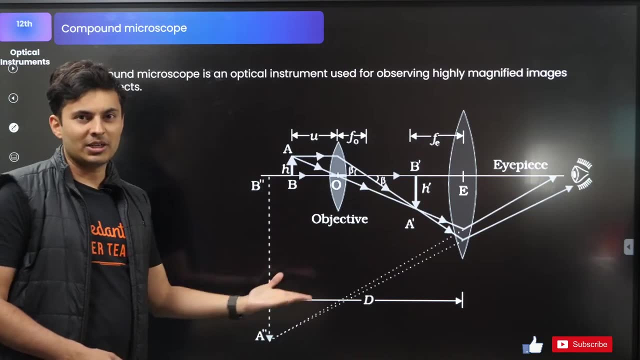 you will generally be using these two formulas. at the most, you might be asked to draw the ray diagrams in case of board examinations and they will be asking you how the image is formed, what kind of image is formed, etc. so these are the standard problems. direct application of the. 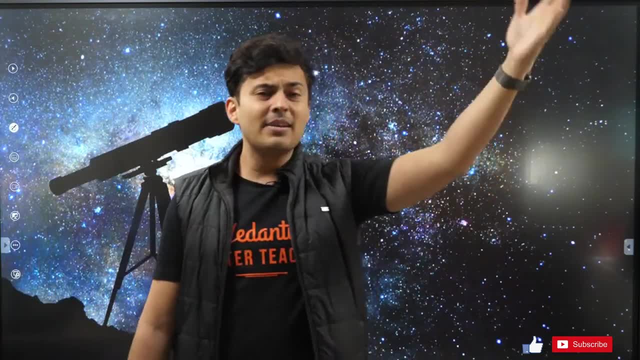 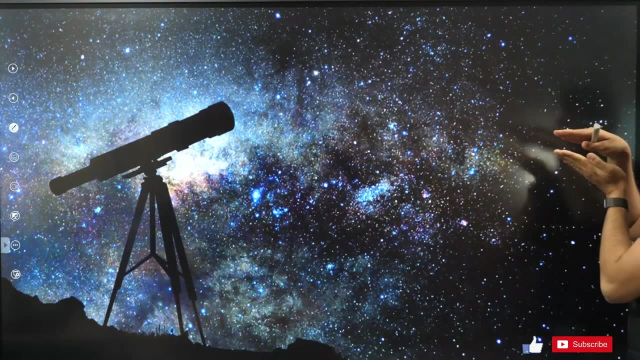 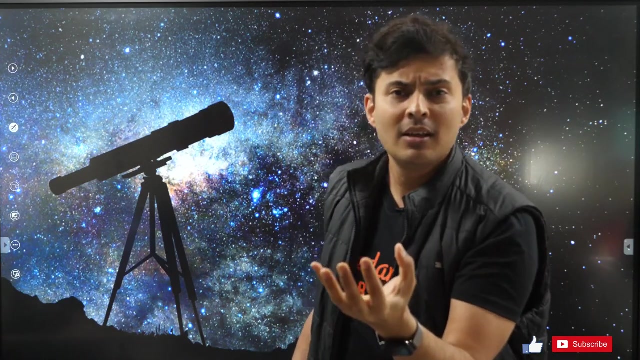 formulas, nothing great. now the object is very far. like you look at a star or the moon, the rays are almost going to be parallel and the object is going to subdend very small angle on your eye. so to see it very clearly, you want to make sure that those parallel rays get magnified. 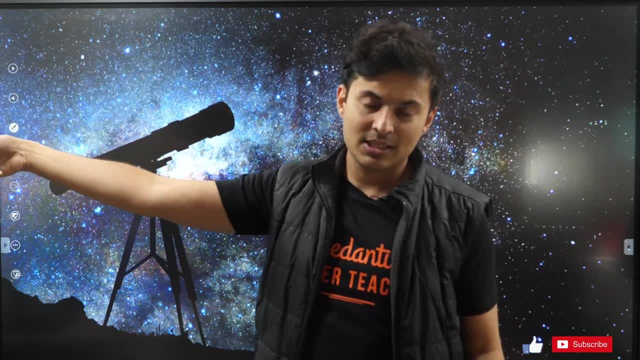 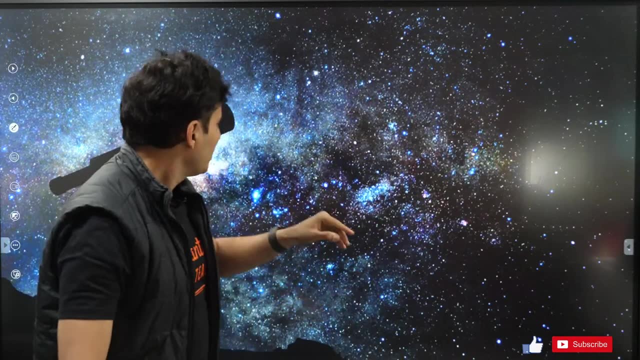 and you get a big image formed behind the lenses. again, the arrangement is very similar to a magnified image. the arrangement is very similar to a magnified image. the arrangement is very similar to a microscope. you are going to have two. you are going to have, basically, two lenses. 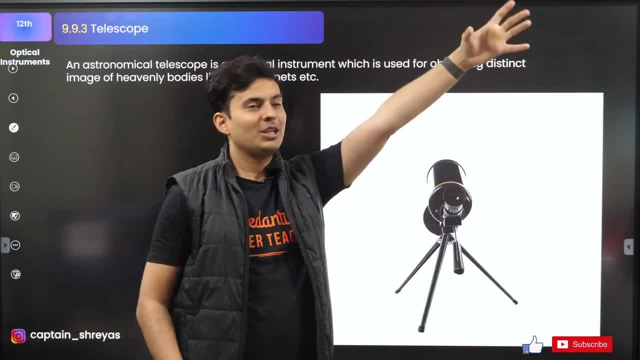 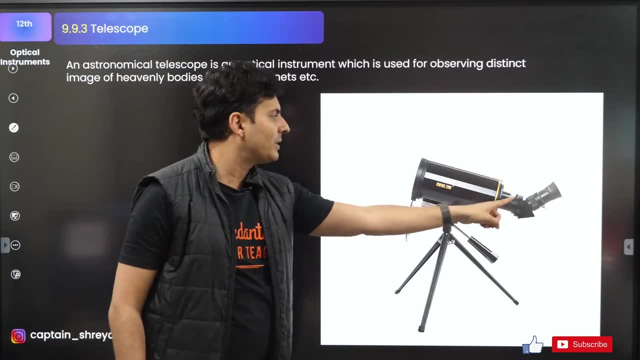 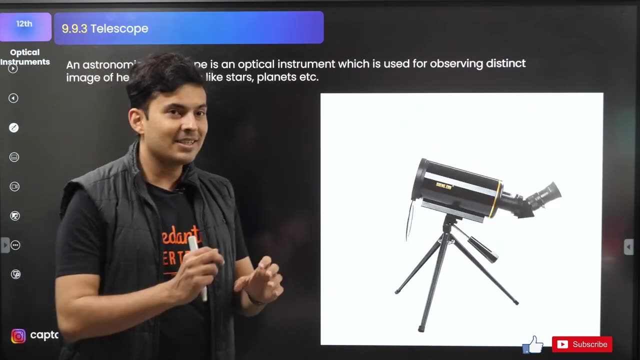 one is the objective, the one which is used to see the object and through one where you are going to put your eye and look into the telescope. that is basically your eyepiece. that one, okay. this one over here, okay. so that is basically your eyepiece and this is basically your objective. so this is. 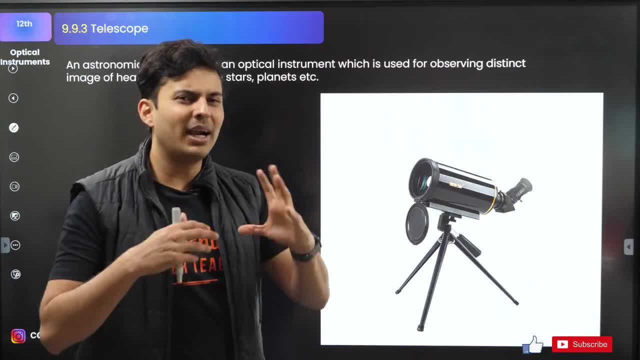 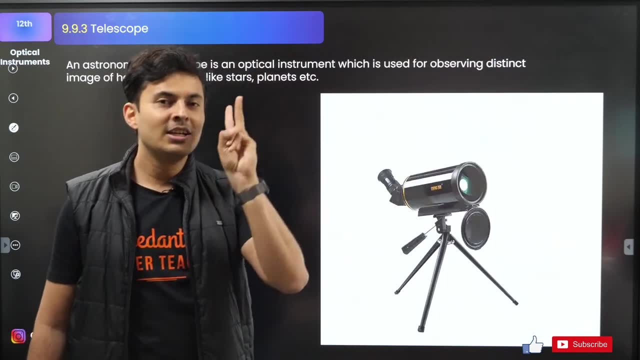 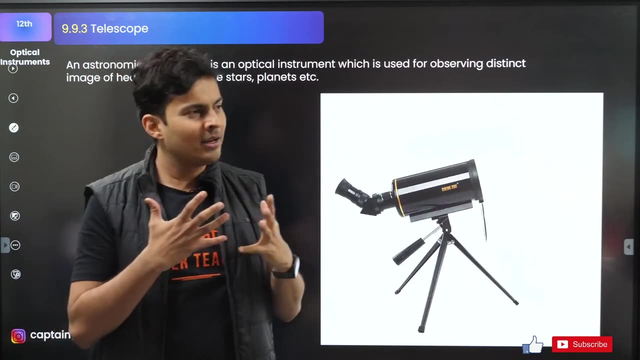 again very similar to a microscope, but there are some small changes here. the object is going to be at infinity. it's not going to be close. number one change. number two change is that the image will also be formed very far. it won't be formed very close to your eye because the object is very far, the image is also. 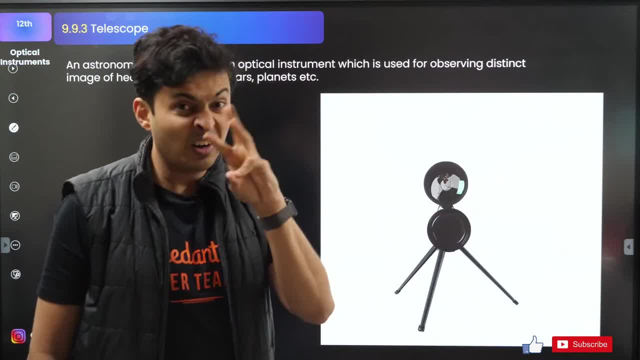 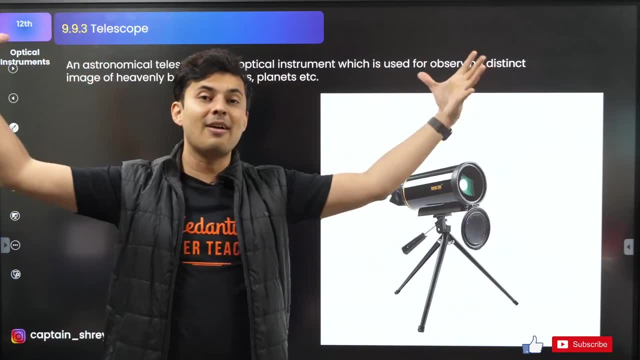 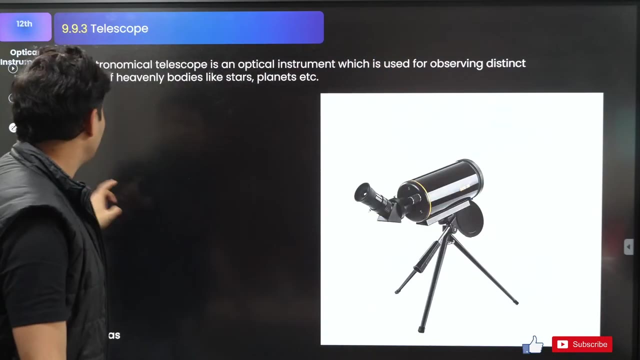 very far, but the image is very magnified. the third thing which is different is, you will see, the objective lens is very big. you will see telescopes have very large aperture. there are two main reasons for having a very large aperture of the eyepiece. so let me just mention that over here: the eyepiece. 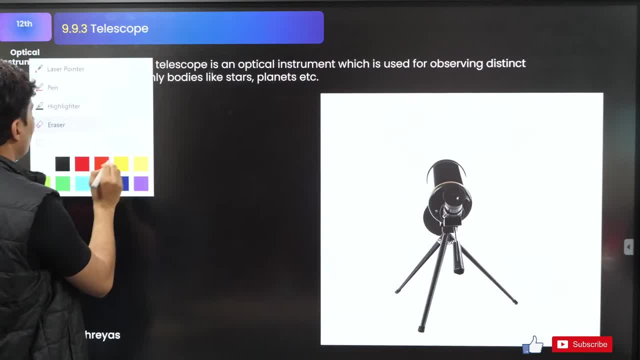 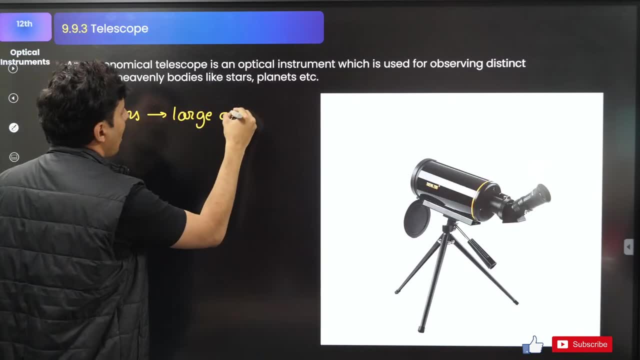 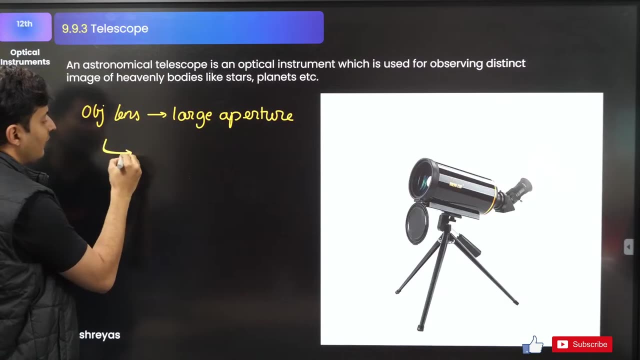 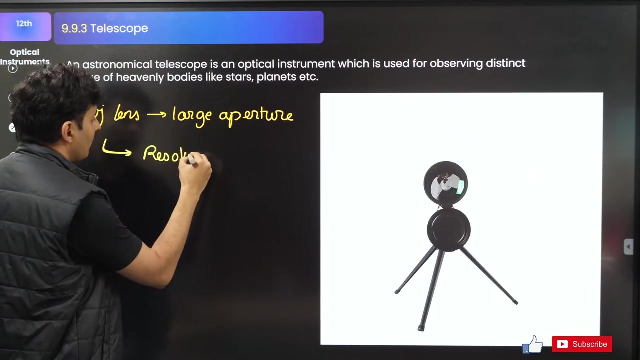 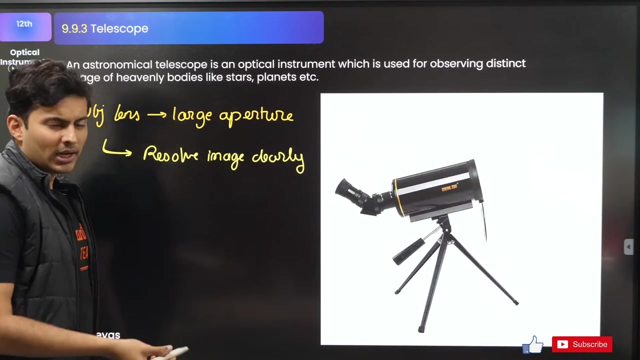 sorry, not the eyepiece, the objective, the objective lens. objective lens has a very large aperture. the reason for having a very large aperture is number one. the first reason is to basically resolve the images. to resolve resolve the images clearly, clearly. you will understand more about resolution in the wave optics chapter. so there is this. 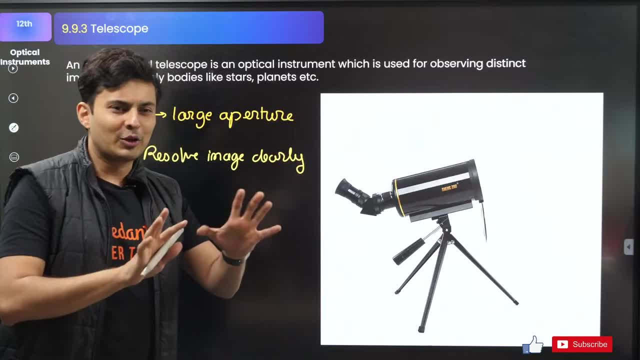 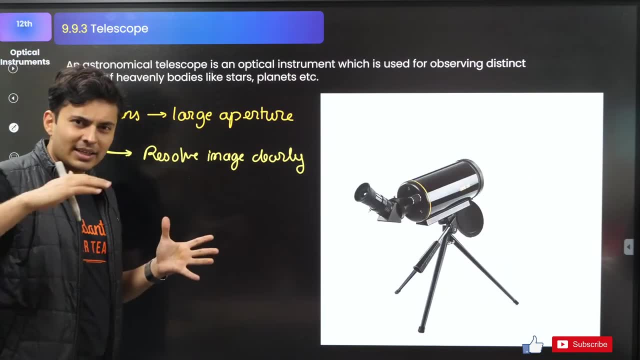 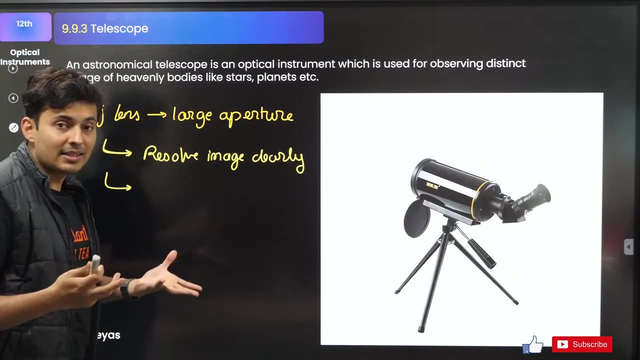 concept called as the resolution, which is based on diffraction effects, so the images are very clear, distinct. when you have a large aperture as compared to a small aperture, your diffraction effects get nullified little bit. and the second one is: accommodate more light, to increase the intensity of the light rays to see a more clear image. 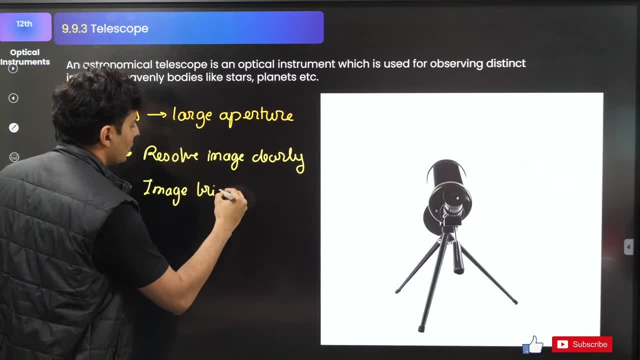 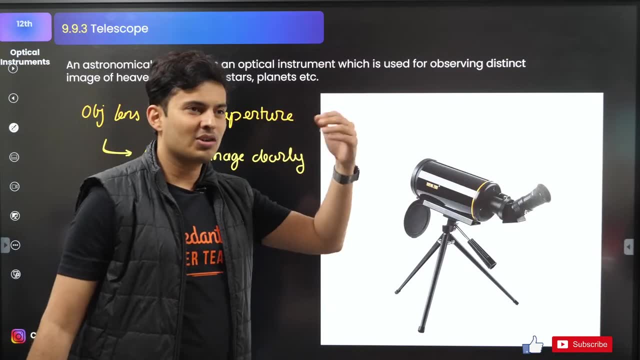 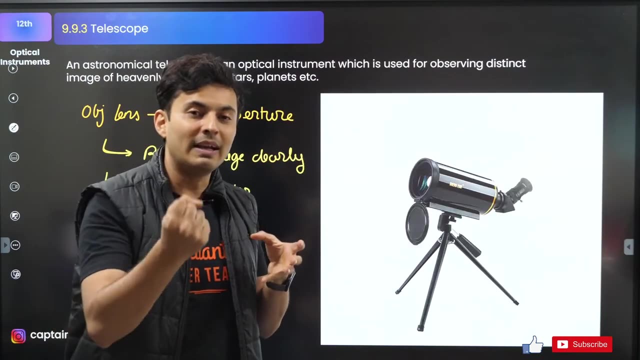 To make the image intense or basically brighter. to make the image brighter by taking in more and more rays, because when you see maybe Mars or some star, the light which is coming is hardly anything. So if you have more and more light rays, the image form will be more intense and bright. 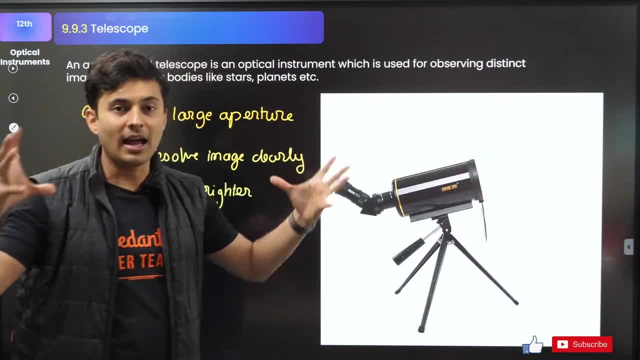 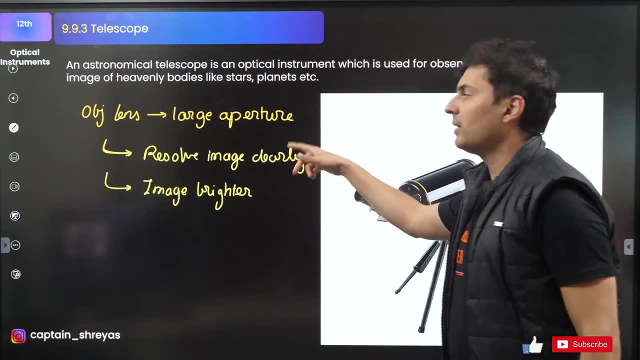 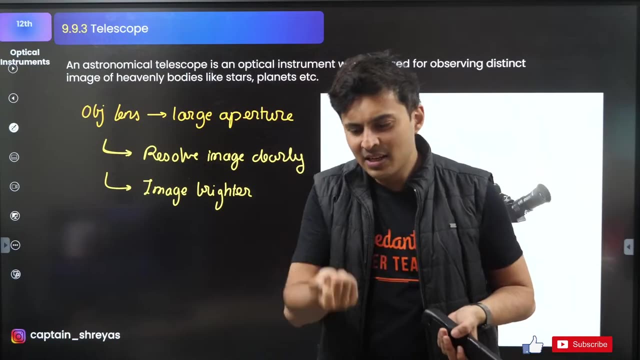 so that is another reason why you have a large diameter or an aperture of the objective lens. Is that clear? Is everybody understanding the two reasons why the objective lens of a telescope is large? For a microscope it is not needed. The object that you are seeing is only so small: bacteria, fungus cell. it is so small. 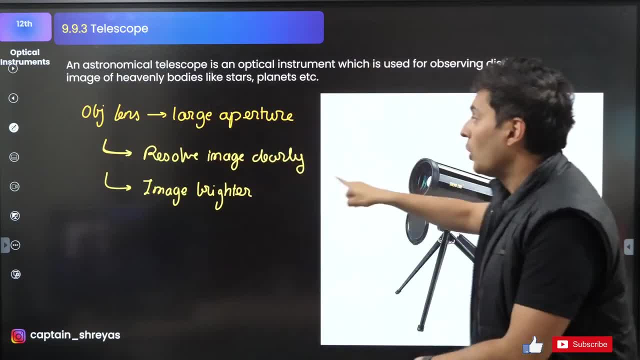 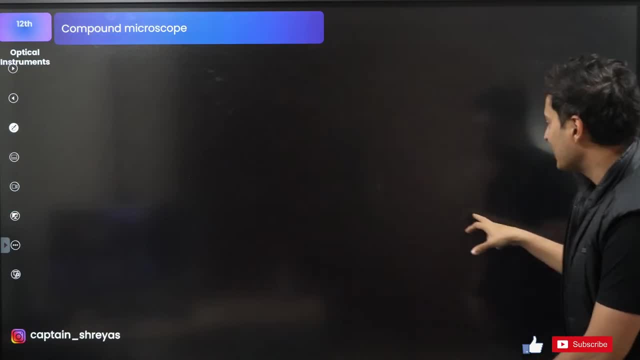 so having such a big lens is of no use. So that's why in a microscope you would have seen- I don't know how many of you noticed this- In a microscope The objective lens is very small. You can see that even in the actual diagram of the microscope. 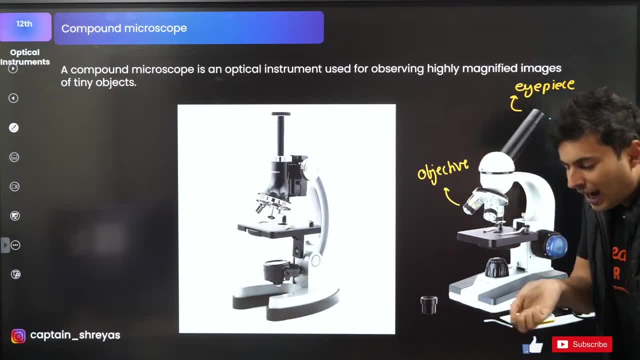 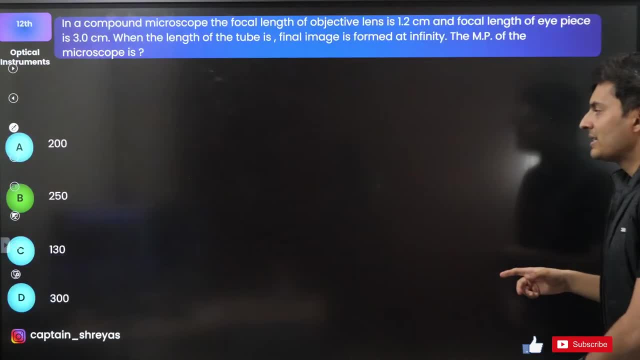 The objective lens is very small. so small because you are hardly seeing such a small object here. Why do you need such a big lens? It's a waste of money, material resources, So that's why you will see. only in the case of telescopes you will see that the objective 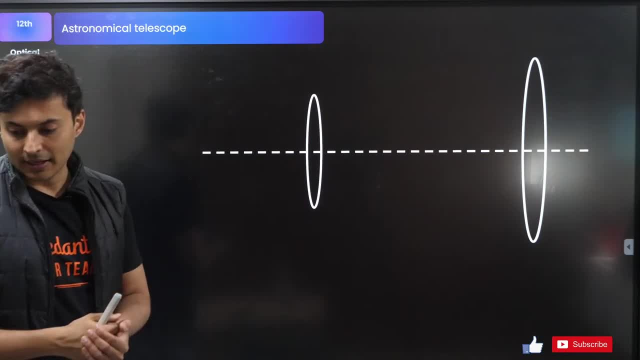 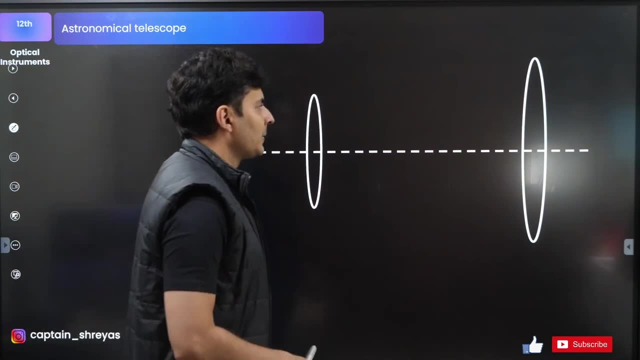 lens will be much, much bigger. Okay, great, great, Soma Sundaram, you can just replay the part later on and you can join in bacha. Okay, don't worry, The entire lecture is going to be there. So, in case of a telescope, the only change in the ray diagram will be: 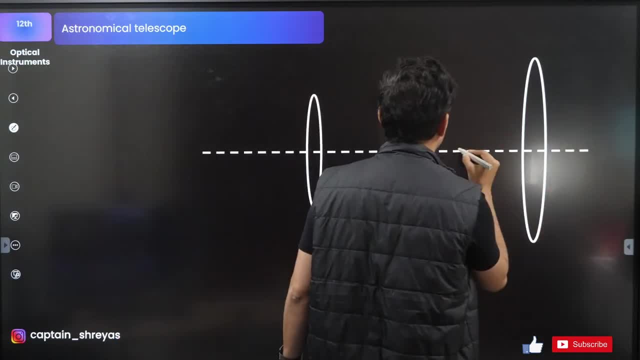 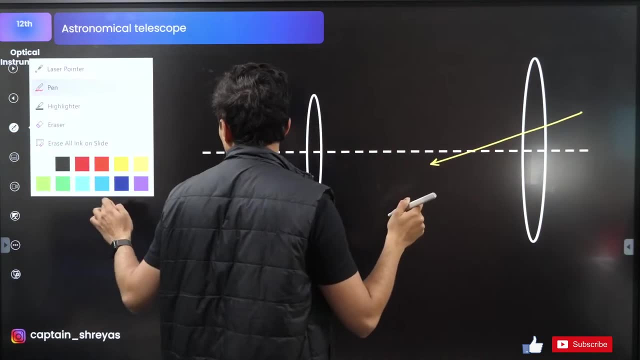 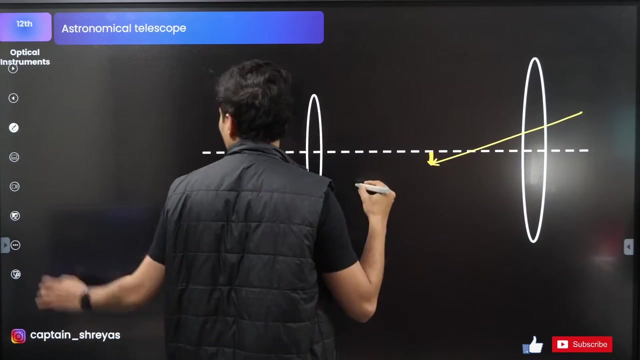 You will see that the rays. rays will come from infinity, Rays will come from infinity, from the objective lens, and it will form an intermediate image somewhere over here. It will form an intermediate image over here, So I would just say: Object At. 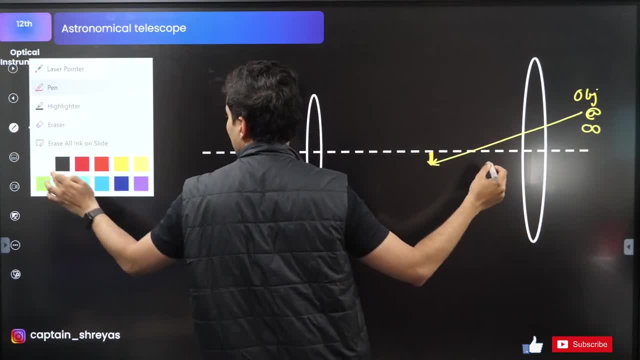 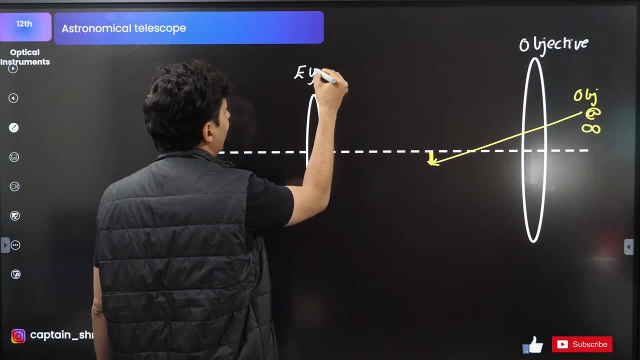 Length Of Infinity, Because the object is on that side. hence, this will be the objective lens, and this will be the objective lens, This will be the eyepiece. That's the big change. over here, The image is going to be formed. 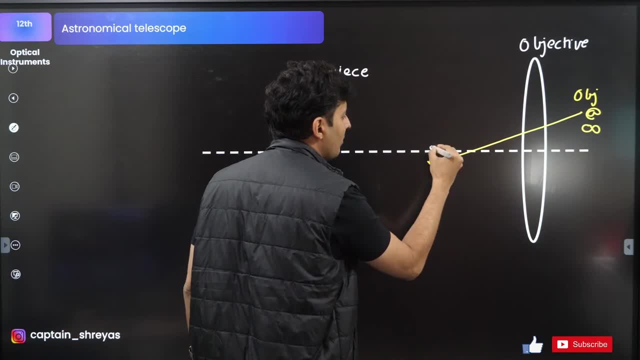 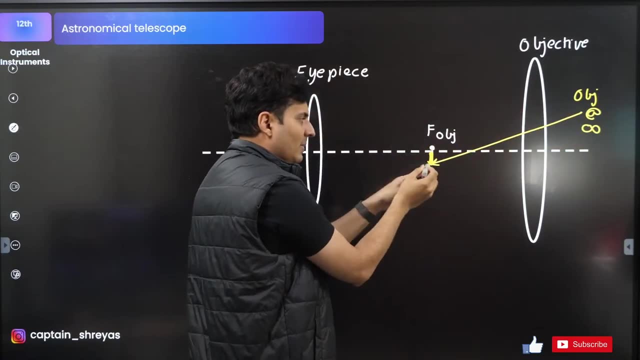 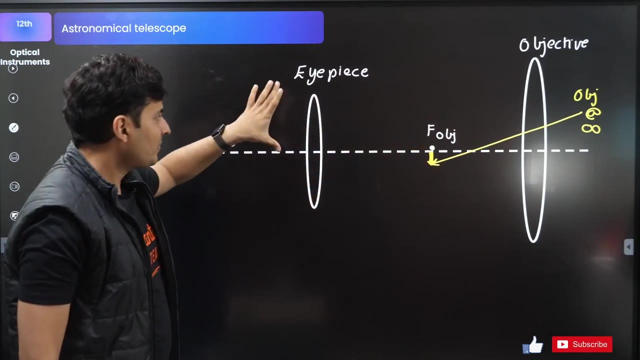 The image is going to be formed almost at the focal point, focal point of the objective lens, because, object at infinity, images will be formed on the focal point or on the focal plane. This image is placed in such a manner that this eyepiece acts like a simple microscope. 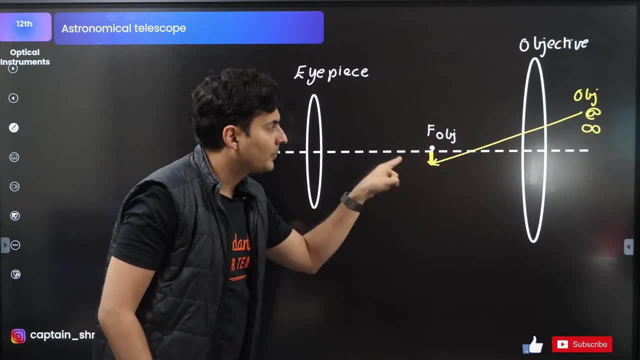 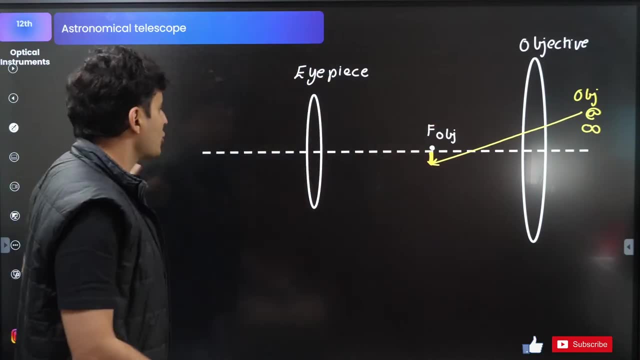 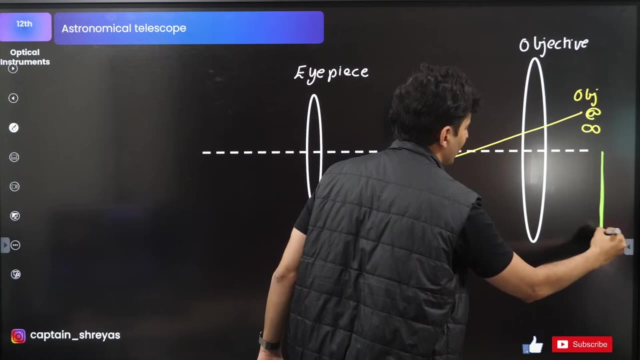 So it will make a magnified image of this object, This intermediate object on that side, which is magnified, It is erect with respect to it and it is also virtual. So you are going to see a big image on this side. So this image, I'm just showing it here for now, but actually this image which is finally, 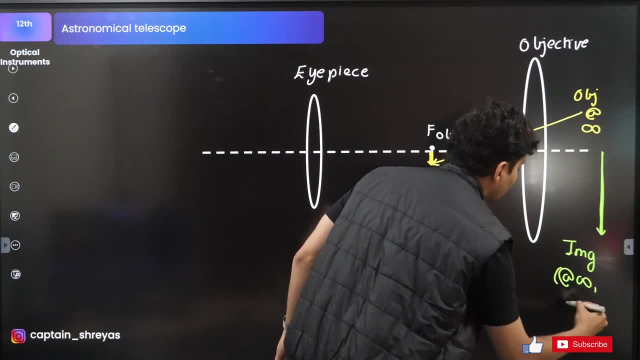 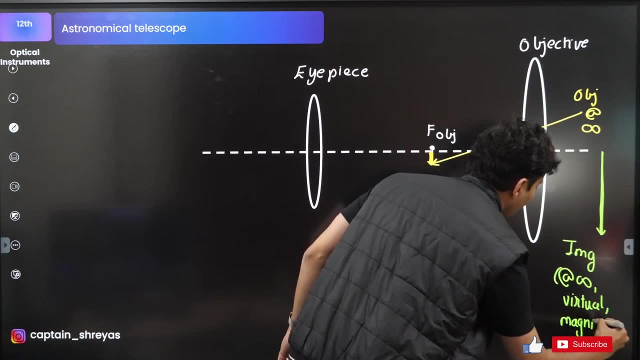 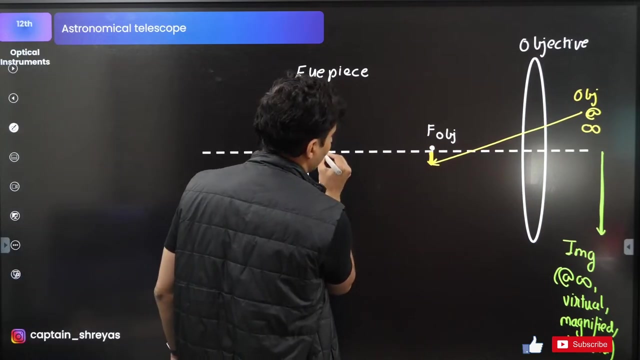 formed, It is at infinity, It is also virtual. It is also virtual. It is also magnified or enlarged. It is also magnified or basically enlarged, and it is also inverted in nature as compared to the original object. So if one has to show the ray diagram for this, probably you might show it like this: 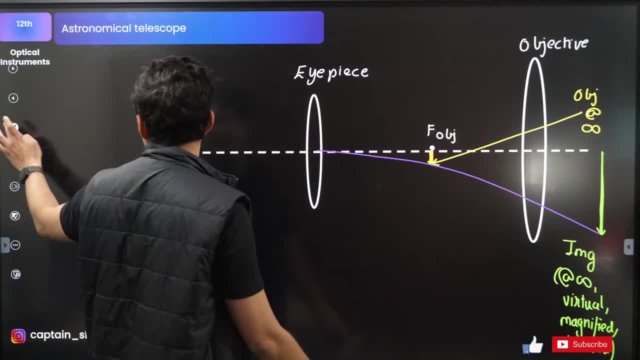 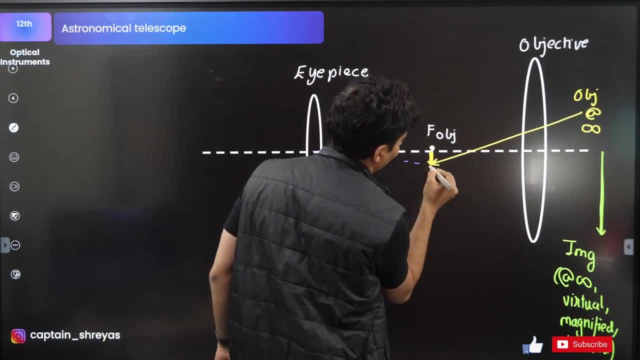 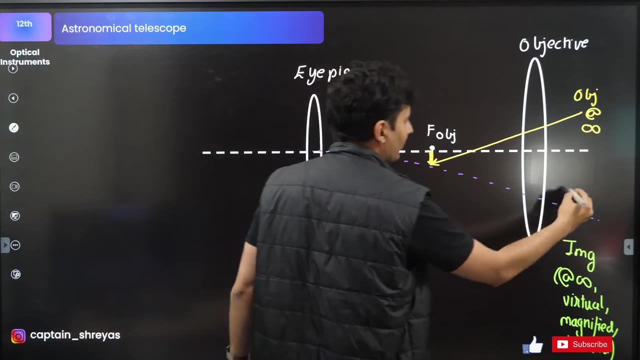 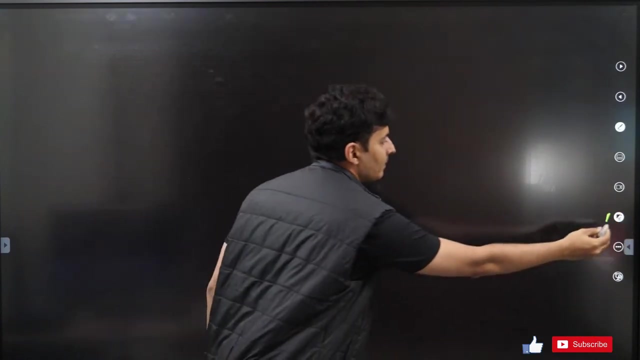 Oh my god, I think the ray only bent, So it's better not to show it because it's not to scale and I have not drawn it properly. So maybe, if I had to, I'll have to redraw this entire thing, Something like this: 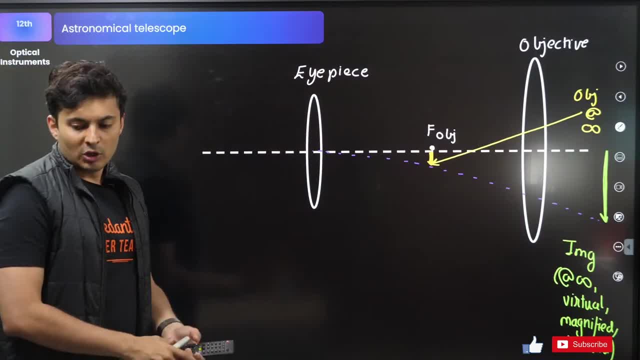 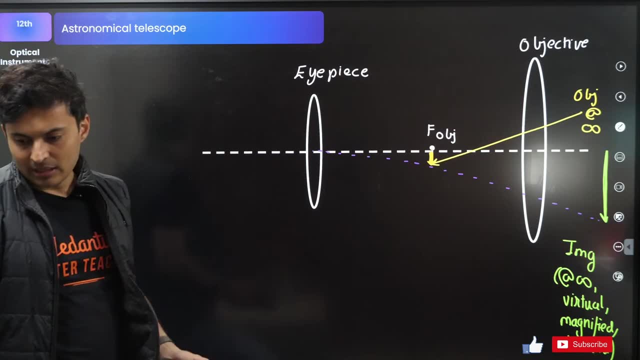 Now it's fine. Look at this Wave optics. I'm not sure. bacha, First time concentrating only on the heavy weightage chapters. Shaku, Okay, Should I follow my classes or learn derivations for my board, sir CBSE, Yes, you should learn derivative derivations for your board separately. 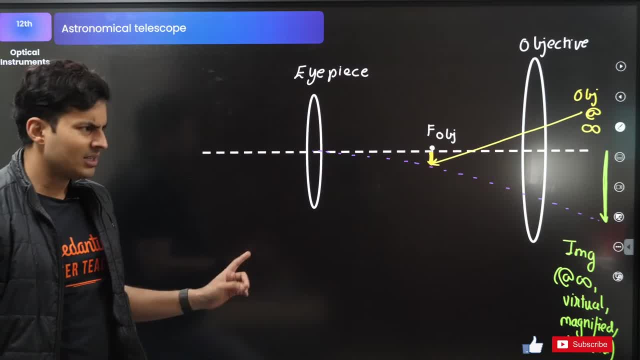 In fact, on J English channel I have done all the derivations and recently also uploaded some derivation classes on this channel as well. So please watch those derivation classes. It's there for boards. whatever derivations are required of at least the main chapters, I have done it already. 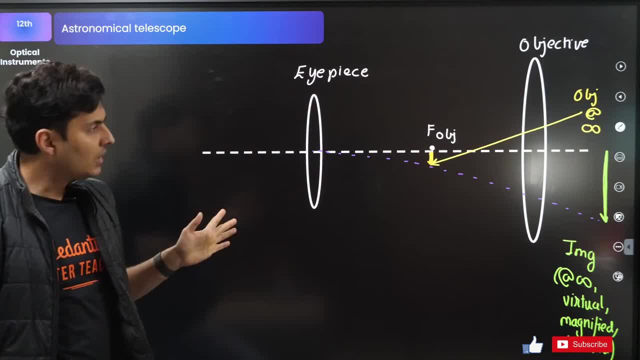 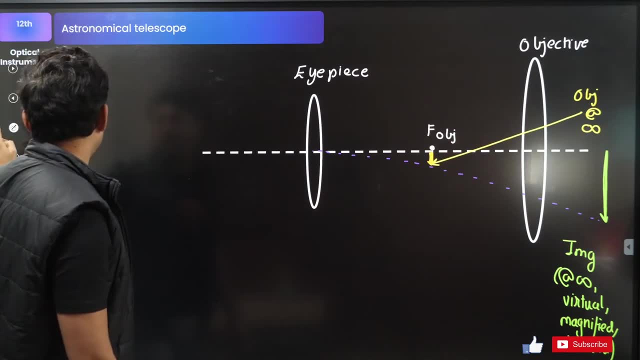 Just watch it. Okay, Everybody with me on this Understood Clear, Okay. So this is how the final image is going to be formed, and again over here you have the definition of length of the tube. again have the definition of the length of the tube. 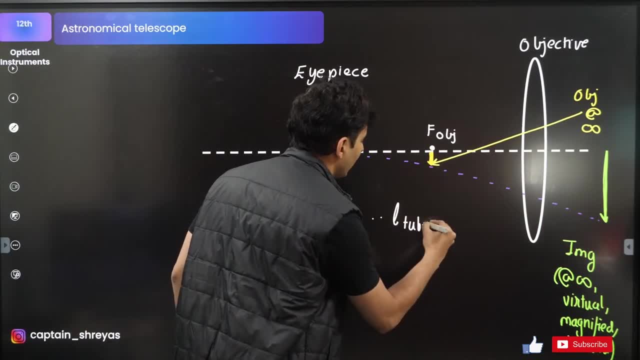 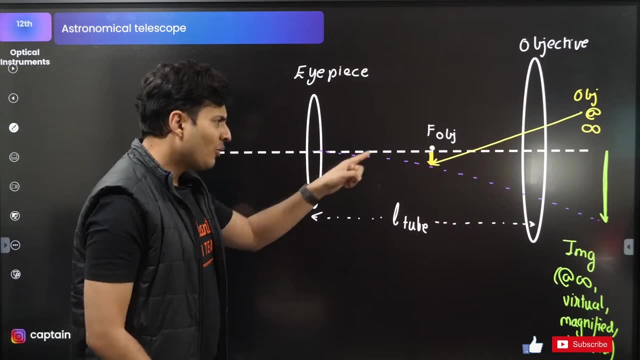 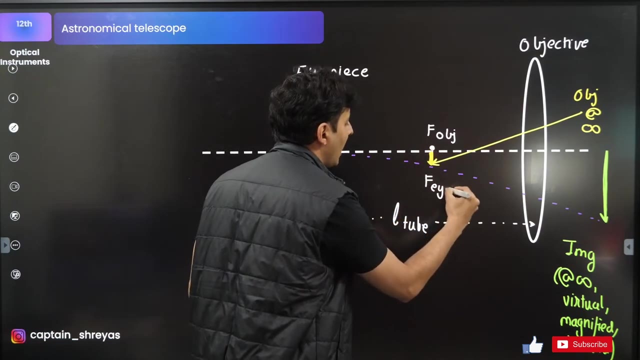 So this distance is basically called as the length of the tube of the telescope is a distance of the length of the tube of the telescope. and one more thing, guys: when this image is formed- because the final image is also formed at infinity- This point also happens to be the focal length of the eyepiece. 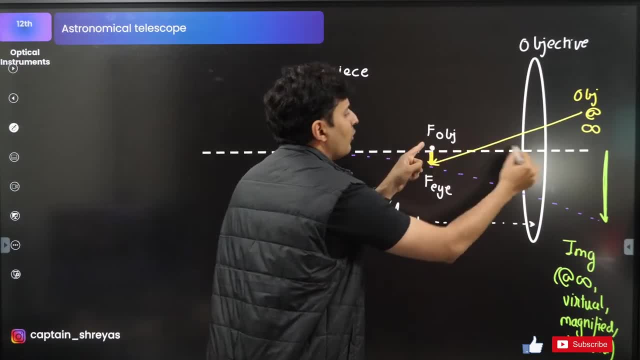 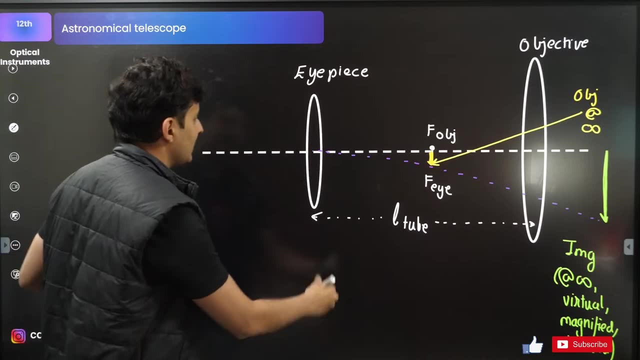 This is the focal point of the eyepiece. This is focal length of the eyepiece, This is focal length of the objective. So, in fact, from this diagram only, you can see one more interesting thing. I don't know whether you can see that this is basically the focal length of the eyepiece. 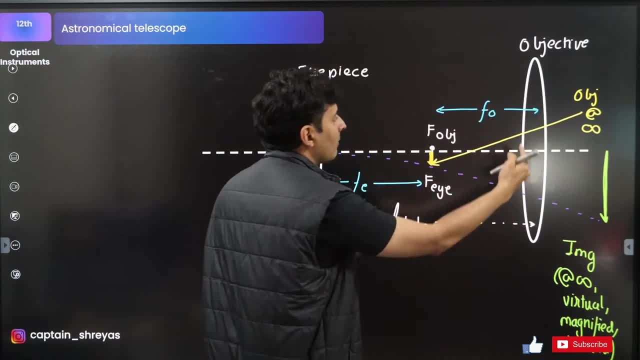 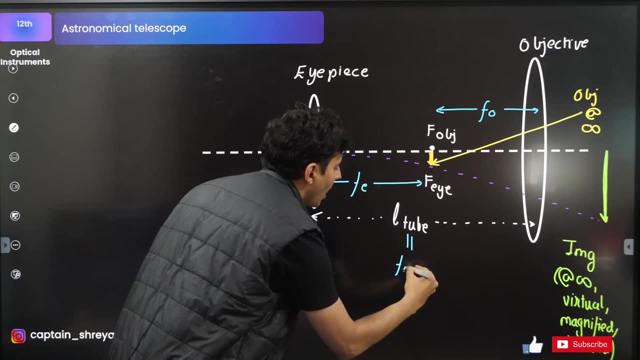 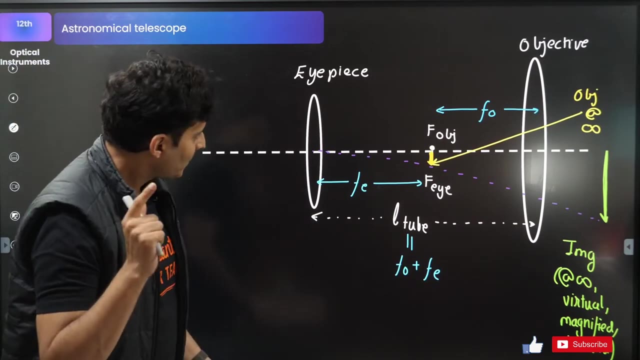 and this one is basically focal length of the objective. So FO and FE together give you the length of the tube. So the length of the tube, I can just say it is equal to F naught plus FE in case of a telescope. In case of a telescope, everybody clear about this, very good. 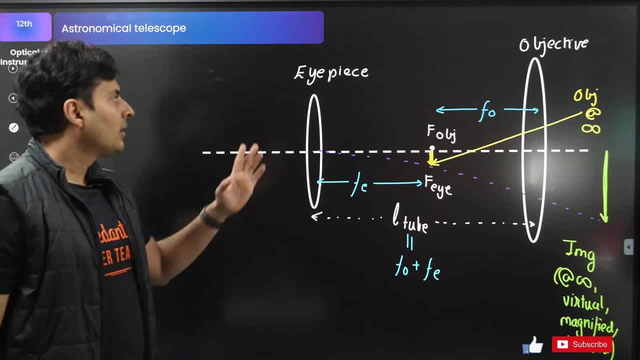 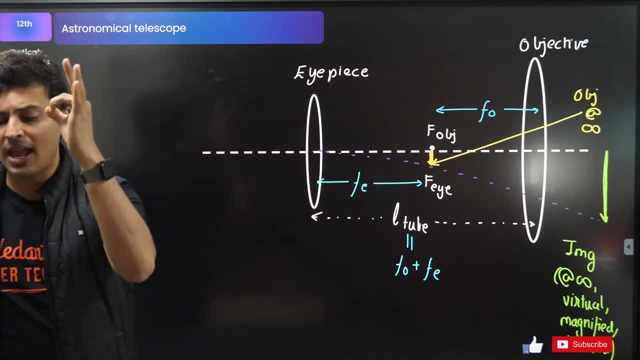 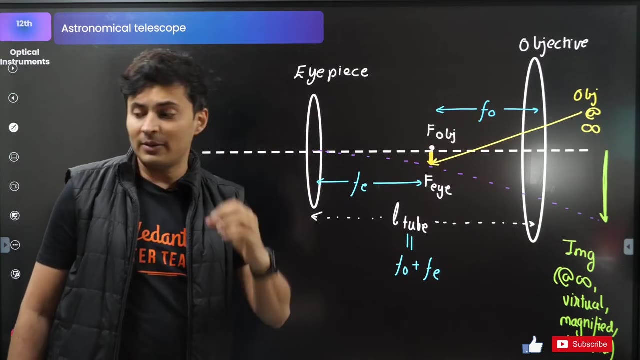 Now the magnifying power. you only thing can tell me: will a telescope be used in least distance of distinct vision mode or normal vision mode? I want answers from everybody out here. Is the telescope going to be used in least distance of distinct vision mode or normal? 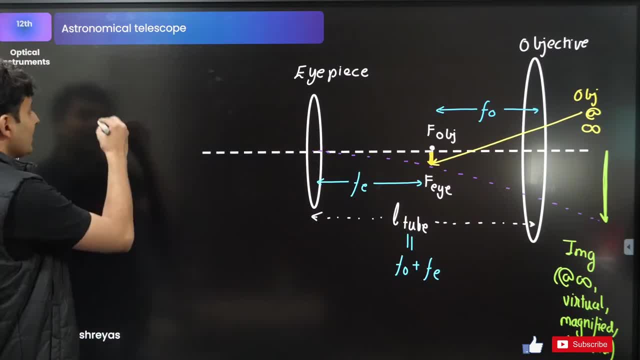 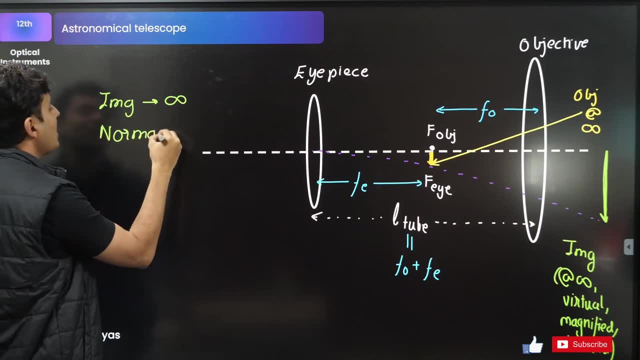 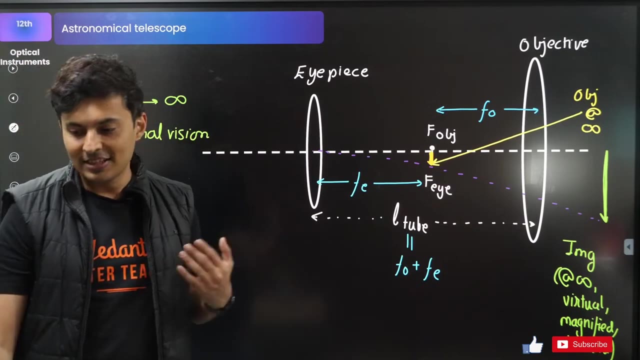 vision mode, Obviously. come on think about it. The image. image is formed at infinity, So the telescope is formed at infinity. That means it must be normal vision, yes or no? It must be normal vision. There is no case of least distance, of distinct vision. So there is only one formula for a telescope, and that is magnifying. 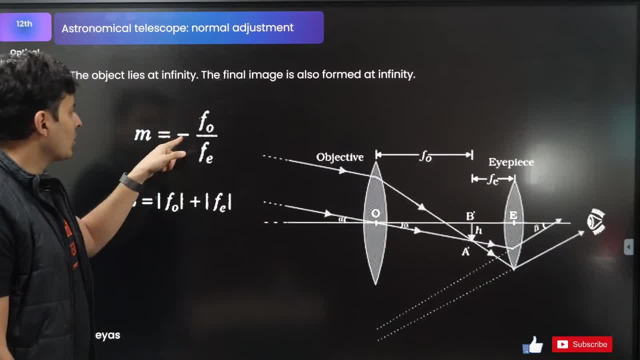 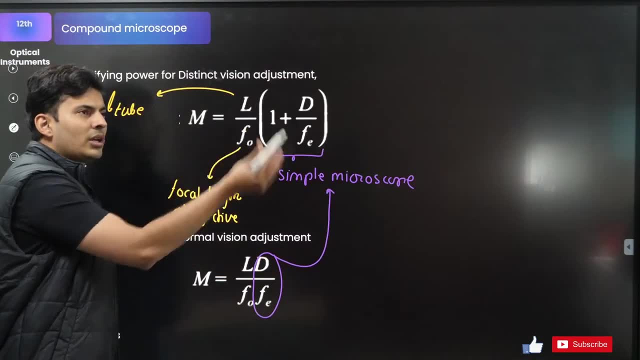 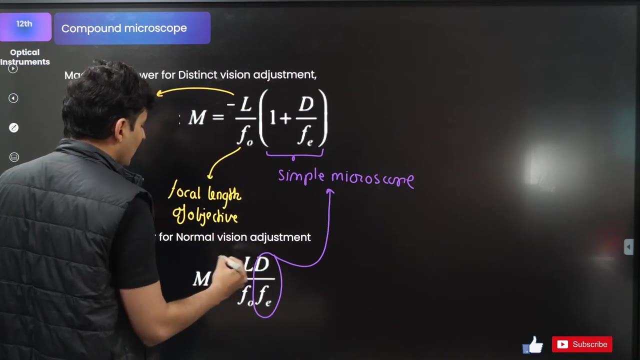 power at infinity, that is f0 by fe. Some books also put minus sign, not just over here, but some books also put the minus sign even in this formula. that is only to show that the final image is inverted. So don't get scared, even if you see a minus sign over here. Even if you see a minus. 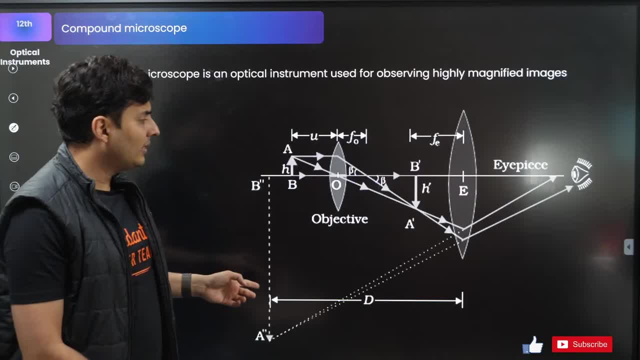 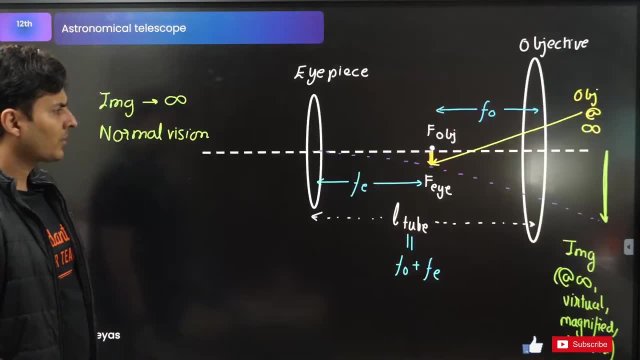 sign here and here. don't get scared. It is just because I know that the final image is going to be inverted in nature, be it a microscope or even for a telescope. guys, even for a telescope, the final image is inverted. So that's why you will see this minus sign. You can show it in either. 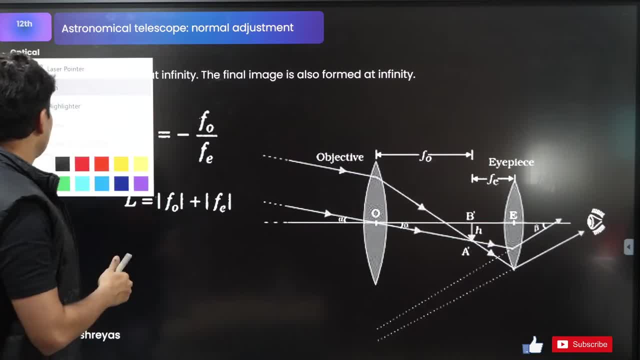 places. Just the magnitude will be f0 by fe. So this is the main formula that you are going to use. The length of the telescope is the width, which is are kob pattern. If you have a mah choix, maybe- and you can have someweder- this rounderving diagram like S, q or e or b, ruin it, Which is the. 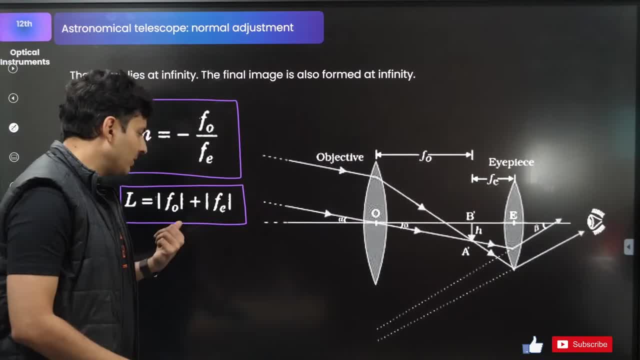 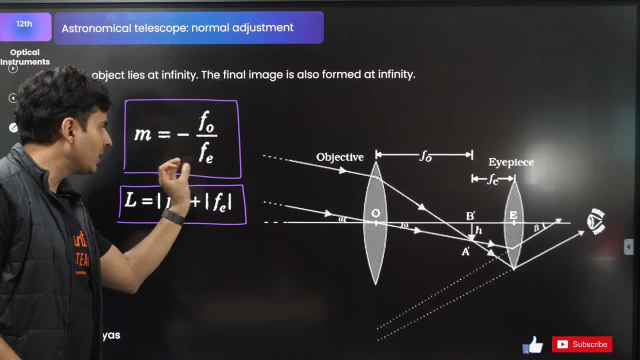 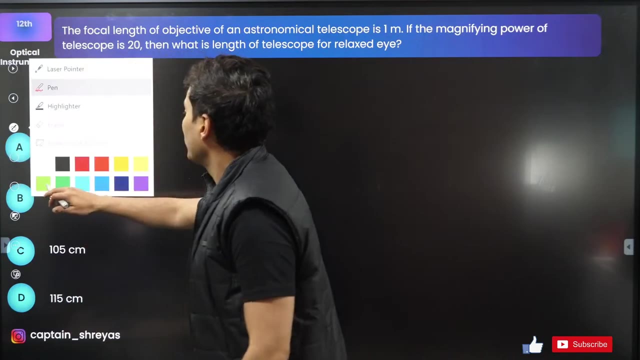 the tube. i just told you it is f0 plus fe, focal length of the objective plus focal length of the eyepiece. as simple as that. object, first eyepiece, later on objective by eyepiece. simple, let's do some questions. let's do some questions. okay, here it comes. what does this question say? the focal? 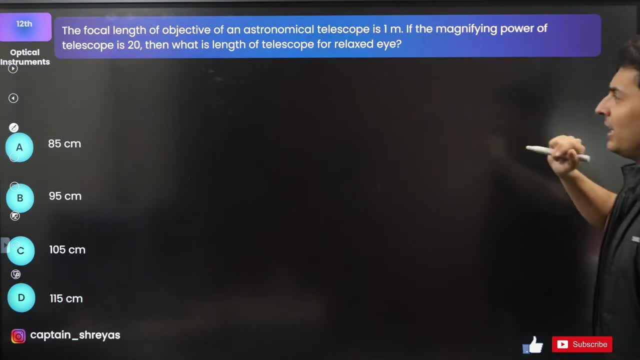 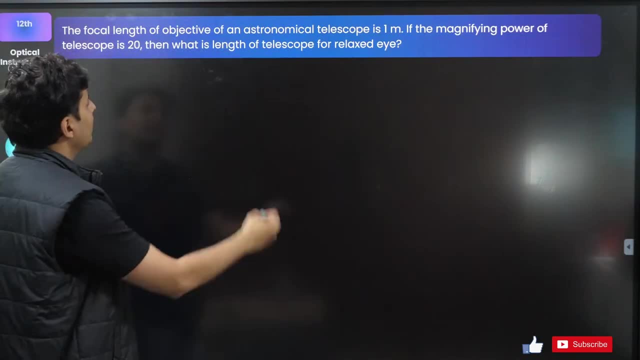 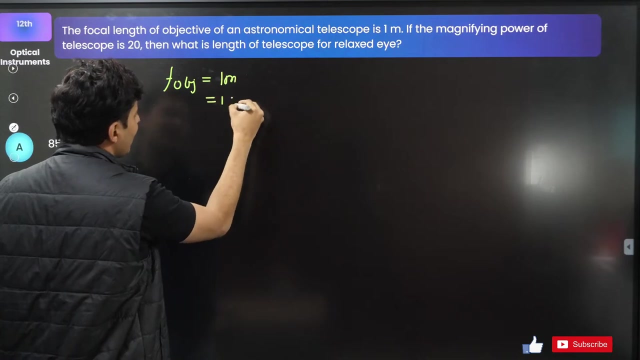 length of the objective is one meter. the magnifying power is 20. what is the length of the telescope? for a relaxed time, everything is in centimeters, so maybe i'll keep all the things also in centimeters. the focal length of the objective is given to be one meter, which is basically 100 centimeters. 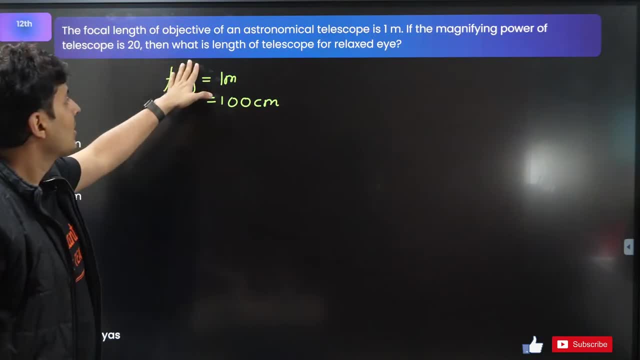 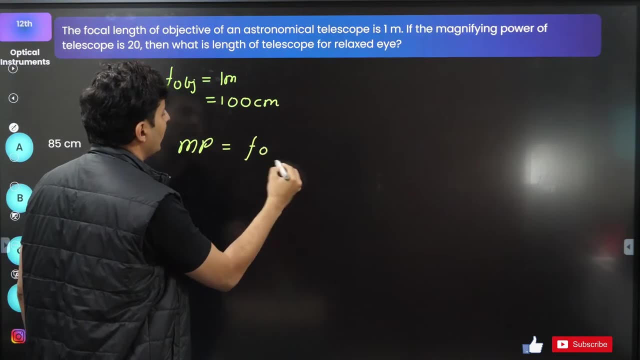 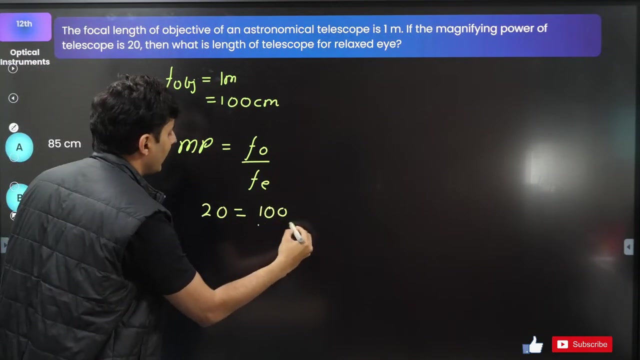 the magnifying power is given for a relaxed time, which is the general case of a telescope. we know the magnifying power of a telescope is focal length of objective by focal length of eyepiece. magnifying power is 20. focal length of objective is 100 divided by fe. so fe will be 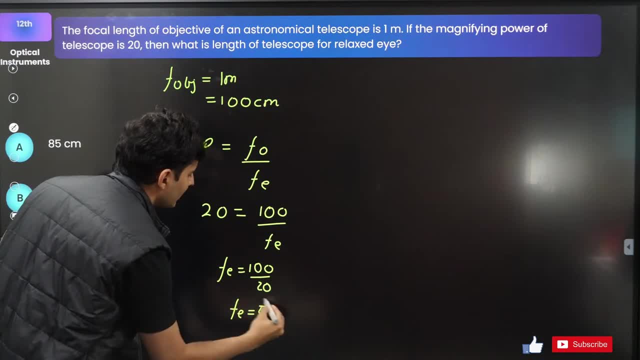 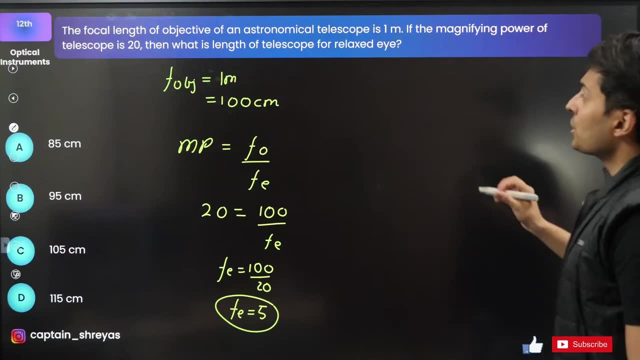 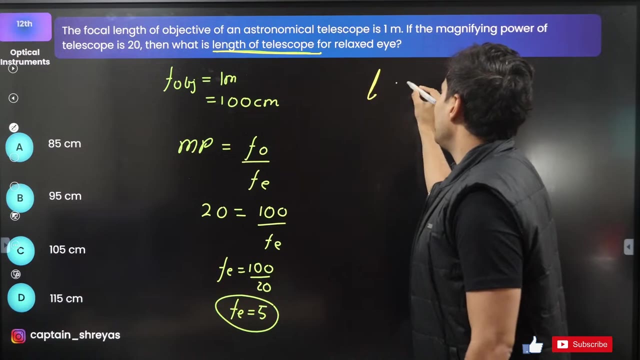 100 by 20. so fe will be just 5, so focal length will be 5 centimeters. great, but the question is not. that question is: what is the length of the telescope? read the question carefully. the question says what is the length of the telescope. the length of the telescope is f0 plus fe. f0 is 100, fe is 5. 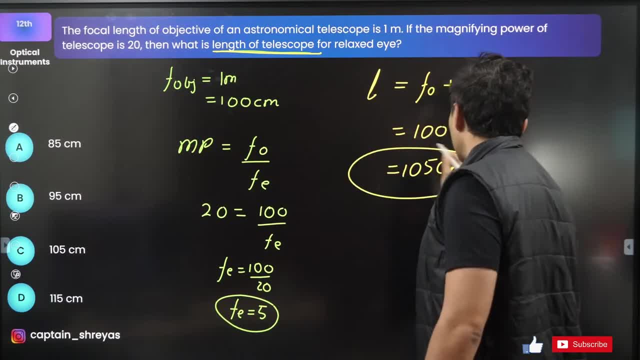 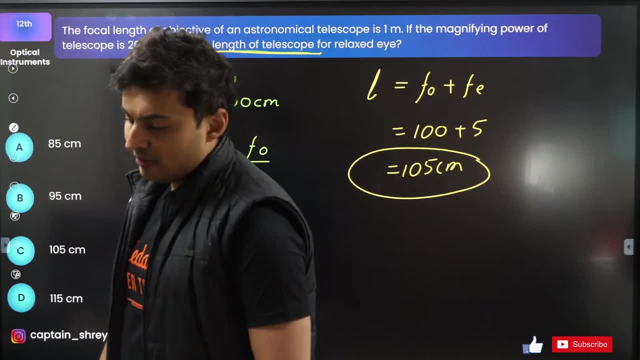 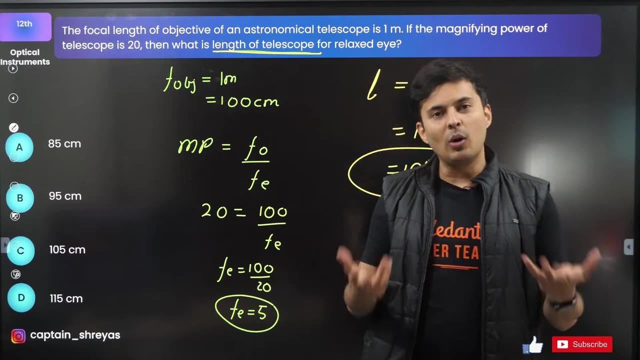 so it should be 105 centimeters. this should be the answer. where is it option c exactly? uh, when we will we then see inverted image? yes, shaku, you'll always see inverted image, be it microscope or be it a telescope. now, because we already know that it is inverted. so one option. 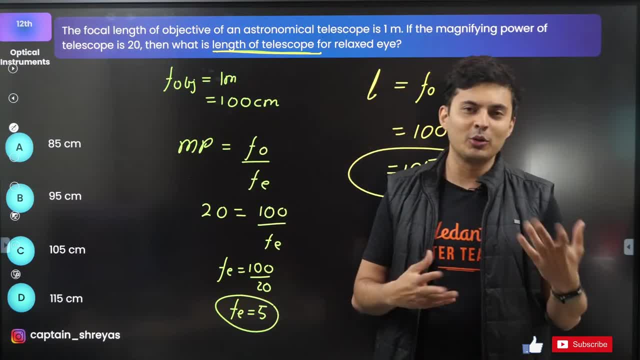 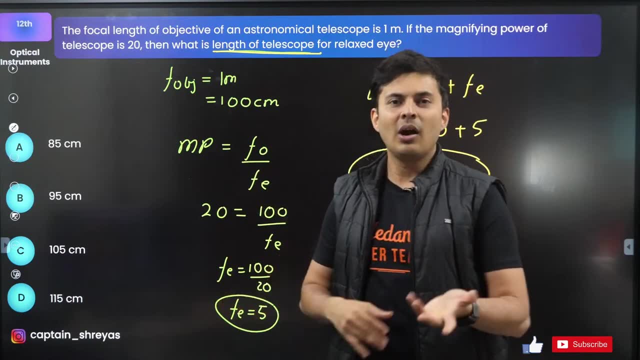 is always: look at it, ulta, you look at it only upside down so you can see the perfect image, or you keep it in mind that whatever you are seeing is opposite and if you, whatever calculations you make accordingly, you make note of that. okay, cool. so moving on to one more question, maybe. 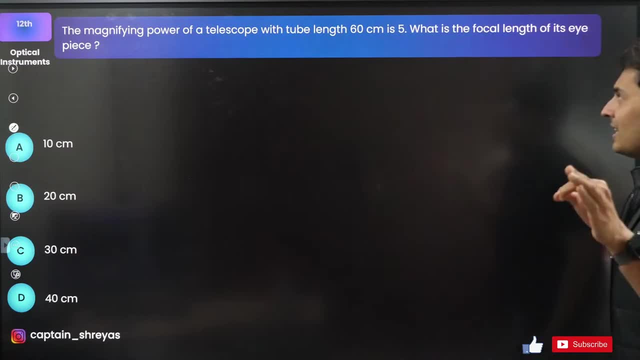 you have two questions right, so we have one question. what is the length of the telescope? yes, the magnifying power of a tube 60 centimeters in length is 5, so a telescope whose tube length is 60 has a power of 5. what is the focal length of the eyepiece? i think it's a complete question. 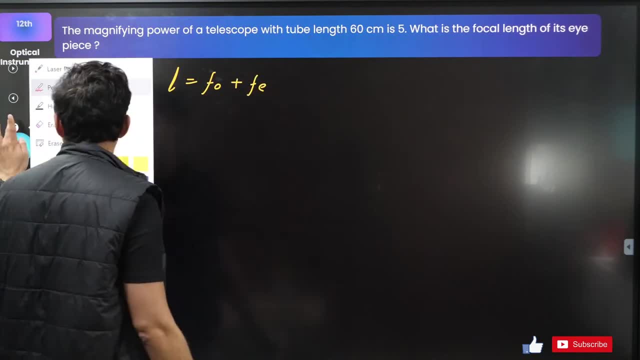 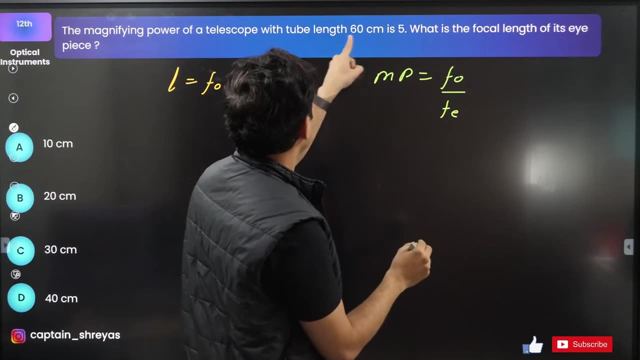 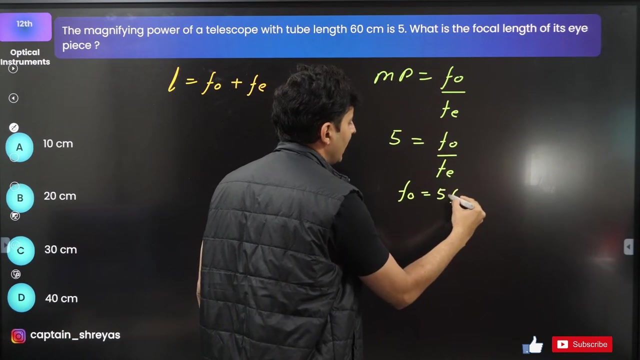 based on formulas. let's stick to the formulas. length of the tube is f0 plus fe. that's one formula. the second formula is magnifying power. magnifying power is f0 by fe. magnifying power is Fe is also not known. So from this, F0 is 5 times of Fe. F0 is 5 times of Fe. So how about putting? 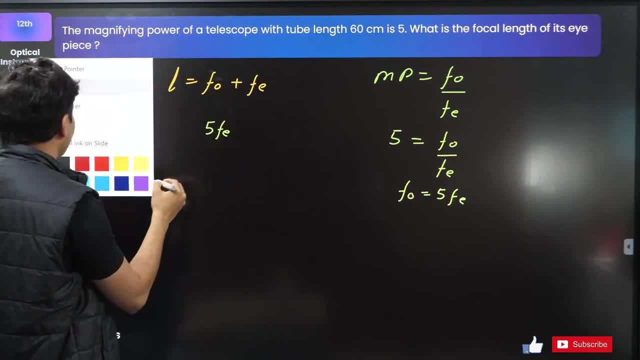 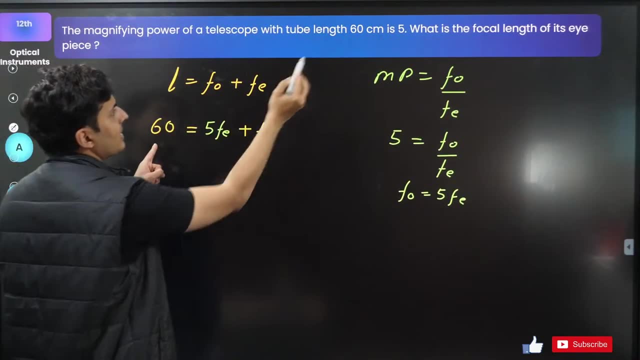 the value of F0 over here. So if I just put 5 times of Fe over here, let's see what do we get. So 5 Fe plus Fe is basically the length, which is 60 centimeters. As per the question, length is 60.. 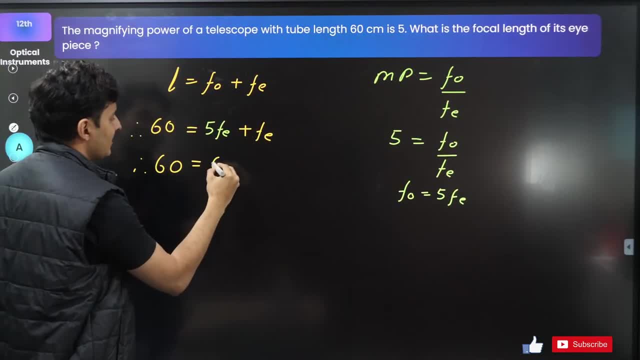 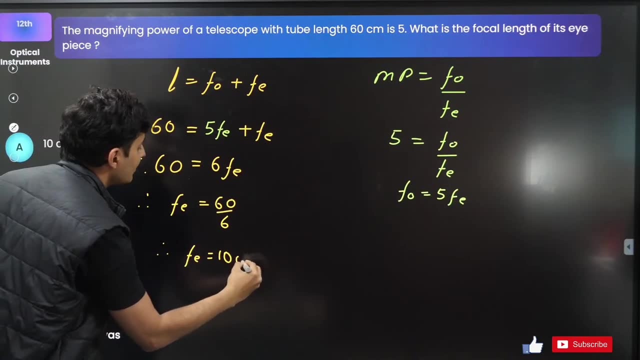 So this 60, therefore, will become 6 times of Fe, So Fe will become 60 by 6.. Therefore, what will Fe be? It will be 10 centimeters. What is asked in the question? Focal length of the eyepiece: Yes, 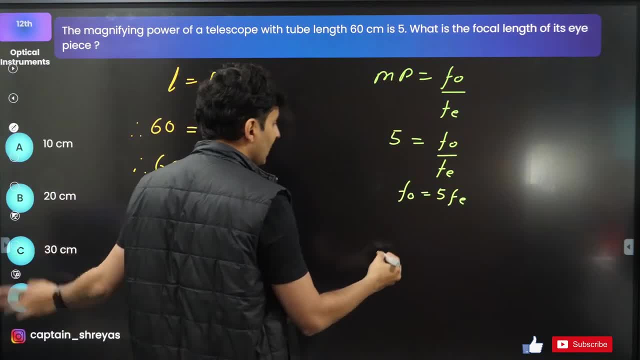 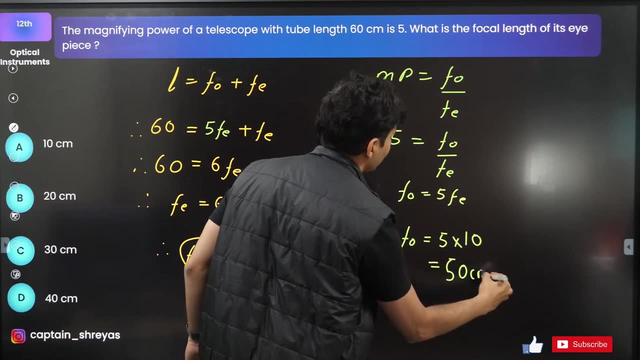 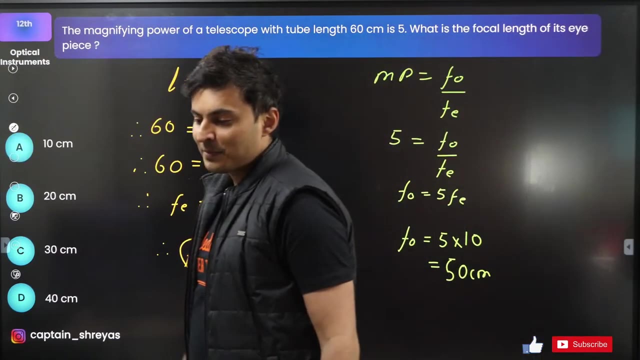 focal length of the eyepiece is 6, sorry, 10 centimeters. If the question said what is the focal length of objective, It will be 5 into 10, which is basically 50 centimeters. But that is not asked, just finding it for you. Hence the answer is 10 centimeters. Everybody clear? Yes, 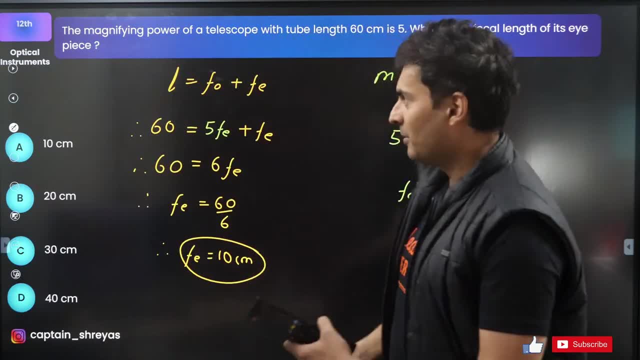 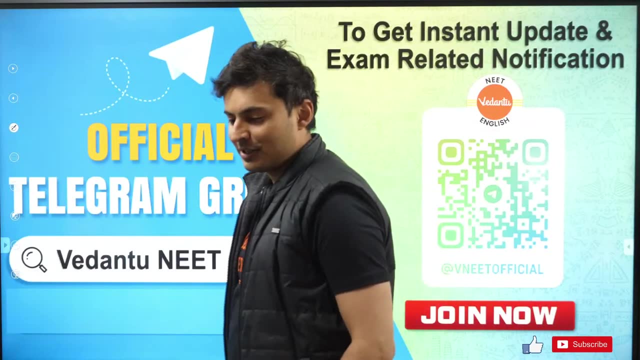 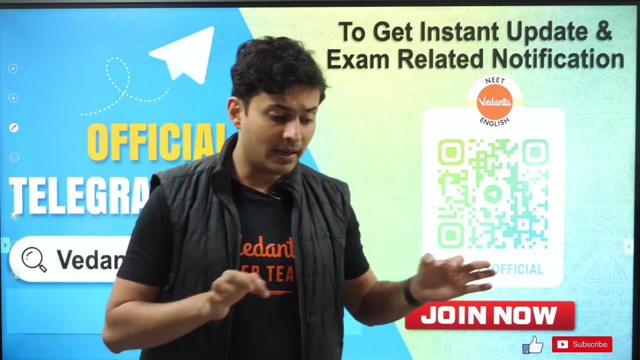 Ashwita. very good, very good, very good. Google logical. you are posting unnecessary doubts over here. I will not be answering. Okay, So now that we have completed optical instruments, what is the next job? You just need to go to telegram channel. Make sure that you join the telegram channel by going to the link. 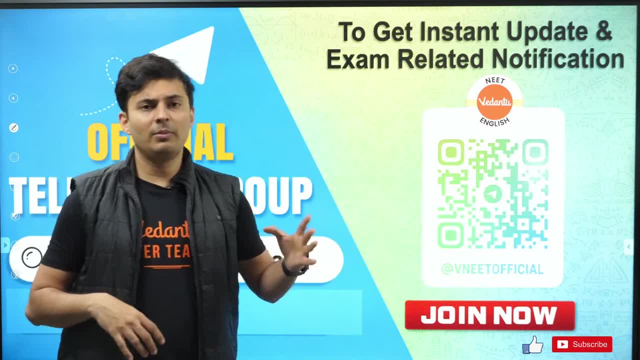 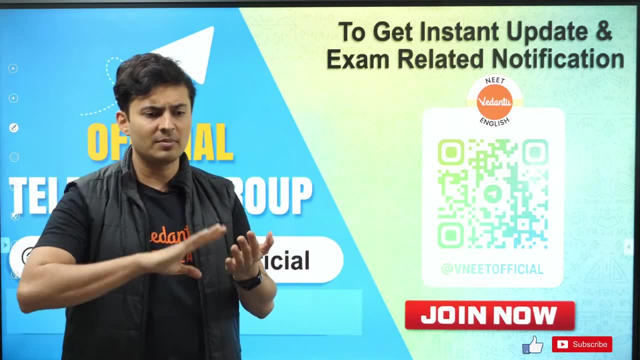 which is there in the description box. I will be posting the PDF. Download the PDF and revise all the problems, all the questions, be it from NCIT, be it your formulas, be it the definitions, be it the ray diagrams, be it your need questions, Keeping in mind that you have formulas concise.